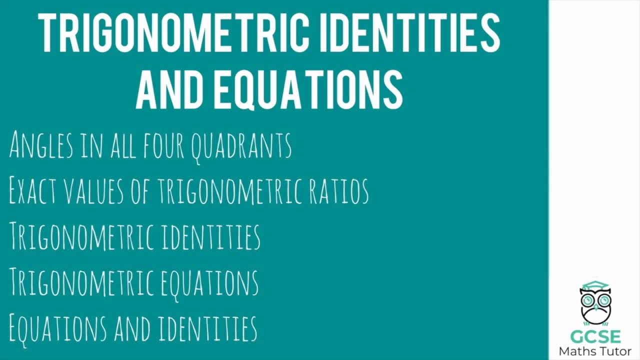 of these videos, I'm just going to quickly show you how these videos work. So let's have a look at that now. So when you are on one of these videos, if you click into the description, 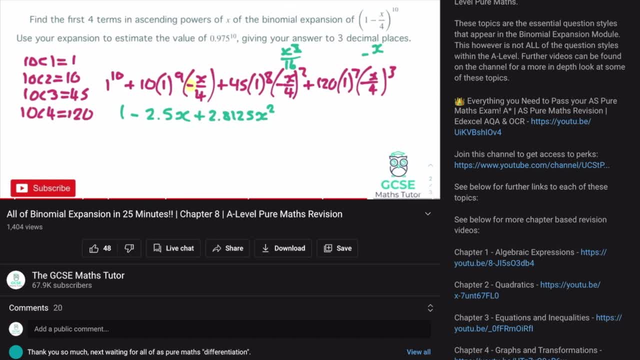 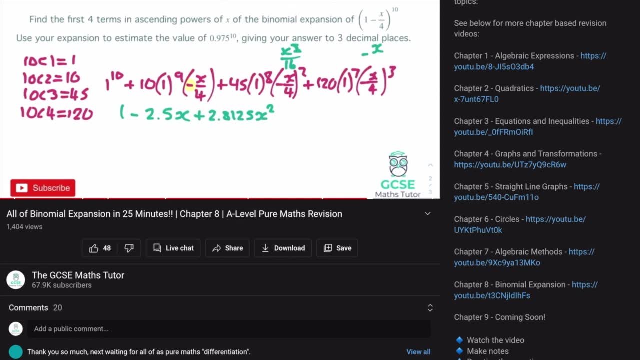 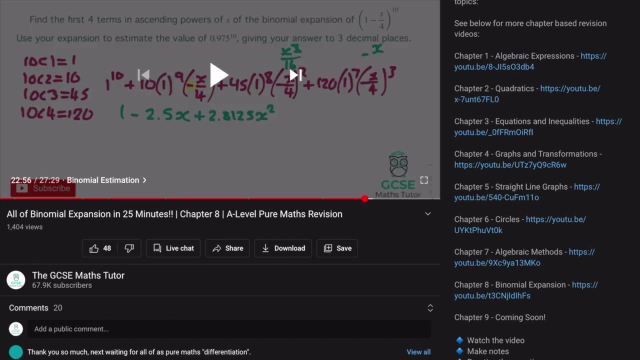 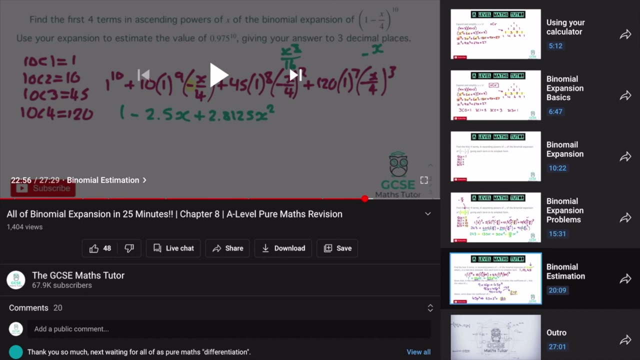 you can see the video there where I cover all of the AS Pure curriculum. And if you scroll down, you can also see all of the chapters. Now these will slowly be filling up until it has filled the entire AS Pure curriculum. So hopefully by the time that you are watching this video, all of them will be actually in the description and you can click and watch each chapter. If you click onto the video and click the link in the bottom left there, you can actually see all of the chapters that are within this video as well. So you can skip through and have a look at the pieces of that chapter that you are needing to have a look at 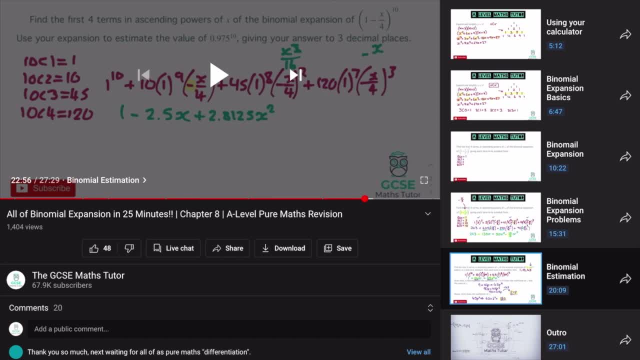 for your revision. So that's how this video works. Hopefully that's useful and helpful. 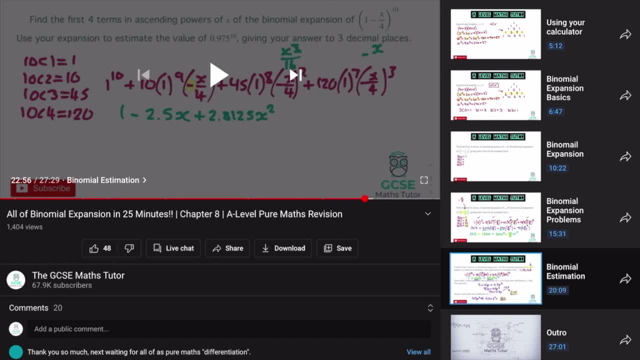 If you enjoy this video, please don't forget to like the video. Don't forget to share it with some of your friends. But with that being said, let's get started. 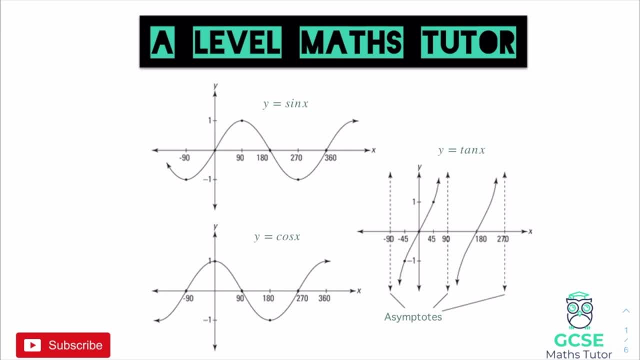 Okay, so when it comes to trigonometric identities and equations, it is essential that you know the trigonometric graphs. So as you can see on the screen, I have three of the trigonometric graphs, and it's very important that you are able to do a sketch of these. These are quite accurate, the ones that I've done on the screen, but you need to be able to draw a sketch of them. So you need to know that for y equals sine x, it goes in the origin, and then we have these waves that go up and over every 90 or up and under every 90. So it goes over the 90, down through the 180, under the 270, and then back through the 360. 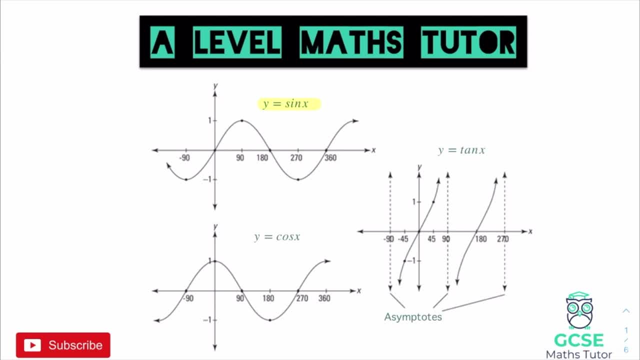 And this graph here goes on infinitely to the left and right of the y-axis, but we need to know how to draw a sketch of that, and you're going to see why in some later questions. 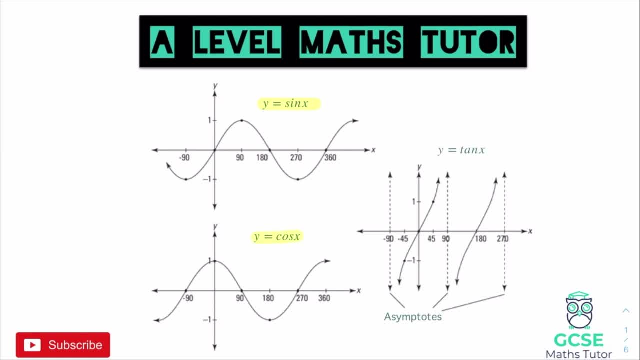 For the one below, for the cos graph, this has just been translated, or it's the sine graph, which has been translated 90 degrees to the left. So you can see instead it starts at 1 on the y-axis, but then it follows a very similar pattern. It goes down through 90, under 180, up through 270, and up and over 360. 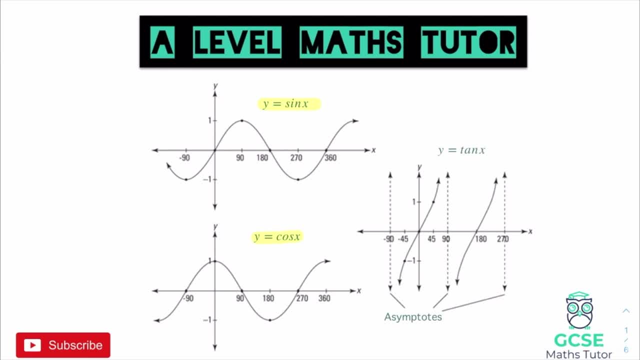 And again, this goes on infinitely to the left and right of the y-axis, but it follows this pattern. 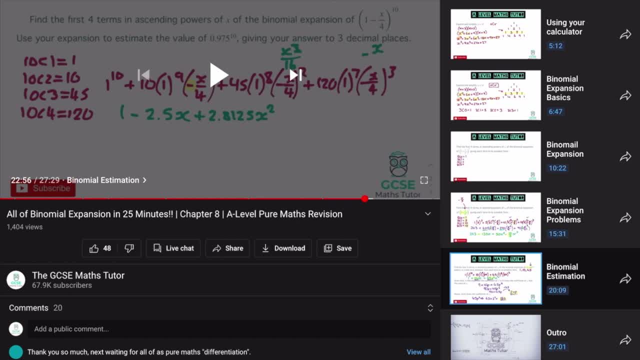 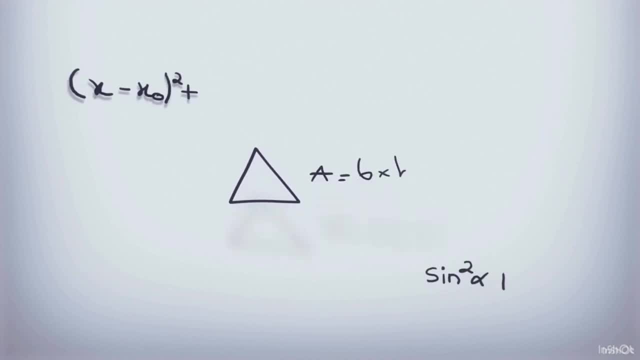 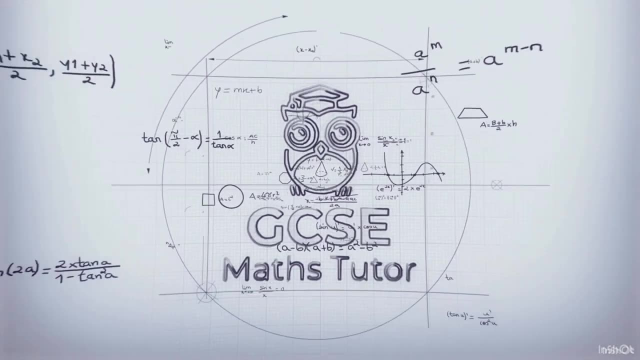 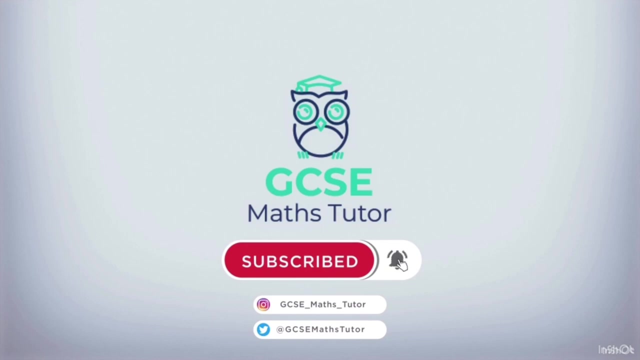 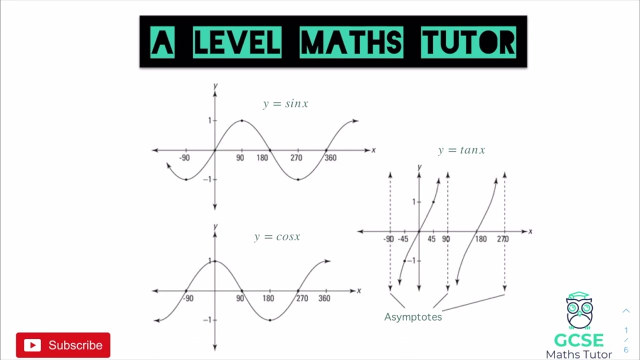 If you enjoy this video, please don't forget to like the video. Don't forget to share it with some of your friends. But with that being said, let's get started. Okay, so when it comes to trigonometric identities and equations, it is essential that you know the 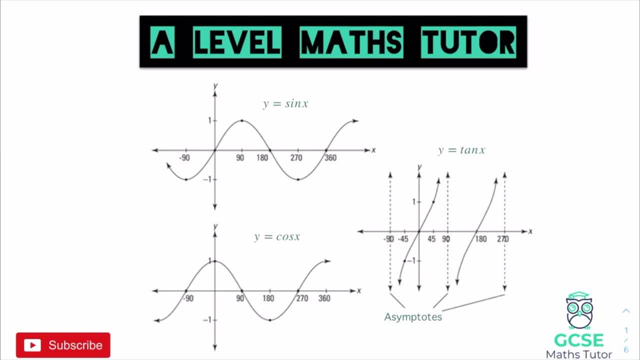 trigonometric graphs. So, as you can see on the screen, I have three of the trigonometric graphs and it's very important that you are able to do a sketch of these. These are quite accurate, the ones that I've done on the screen, but you need to be able to draw a sketch of them. 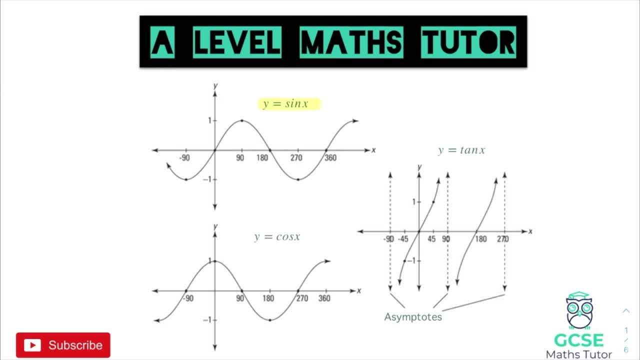 So you need to know that, for y equals sine x, it goes in the origin, and then we have these waves that go up and over every 90 or up and under every 90. So it goes over the 90, down through the 180,. 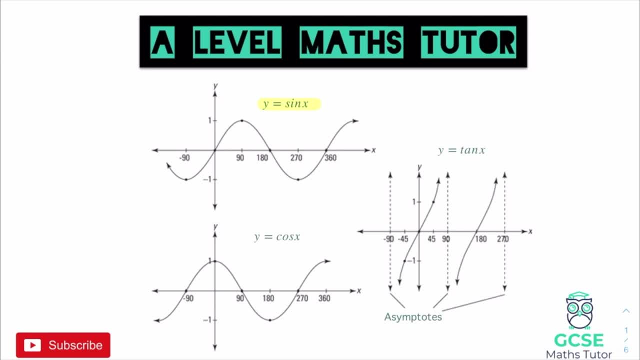 under the 270, and then back through the 360. And this graph here goes on infinitely to the left and right of the y-axis. but we need to know how to draw a sketch of that, and you're going to see why in some later questions. 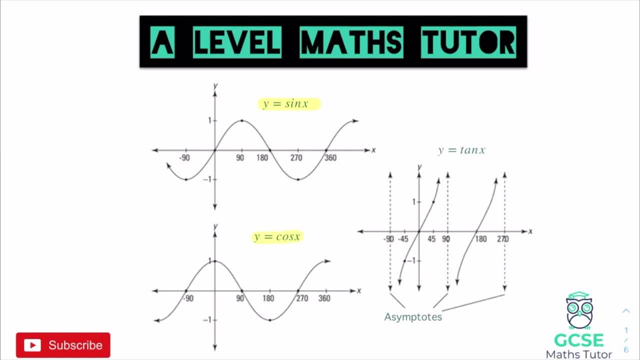 For the one below, for the cos graph, this has just been translated, or it's the sine graph which has been translated: 90 degrees to the left, So you can see. instead it starts at 1 on the y-axis, but then it follows a very similar pattern. It goes down through 90, under 180, up through 270,. 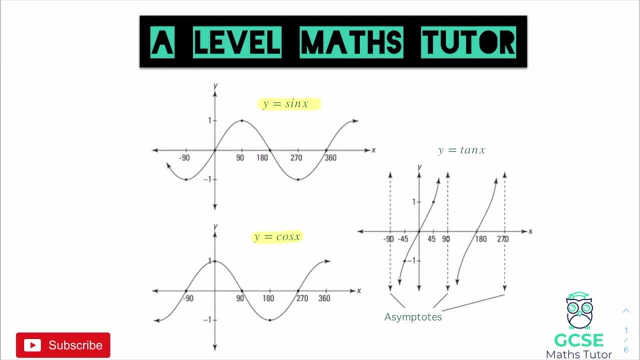 and up and over 360.. And again, this goes on infinitely to the left and right of the y-axis, but it follows this pattern. The tan graph is very different. It does have these waves and, as you can see, there are asymptotes. 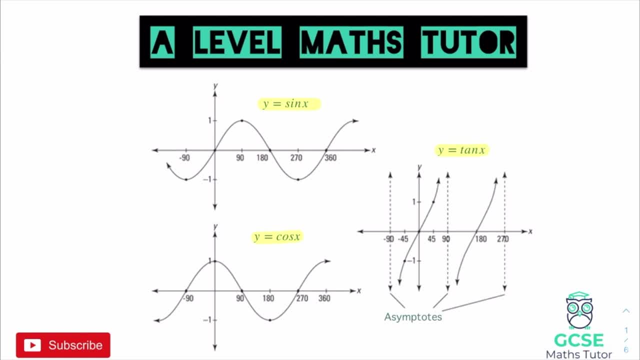 at minus 90 and 90, and then each asymptote follows on every 180 degrees and again, that is to the right and to the left of these curves. So you do need to know these graphs, You need to be able to draw basic sketches of them, and this is going to be very helpful when 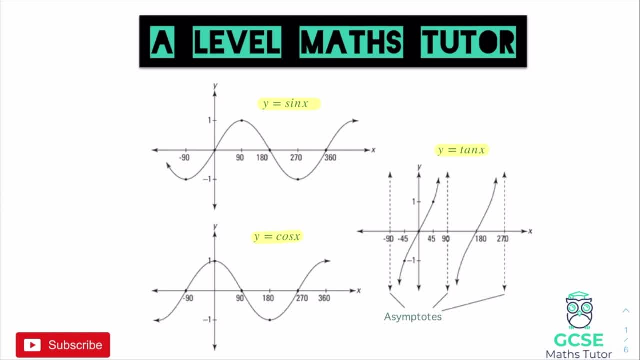 we are solving our trigonometric equations as I do. Again, there are other ways of solving trigonometric equations, but I do use this graphical method as I do like them, and I do think that it's important that you know these. 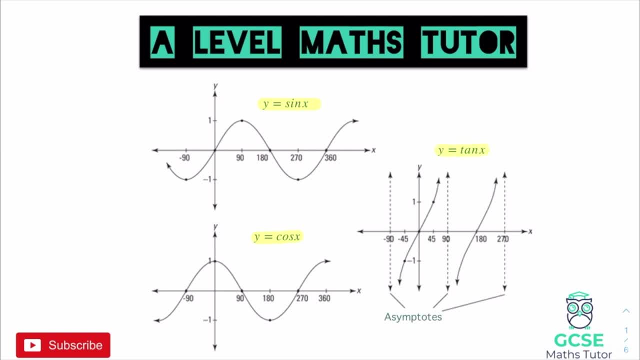 The tan graph is very different. It does have these waves, and as you can see, there are asymptotes at minus 90 and 90, and then each asymptote follows on every 180 degrees, and again, that is to the right and to the left of these curves. So you do need to know these graphs. 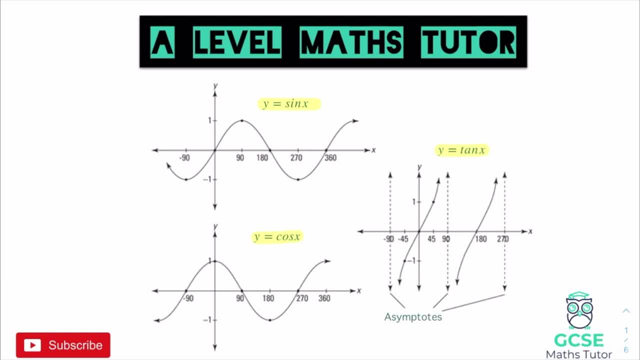 You need to be able to draw basic sketches of them, and this is going to be very helpful when we are solving our trigonometric equations, as I do. Again, there are other ways of solving trigonometric equations, but I do use this graphical method as I do like them, and I do think that it's important that you know these anyway, so it's always good to be able to use them for further elements. 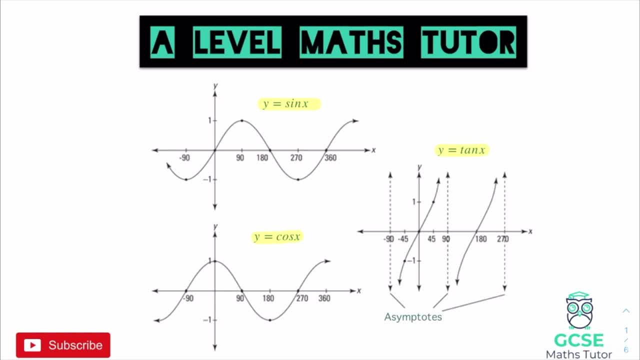 So do make sure that you can draw a basic sketch of all of these graphs, and you know that they're very well. 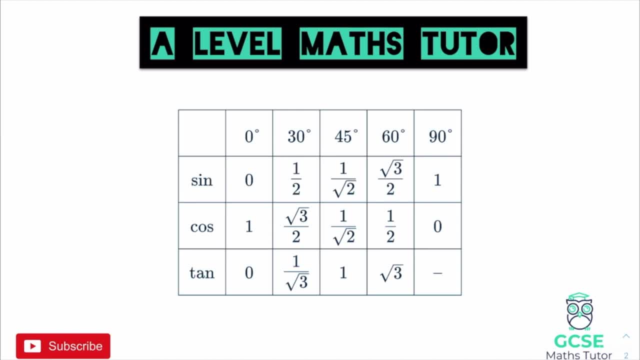 Okay, so within this is also some exact trig values. Now, you should know a lot of these exact trig values from GCSE level, but these are just the basic trig values, or the exact trig values. 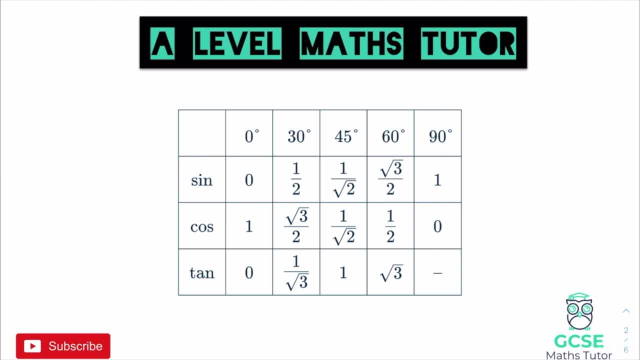 Now, some of these can be written slightly differently. For example, 1 over root 3 down here for tan 30, you could actually rationalize that, multiplying top and bottom by root 3, and instead you could write it as root 3. 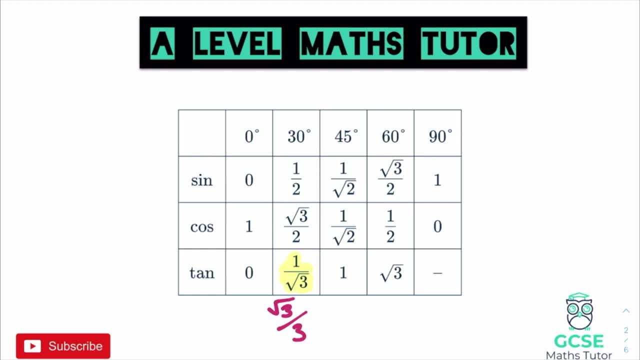 That's absolutely fine, and of course you will have a calculator for all these questions, but there are some exact trig values that you should know, and also you should be able to then relate these to the trigonometric graphs, and we will see on some later questions when we are looking at solving them. So for now, all you need to do is you need to make sure you know these exact trig values, and you also need to know the method for finding them. Again, I'll link the video in the description, for how to find these, so if you're not sure on how to find them, or how to learn these, then obviously you can go and you can check the full video in the description. 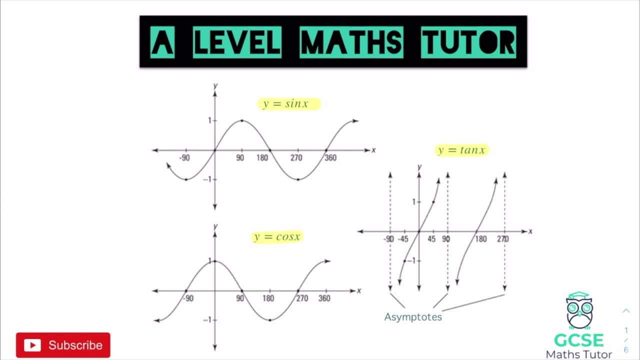 anyway, so it's always good to be able to use them for further elements. So do make sure that you can draw a basic sketch of all of these graphs and you know that you're going to be able to use them for further elements. 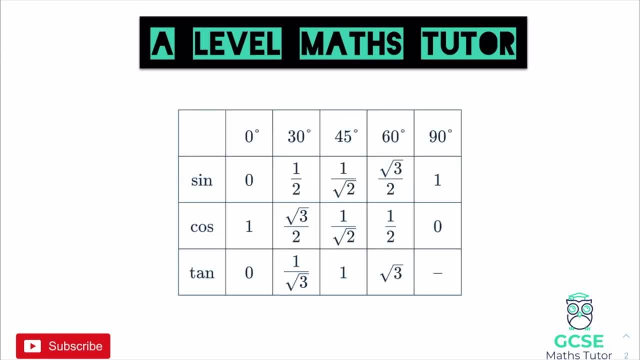 So do make sure that you can draw a basic sketch of all of these graphs, and you know that you're very well. Okay, so within this is also some exact trig values. Now, you should know a lot of these exact trig values from GCSE level, but these are just the basic trig values or the exact trig. 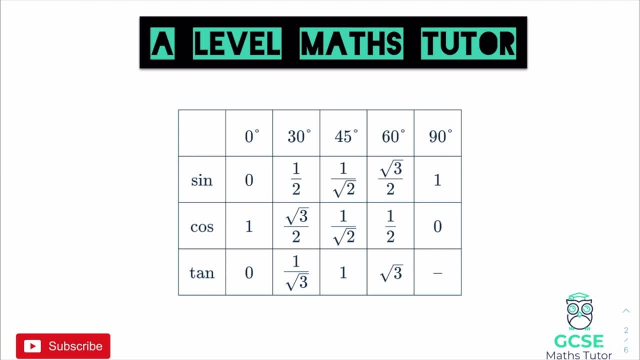 values. Now some of these can be written slightly differently. For example, 1 over root 3 down here for tan 30, you could actually rationalise that multiplying top and bottom by root 3, and instead you could write it as root 3.. So you could actually rationalise that multiplying top and bottom by 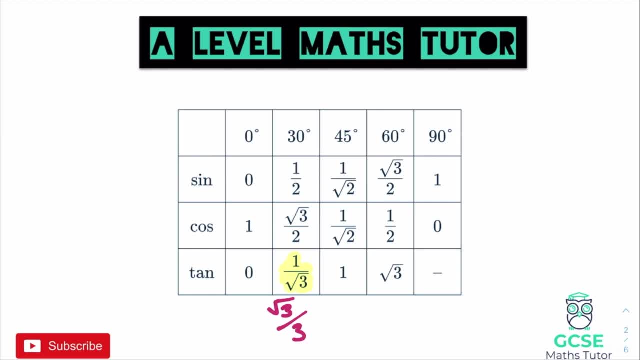 root 3 over 3.. That's absolutely fine and of course you will have a calculator for all these questions, but there are some exact trig values that you should know and also you should be able to then relate these to the trigonometric graphs. and we will see on some later questions when we 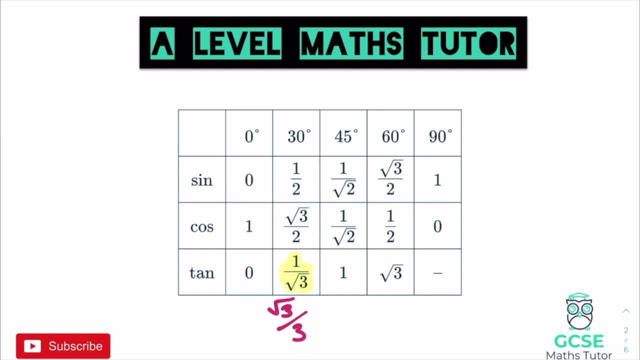 are looking at solving them. So for now, all you need to do is you need to make sure you know these exact trig values, and you also need to know the method for finding them. Again, I'll link the video in the description for you to see how you can do that, and I'll also link the video in the 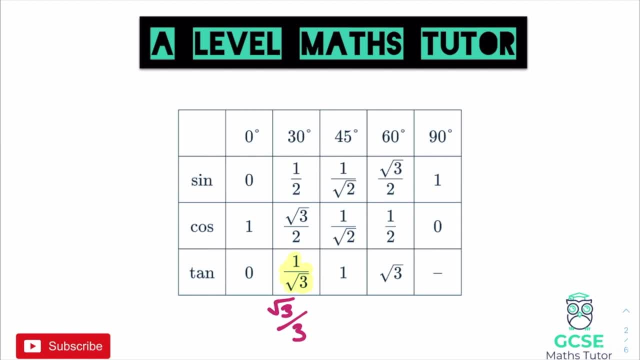 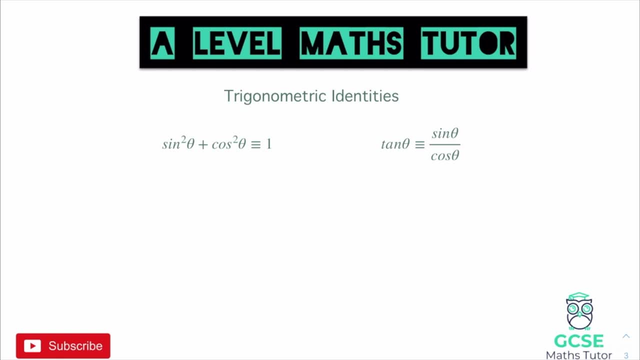 description for how to find these. so if you're not sure on how to find them or how to learn these, then obviously you can go and you can check the full video in the description. Okay, so the two main trigonometric identities that we need to know are these two, So we'll start with. 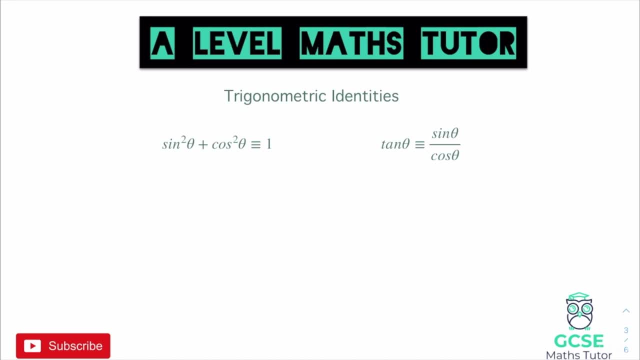 the one on the left. We've got sine squared theta plus cos squared theta is always equal or identical to 1.. Now, this one is super important, as is the other one, but this one is very important. Now, this can also be rearranged. So if you want to know how to find these, you need to know the method for finding. 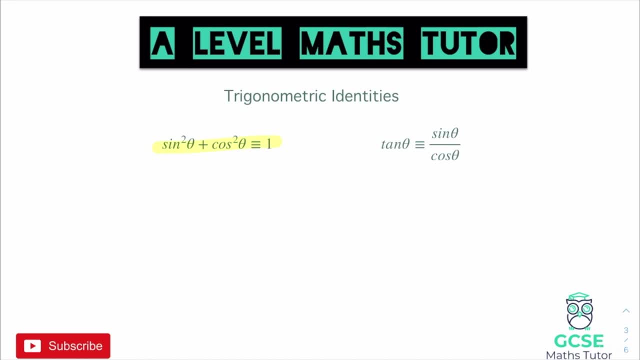 these. So we'll do minus cos squared theta to the other side. So if we look at the image we've just hayaed, it is the same as the rough image. So this one is EX colleges and we can multiply it with the theorem and multiply it. That way we can hear exactly what we have to do. We can also say that: 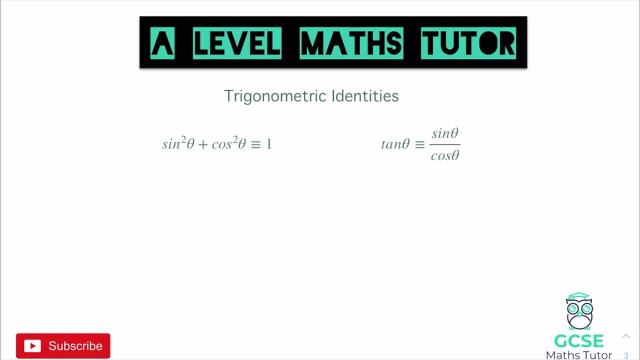 Okay, so the two main trigonometric identities that we need to know are these two. So we'll start with the one on the left. We've got sine squared theta plus cos squared theta is always equal or identical to 1. Now, this one is super important, as is the other one, but this one is very important. Now, this can also be rearranged. We've got the trigonometric equation. We've got sine squared theta plus cos squared theta is always equal or identical to 1 minus cos squared theta. So that is another one of our identities. Of course, we could have also rearranged it by minusing sine squared theta to the other side, which would have left us with cos squared theta, which is identical to 1 minus sine squared theta. So you need to know that identity. 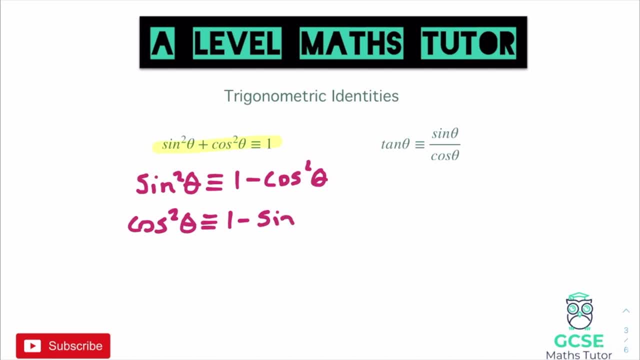 So we've got the trigonometric equation. We've got the trigonometric equation. We've got the trigonometric equation. 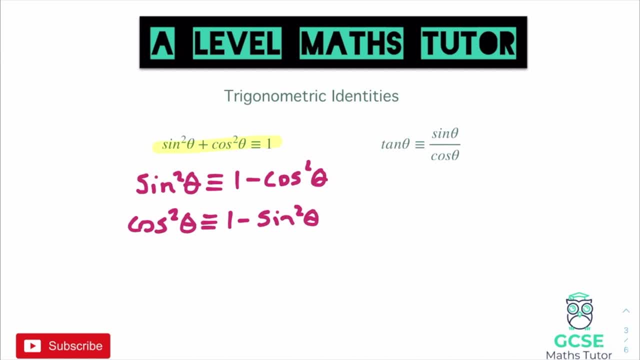 We've got the identity. And you need to also know these two rearrangements, as we'll be using these a lot throughout our trigonometric identities. For the one on the right, when we're looking at tan theta is equal to sine theta over cos theta, we can also do rearrangements of that. So if we multiply cos theta to the other side, we could also say that tan theta multiplied by cos theta, so tan theta cos theta, is equal to sine theta. And again, we could rearrange that by dividing both sides by tan theta. And we could say that cos theta is equal to sine theta over tan theta. 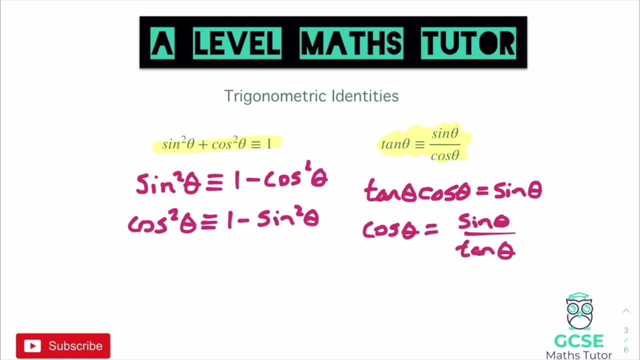 So there are rearrangements of this as well that you need to know, but as long as you know the two at the top that I've highlighted, you should be perfectly comfortable rearranging them. And of course, that leaves us with quite a few identities here. So really, you only have to learn the main two and then obviously how to rearrange them. But these arrangements, are very important, I'd make sure that you had these written down on some exam revision flash cards so that you always had these to hand. As we're going to be using these for any trigonometric 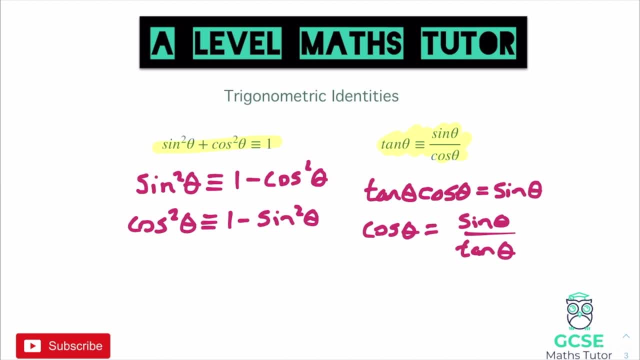 identity, we'll be using one or the other, and particularly with our trigonometric equations, 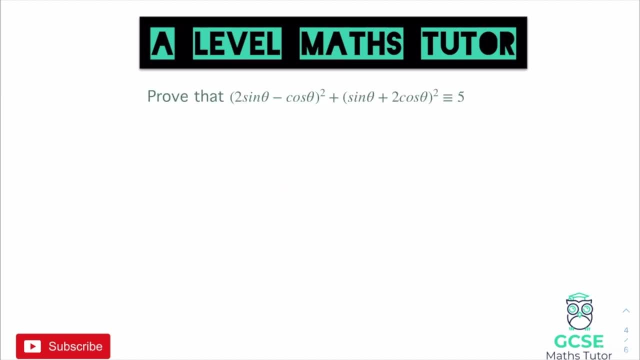 so do make sure you know these very well. Okay, so looking at a trigonometric identity. Now as you can see here, it says prove that 2 sine theta minus cos theta squared plus sine theta 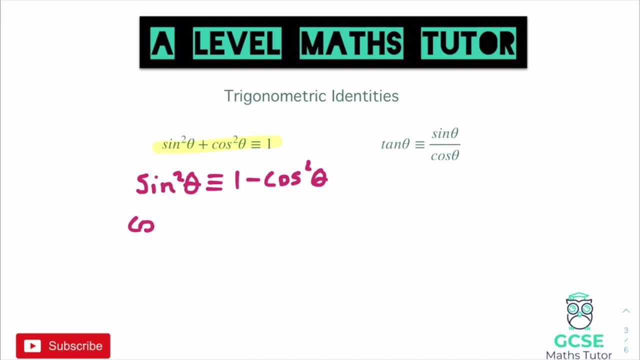 sine squared theta is 1.. If we multiply it by the derivativeoi, we get the siguiente has the same homogenous line as that. So if we think out the original equation, why don't we do the reverse? know that identity and you need to also know these two rearrangements, as we'll be using. 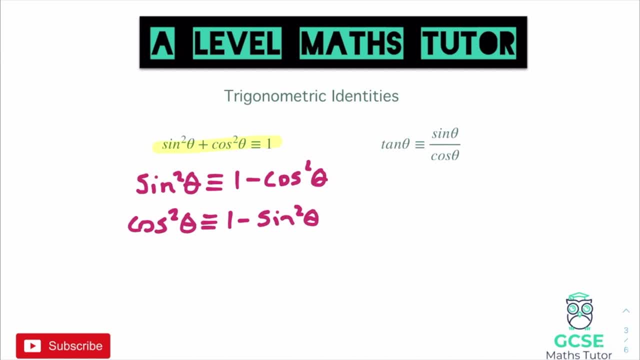 these a lot throughout our trigonometric identities. For the one on the right, when we're looking at tan theta is equal to sine theta over cos theta. we can also do rearrangements of that. So if we multiply cos theta to the other side we could also say that tan theta multiplied. 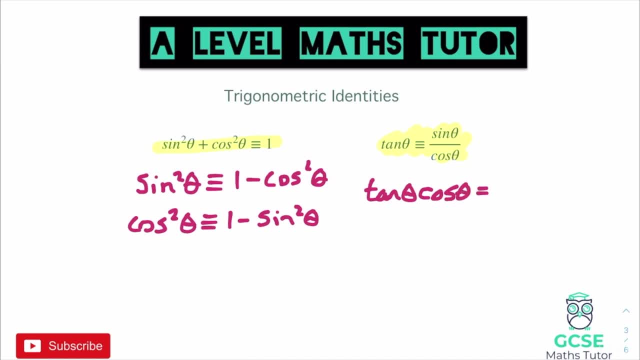 by cos theta, so tan theta, cos theta is equal to sine theta. And again, we could rearrange that by dividing both sides by tan theta and we could say that cos theta is equal to sine theta over tan theta. So there are rearrangements of this as well that you need to know. but 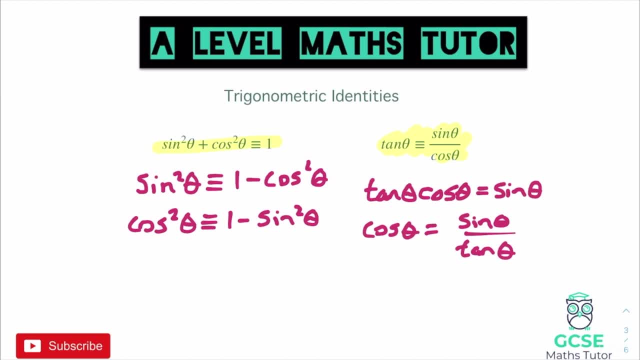 as long as you know the two at the top that I've highlighted, you should be perfectly comfortable rearranging them, and of course that leaves us with quite a bit of time. Let's look at a few identities here. So really, you only have to learn the main two and then. 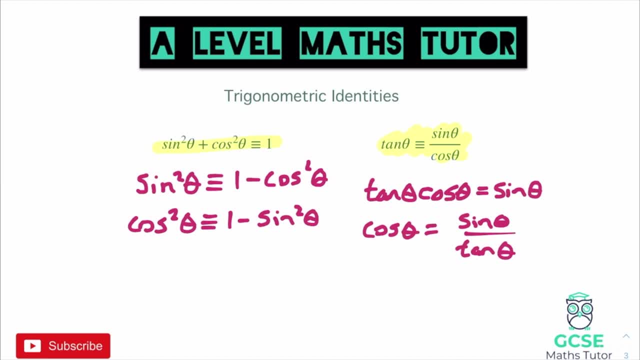 obviously how to rearrange them, But these are very important. I'd make sure that you have these written down on some exam revision flashcards so that you always have these to hand, As we're going to be using these for any trigonometric identity we'll be using. 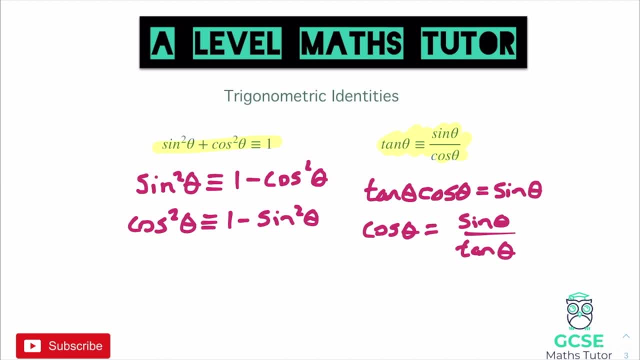 one or the other, and particularly with our trigonometric equations. so do make sure you know these very well. Okay, so, looking at a trigonometric identity Now, as you can see, we've got a trigonometric identity and we've got a trigonometric identity. 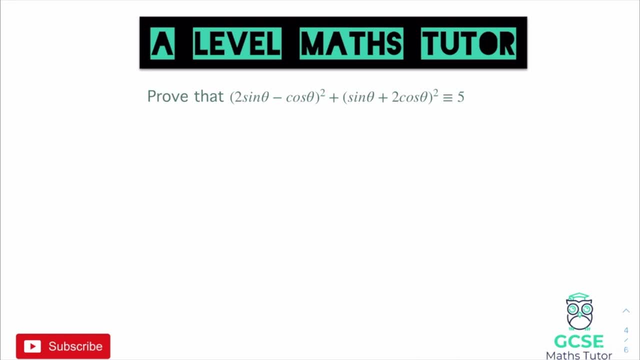 and you can see here it says: prove that 2 sine theta minus cos theta squared, plus sine theta plus 2 cos theta squared is identical to 5, or always equal to 5.. Now this is just one example of lots of different types of questions, So of course you do need to practice. 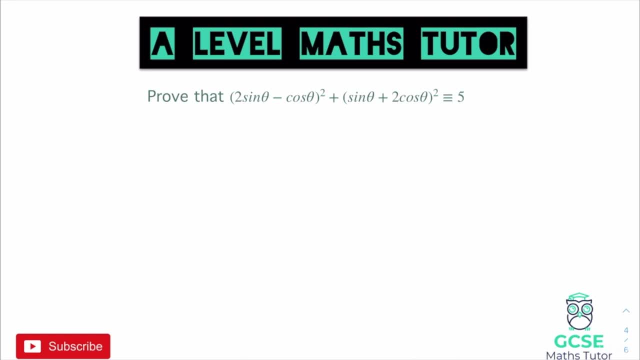 quite a lot of these, but this is a really good one for us to have a look at. So what we need to show in this is that all of this on this left-hand side is going to be equal to 5, or is going to always equal 5.. 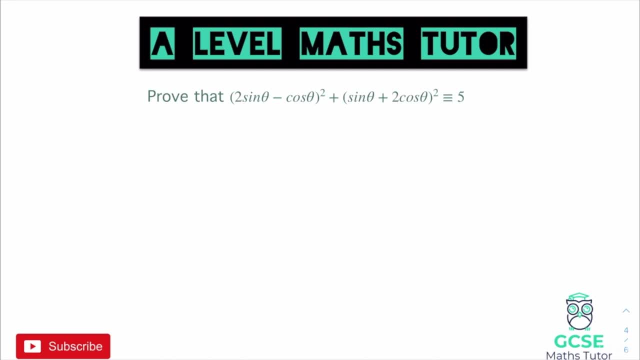 plus 2 cos theta squared is identical to 5, or always equal to 5. Now this is just one example of lots of different types of questions. So of course you do need to practice quite a lot of these, but this is a really good one for us to have a look at. So what we need to show in this 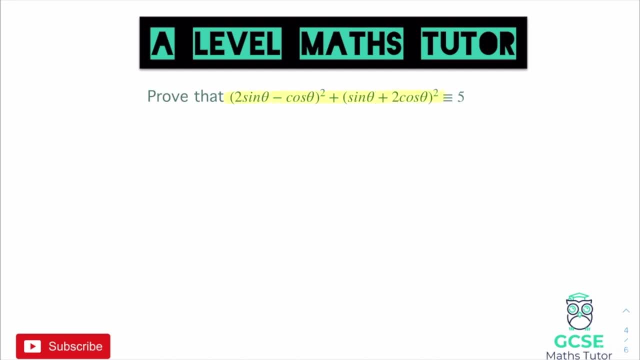 is that all of this on this left-hand side is going to be equal to 5, or is going to always equal 5. And we can go about that by using some of our trig identities. Now we don't have a tan theta in this one, but that's not necessarily the case. So we're going to go about that by using 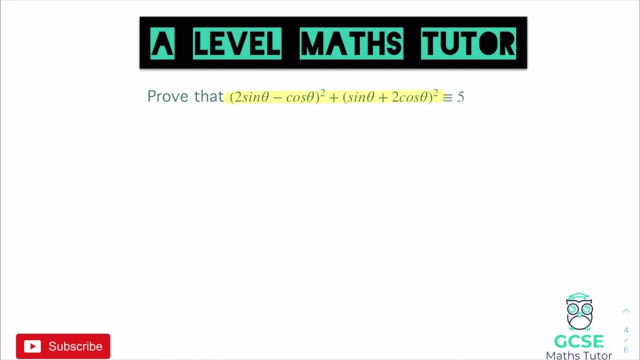 our trig identity. So if we're looking at this one, we want to think about how we could change this so that it just becomes one or the other. But maybe we'll have a look at expanding it first and seeing what we get. So if we expand the first one here, that's going to be a double bracket, and that would be 2 sine theta minus cos theta, and we'll go about expanding it. So we would write that twice. So 2 sine theta minus cos theta, and you can already see that we're going to get some squares involved. So if we expand that, 2 sine theta times 2 sine sine theta would become 4 sine squared theta, and then 2 sine theta times the minus cos theta, and we're going to do that twice. So that would be minus 4, and you could write either sine or cos first here, but 4 sine theta. 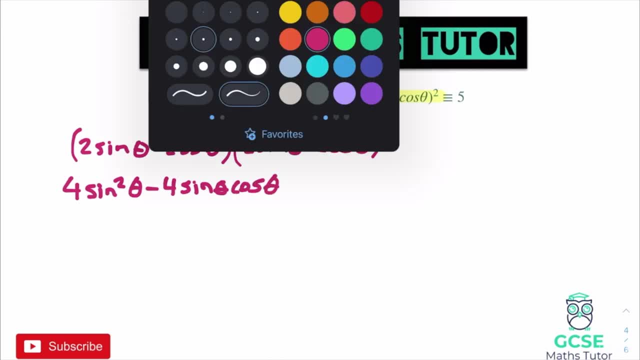 Again, that piece that I've done just there, I have skipped a step in my expansion. I did 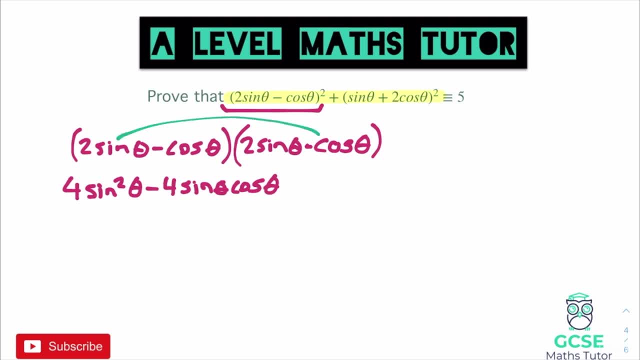 2 sine theta times the minus cos theta, and the minus cos theta times the 2 sine theta. 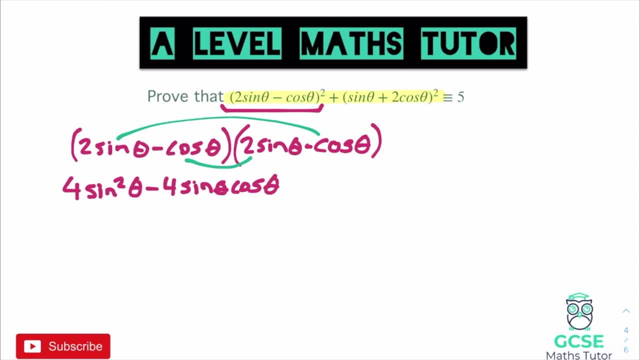 So I just doubled that up in one step. We now have to do the negative cos theta times the negative cos theta, which gives us plus plus cos squared theta. Now we can move on to our second bracket. Now we've fully expanded that one, and our second bracket is this one here. 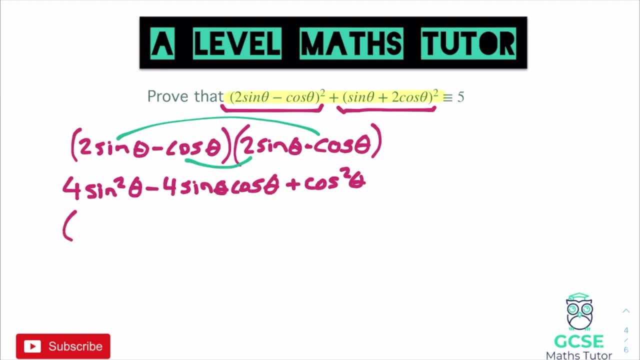 So if we expand that as well, that is, again, two of those brackets. So sine theta plus 2 cos theta, and we're going to multiply that by another sine theta plus 2 cos theta. 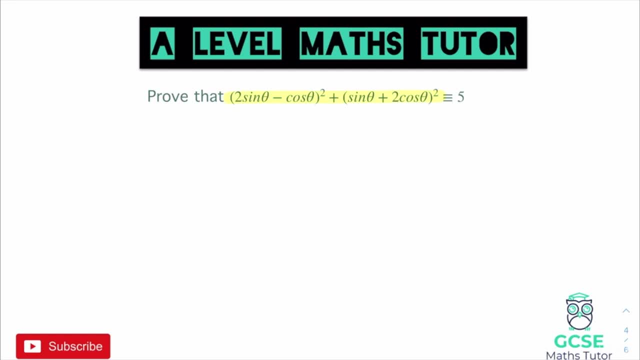 And we can go about that by using some of our trig identities. Now, we don't have a tan theta in this one, but that's not necessarily to say that it won't appear. but obviously we do have our other trig identity that has sin, sine and cos in. So if we're looking 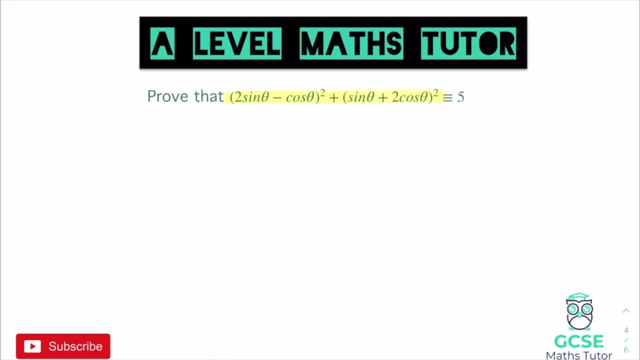 at this one. we want to think about how we could change this so that it just becomes one or the other, But maybe we'll have a look at expanding it first and seeing what we get. So if we expand the first one here, that's going to be a double bracket and that would 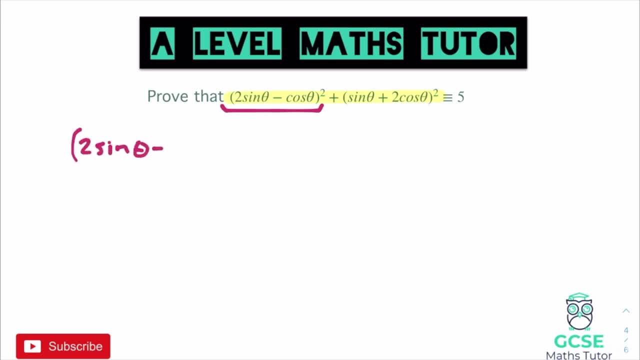 be 2 sin theta minus cos theta and we'll go about expanding that So we would write that twice. So 2 sin theta minus cos theta and you can already see that we're going to get some squares involved. So if we expand that, 2 sin theta times 2 sin theta would 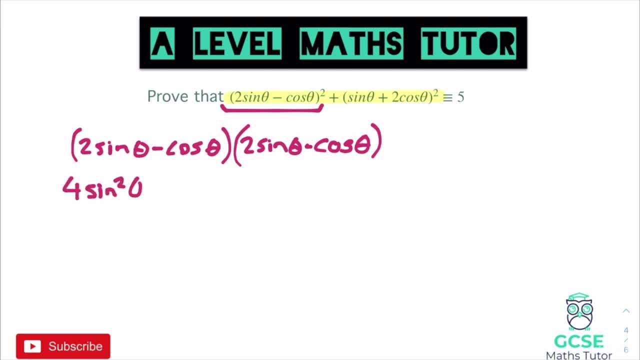 become 4 sin squared theta and then 2 sin theta times the minus cos theta, and we're going to do that twice. So that would be minus 4, and you could write either sin or cos first here, but 4 sin theta. 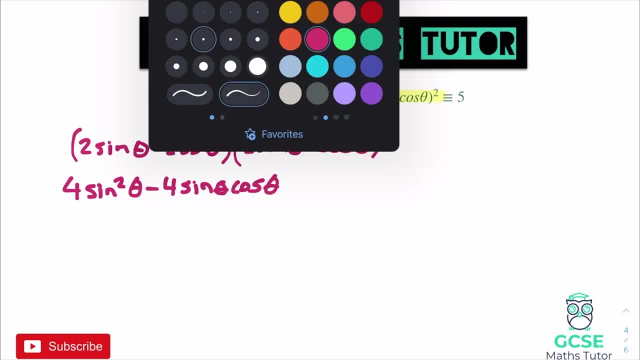 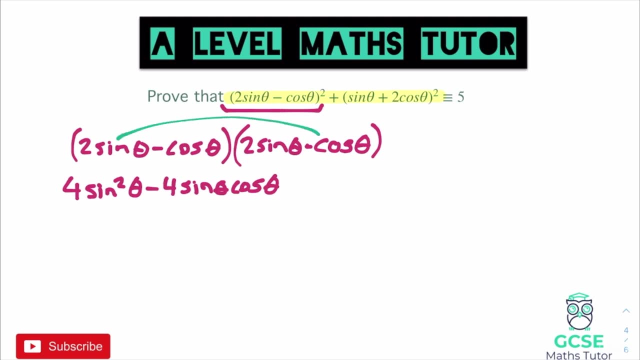 cos theta- Again that piece that I've done. just there I have skipped a step in my expansion. I did 2 sin theta times the minus cos theta and the minus cos theta times the 2 sin theta. So I just doubled that up in one step. We now have to do the negative cos theta times. 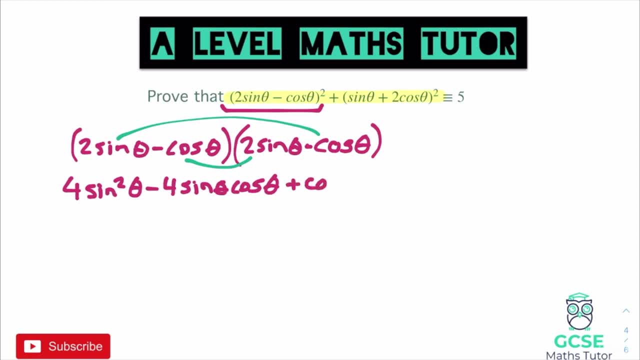 the negative: cos theta which gives us plus, cos squared theta. Now we can move on to our second bracket. Now we've fully expanded that one and our second bracket is this one here. So if we expand that as well, that is again two of. 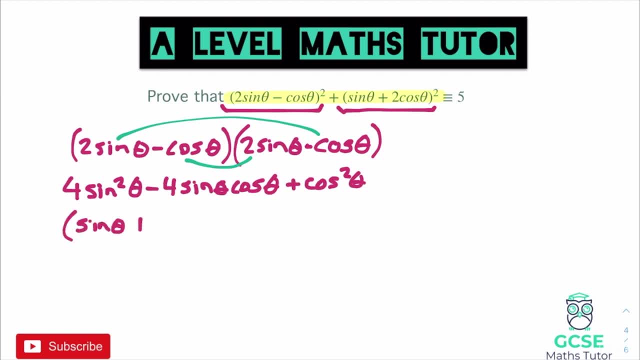 those brackets. So sin theta plus 2 cos theta, and we're going to multiply that by another sin theta plus 2 cos theta. Okay, so if we expand, this one sin theta times sin theta gives us sin squared theta. Then we've got sin theta times the 2 cos theta and we've got that twice. So again that's. 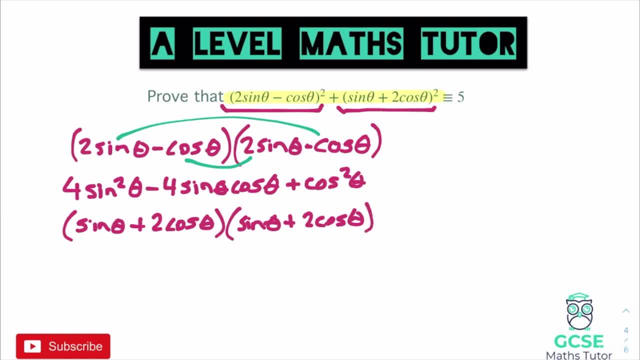 OK, so if we expand this one, sine theta times sine theta gives us sine squared theta. Then we've got sine theta times the 2 cos theta, and we've got that twice. So again, that's going to be plus 4 sine theta cos theta. There we go. And then we have the 2 cos theta times the 2 cos theta, which gives us plus 4 cos squared theta. So we've got our two pieces, and we need to add them together after we had a plus sign between these two. So if we add those two pieces together, and let's see what we get. So we've got the 4 sine squared theta, and a 1 sine squared theta. So we've got the 4 sine squared theta, and a 1 sine squared theta here. So that would be equal to 5 sine squared theta. We've then got these middle 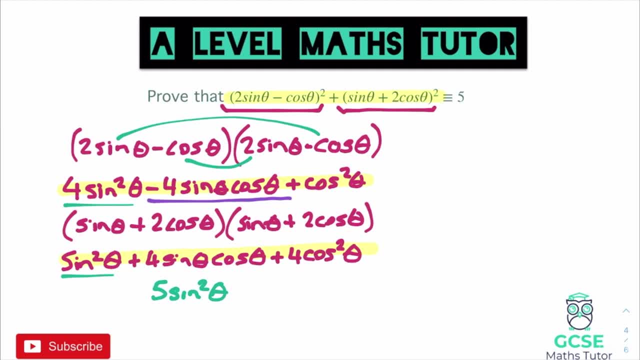 pieces. So we've got the negative 4 sine theta cos theta, and the positive 4 sine theta cos theta. So they would just cancel out. And then we have the plus cos squared theta, and the plus 4 cos squared theta. So that would be equal to 5 cos squared theta. Now we need to figure out how we're going to make this always equal to 5. So we have two options. We could change the sine squared theta into a cos, or we could change the cos squared theta into a sine. So let's just think about our identity, and we'll put one of our rearrangements. So let's change one of them. We'll say that sine squared theta, or we could go, in fact, let's just go with cos squared theta. We'll say that cos squared theta is equal to, 1 minus sine squared theta. And that's going to allow us to change this cos squared theta here into 1 minus sine squared theta. So if we go about doing that, we would still have the 5 sine squared theta at the start, but we would now have 5 lots of 1 minus sine squared theta. 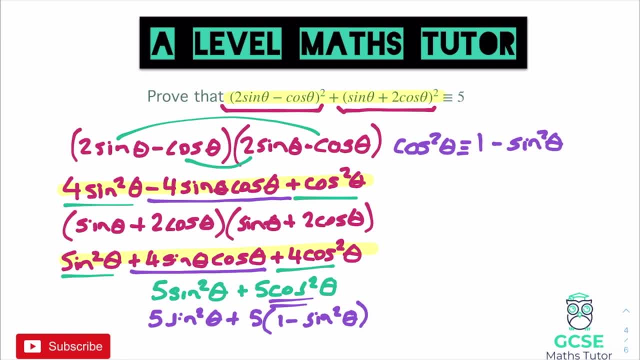 So just replacing the cos squared theta with 1 minus sine squared theta has now eliminated cos from our equation. So again, we could have done it the other way around. We could have got rid of sine and replaced that with cos using our other rearrangement, but it's absolutely fine for this one either way, 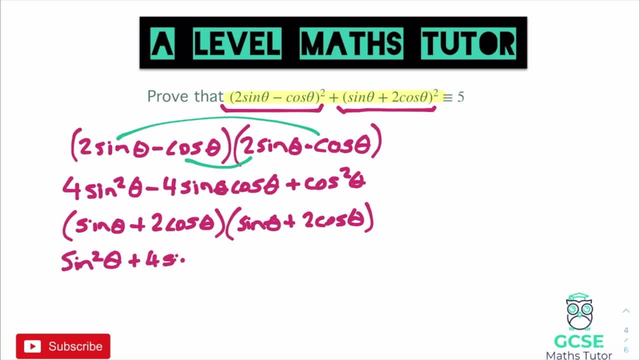 going to be plus 4 sin theta cos theta. There we go, And then we have the 2 cos theta times the 2 cos theta, which gives us plus 4 cos squared theta. So we've got our two pieces and we need to add them together after we had a plus sign. 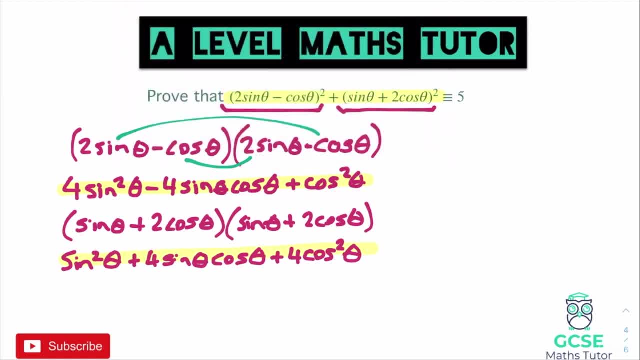 between these two. So if we add those two pieces together and let's see what we get. So we've got the 4 sin squared theta and a 1 sin squared theta here, so that would be equal to 5 sin squared. 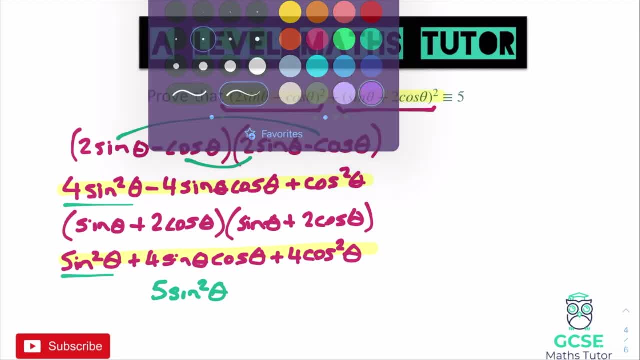 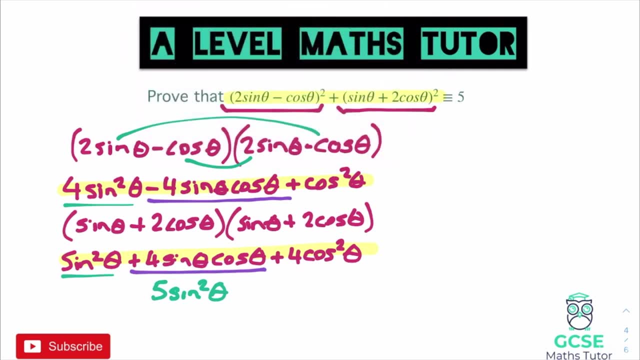 theta. We've then got these middle pieces, So we've got the negative 4 sin theta cos theta and the positive 4 sin theta cos theta. So they would just cancel out, And then we have the plus cos squared theta and the plus 4 cos squared theta, So that would be equal to. 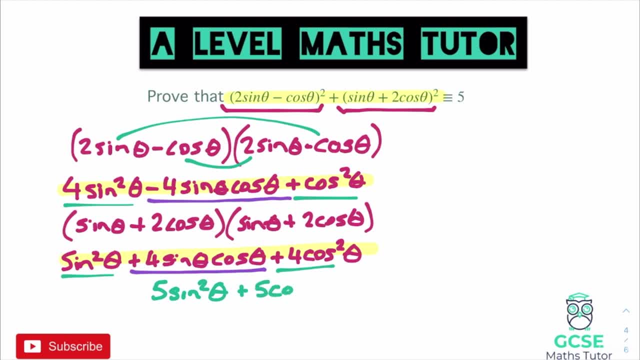 anyway, 5 cos squared theta. Now we need to figure out how we're going to make this always equal to 5.. So we have two options: We could change the sin squared theta into a cos, or we could change the cos squared theta into a sin. So let's just think about our identity and we'll put one of our 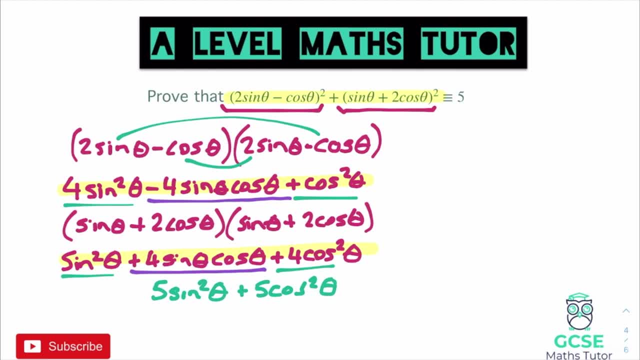 rearrangements. So let's change one of them. We'll say that sin squared theta – or we could go – in fact, let's just go that way, Let's change it, Let's put it in the positive, Let's just go with cos squared theta. We'll say that cos squared theta is equal to 1 minus. 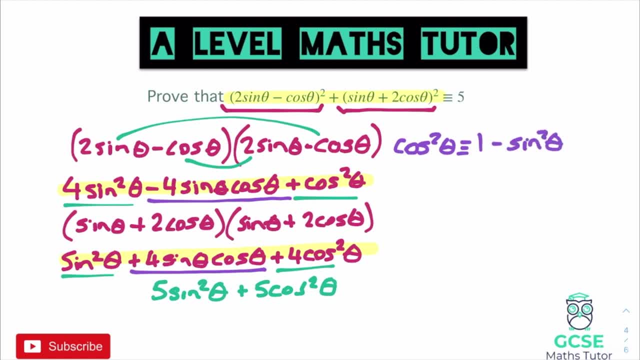 sine squared theta, And that's going to allow us to change this cos squared theta here into 1 minus sine squared theta. So if we go about doing that, we would still have the 5 sine squared theta at the start, but we would now have 5 lots of 1 minus sine squared theta. So just replacing the 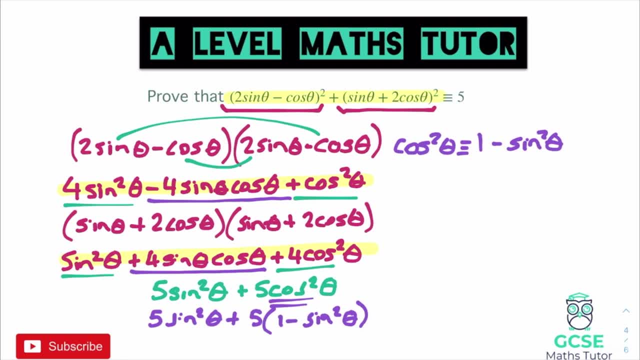 cos squared theta with 1 minus sine squared theta has now eliminated cos from our identity that we're looking at here. So again, we could have done it the other way around. We could have got rid of sine and replaced that with cos using our other rearrangement, but it's absolutely fine for. 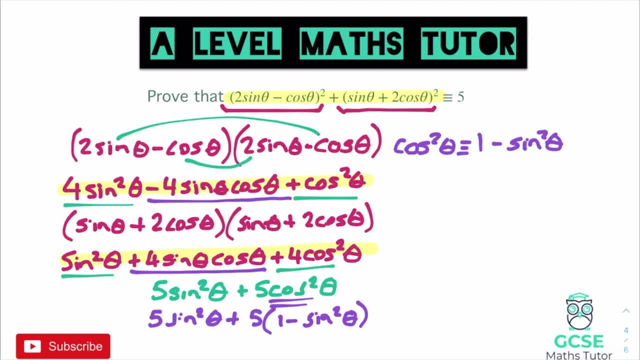 this one either way, as long as we just have sine. So now we could expand that bracket So we would have 5 sine squared theta and that would be plus 5 minus 5 sine squared theta. There we go. So where are we going to go from here? Now, if we bring that up to the top? 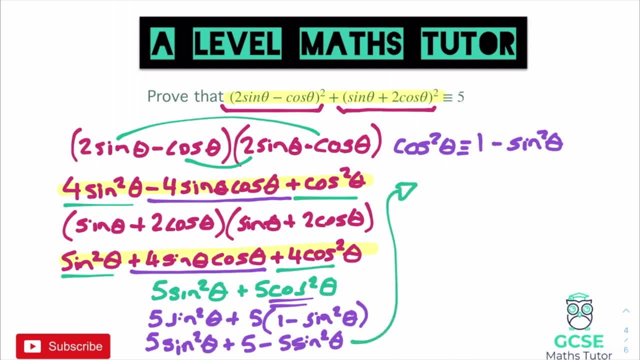 let's just have a look at what we've got there. We have got a- and let's just highlight it- 5 sine squared theta and a minus 5 sine squared theta, which means they're going to cancel out, which just leaves us with the plus 5, so we just have the answer 5.. So, because we've got, 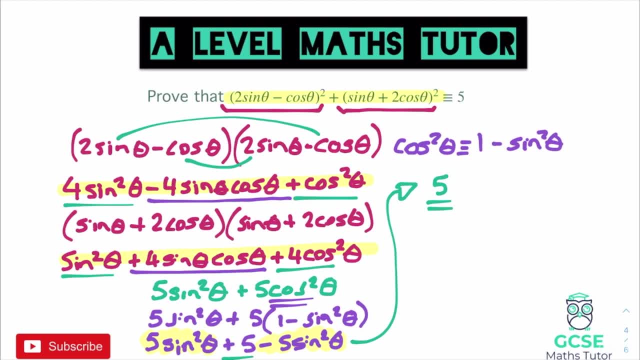 the answer 5. there we have obviously proved that. all of that just simplified down to 5. so therefore we have proved our identity, that the 2 sine theta minus cos theta squared, plus the sine theta plus 2 cos theta squared, is identical to 5, and we've proved all of that. So there we go. that's all we. 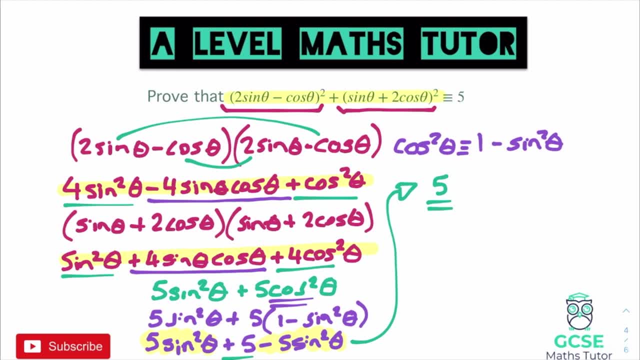 had to do. obviously, we only had to use one of our identities. we use this one just here and again. you could have done that a slightly different way by rearranging it, but again you'd have just got to the answer 5, because you would have had a 5 cos squared theta and a minus 5 cos squared theta, and 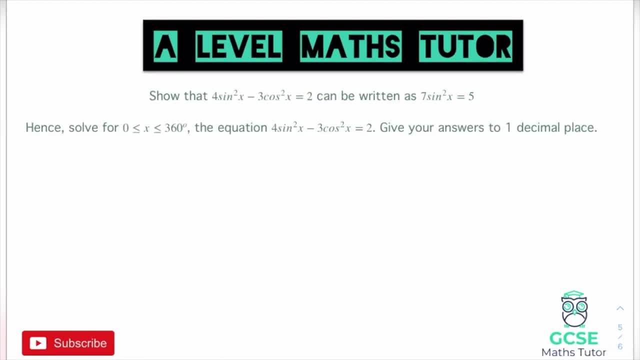 it would have all just cancelled out and you'd have been left with 5.. Okay, so, moving on to our first trigonometric equation. this is going to be quite a tricky one, quite a long one and quite tricky to fit all on the screen, but I think we'll just manage to fit it in. So the first: 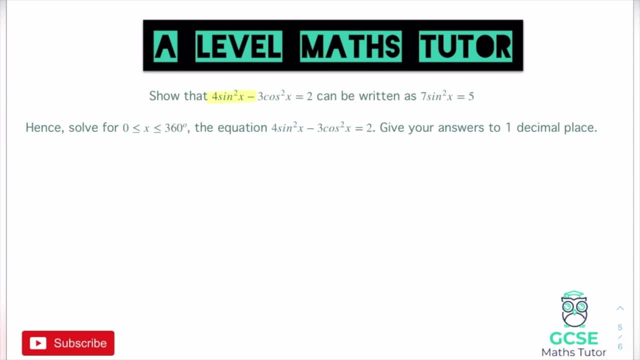 part here says: show that 4 sine squared x minus 3 cos squared x is equal to 2 can be written as: 7 sine squared x is equal to 5.. So the first thing to notice here is that in our second part we only have sine. so in our first piece here we're going to want to try and eliminate this cos. 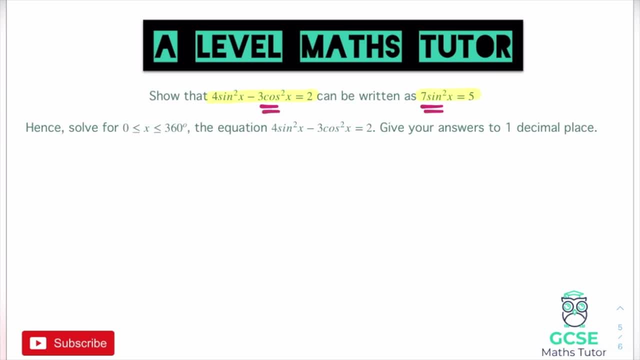 So if we eliminate that, we're going to want to think about which identity would help us to eliminate that. and that is that cos squared theta is equal or identical to 5 cos theta. So we're going to want to eliminate that. so we're going to want to. 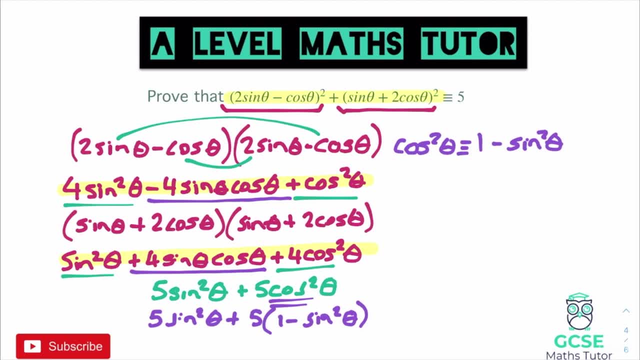 as long as we just have sine. So now we could expand that bracket. So we would have 5 sine squared theta, and that would be plus 5 minus 5 sine squared theta. 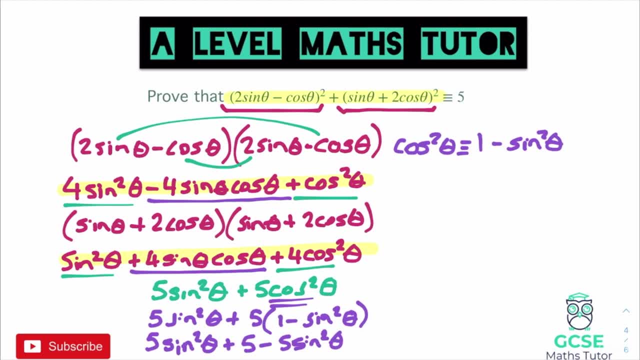 There we go. So where are we going to go from here? Now, if we bring that up to the top, let's just have a look at what we've got there. We have got a, and let's just highlight it, 5 sine squared theta and a minus 5 sine squared theta, which means they're going to cancel out, which just leaves us with the plus 5. 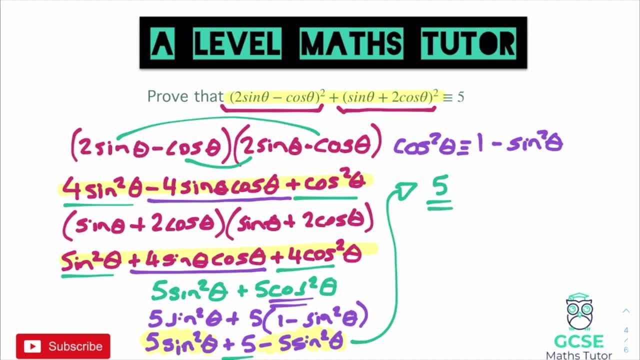 So we just have the answer 5. So because we've got the answer 5 there, 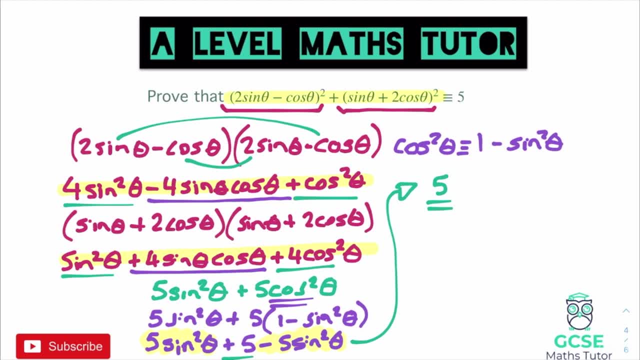 we have obviously proved that all of that just simplified down to 5. So therefore, we have proved our identity. 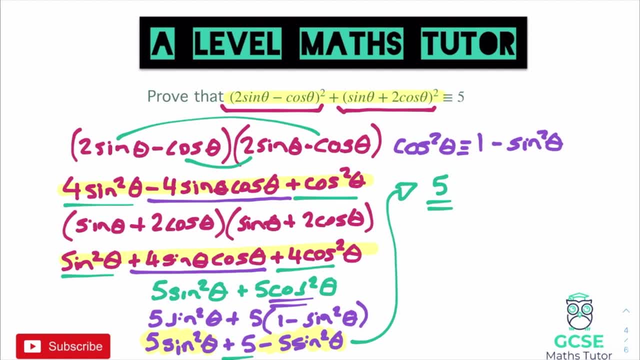 That the 2 sine theta minus cos theta squared plus the sine theta plus 2 cos theta squared is identical to 5, and we've proved all of that. So there we go. That's all we had to do. 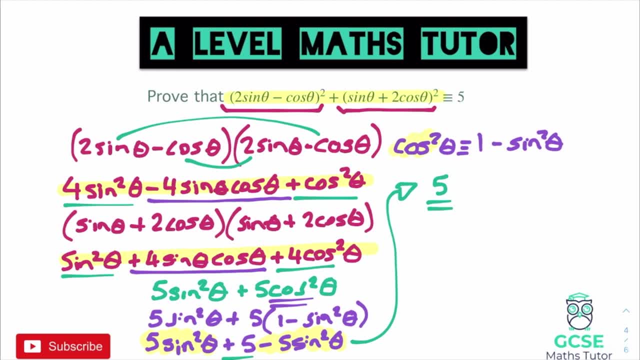 Obviously, we only had to use one of our identities. We used this one just here. And again, you could have done that a slightly different way by rearranging it. 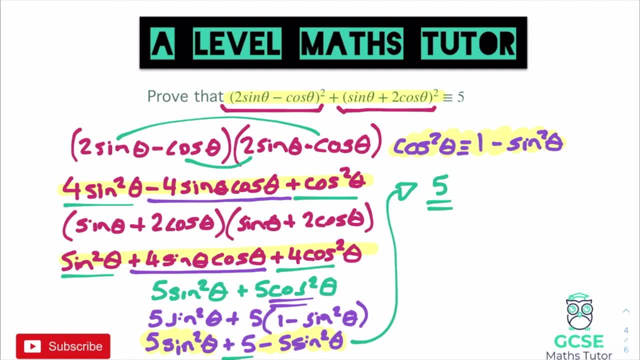 But again, you'd have just got to the answer 5, because you would have had a 5 cos squared theta and a minus 5 cos squared theta, and it would have all just cancelled out, and you'd have been left with 5. 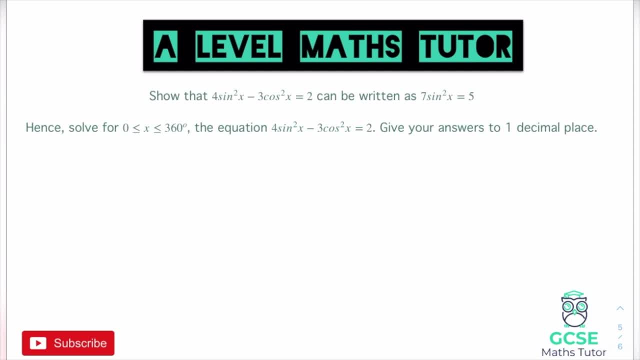 Okay, so moving on to our first trigonometric equation, this is going to be quite a tricky one. 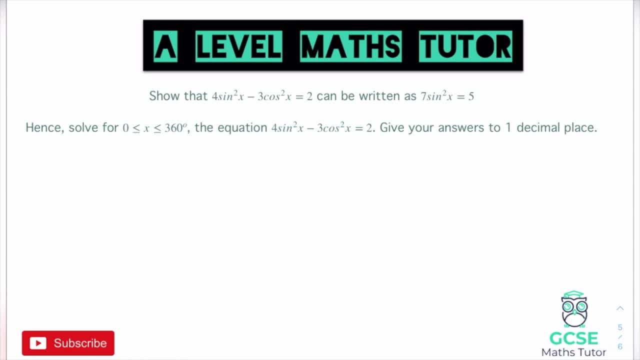 Quite a long one and quite tricky to fit all on the screen, but I think we'll just manage to fit it in. So the first part here says show that 4 sine squared x minus 3 cos squared x is equal to 2 can be written as 7 sine squared x is equal to 5. So the first thing to notice here is that in our second part, we only have sine. So in our first piece here, we're going to want to try and eliminate this cos. 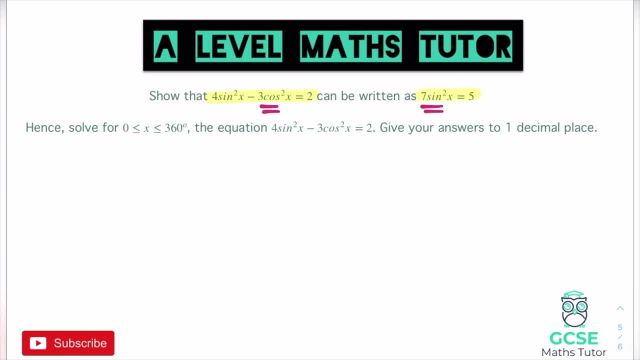 So if we eliminate that, we're going to want to think about which identity would help us to eliminate that, and that is that cos squared theta is equal or identical to 1 minus sine squared theta. So if we replace that cos squared theta with 1 minus sine squared theta, it's obviously going to start getting us towards our final answer. 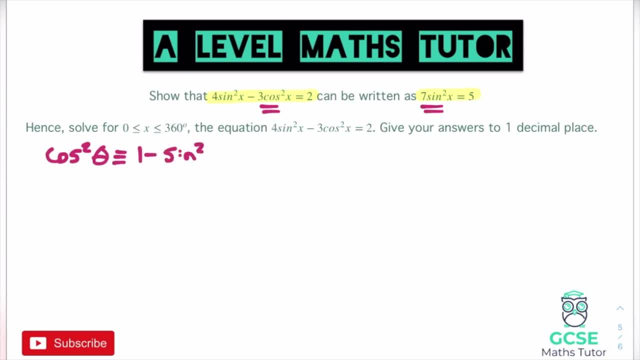 to one minus sine squared theta. So if we replace that cos squared theta with one minus sine squared theta, it's obviously gonna start getting us towards our final answer. So if we go about doing that, we have four sine squared theta or sine squared x. sorry. 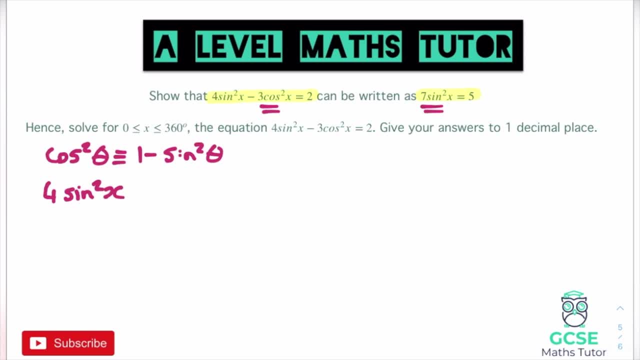 because we've got an x in this, as we're looking at an equation That is going to be now minus three, lots of one minus sine squared x. There we go, and that is equal to two. Now, if we expand that bracket, we've got four sine squared x minus three. 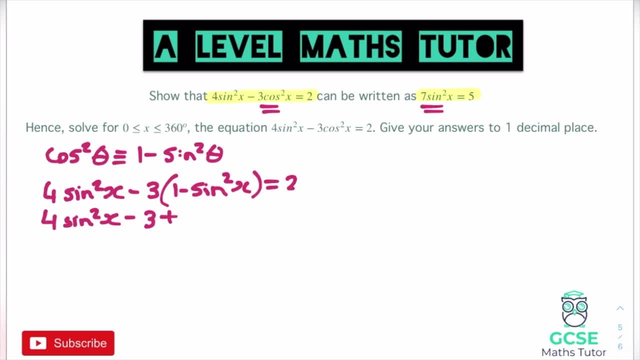 that's negative three times negative sine squared x. so plus three sine squared x is equal to two. There we go. Now we can add together our sine squared x. We've got four sine squared x plus three sine squared x. That adds together to make seven. 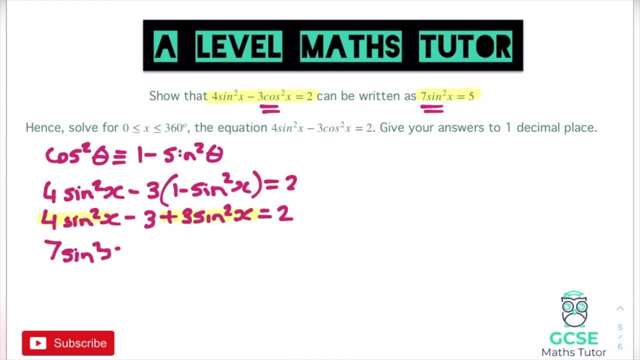 sine squared x. So you can already see we've got something which is matching that seven sine squared x. We also have that minus three is equal to two, And now we could minus two from both sides, or we could add three to the other side. 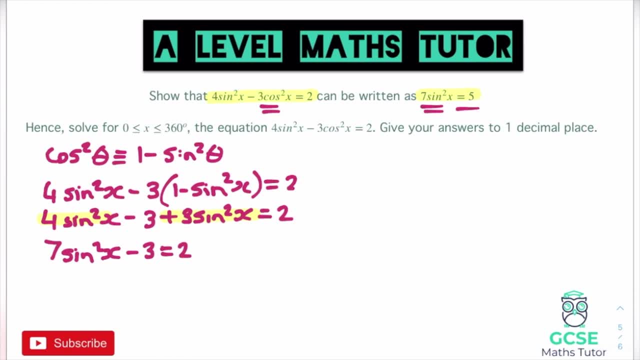 Now, looking at the equation up here, what it wants us to be written as it says it's equal to five. So we want to add three to the other side, which would give us seven. sine squared, x is equal to five. And there we are: we have showed that it equals that. 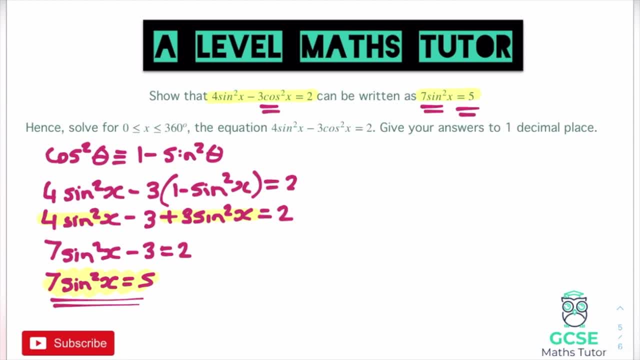 So that would be our final answer, and we have shown that correctly using our trigonometric identity. Part B here says: hence: solve for values between zero and 360, including zero and 360, that this equation here is equal to two. 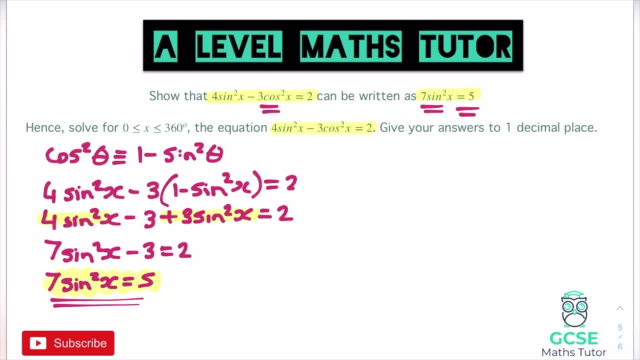 So we're going to solve this equation and we're going to give our answer to one decimal place, or our answers to one decimal place. So we'll have a look at this and think about how we'll go about answering this. So we'll have a look at this and think about how we'll go about answering this. 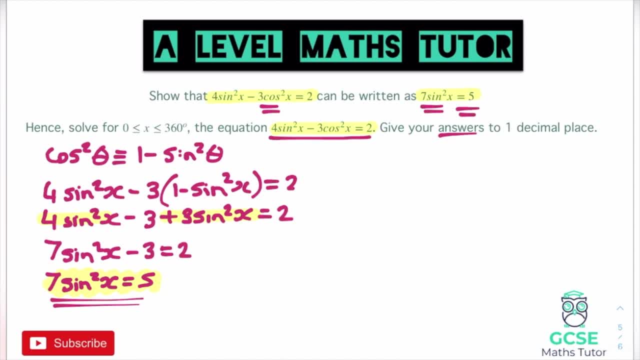 Now, of course, this equation here we have just shown can be written as this equation here, Now that we would not be asked to do that unless it was going to be useful. Now, the reason it's useful is the second equation that we have shown only has sine in. 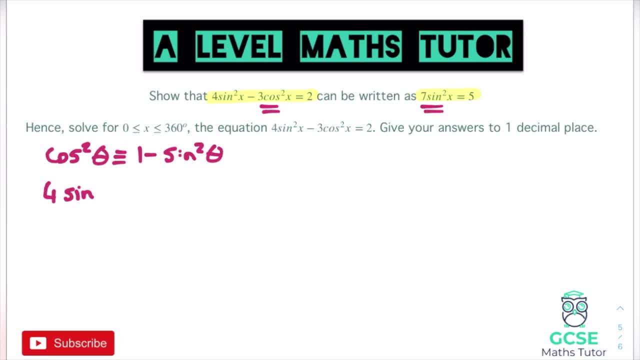 So if we go about doing that, we have 4 sine squared theta, or sine squared x, sorry, because we've got an x in this. 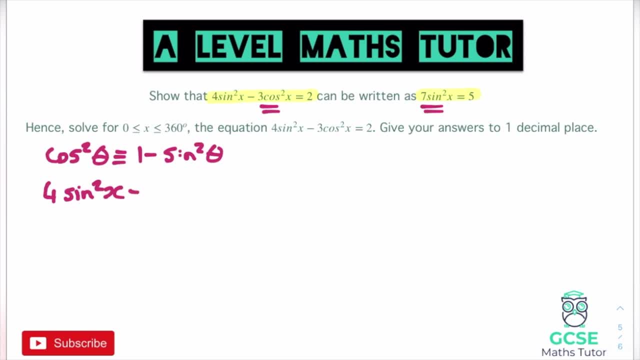 As we're looking at an equation, that is going to be now minus 3 lots of 1 minus sine squared x. There we go, and that is equal to 2. 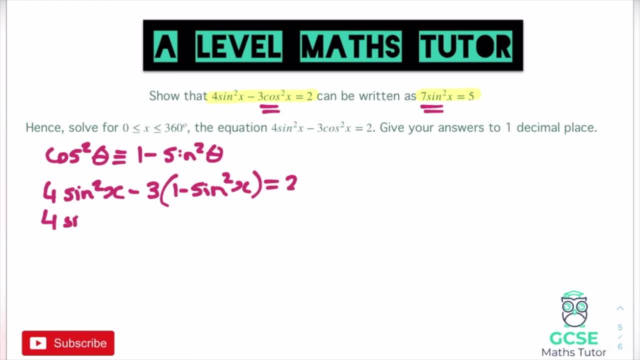 Now if we expand that bracket, we've got 4 sine squared x minus 3. That's negative 3 times negative sine squared x, so plus 3 sine squared x. That's equal to 2. There we go. Now we can add together our sine squared x. We've got 4 sine squared x plus 3 sine squared x. 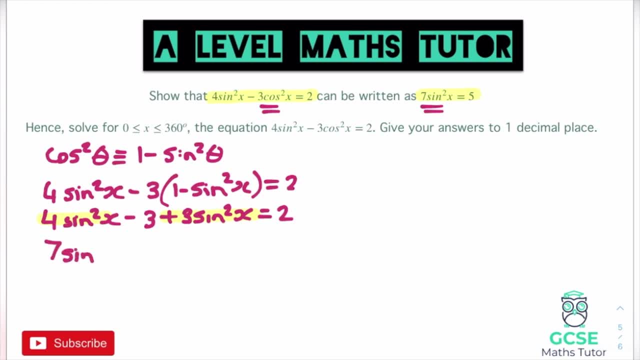 That adds together to make 7 sine squared x. So you can already see we've got something which is matching that 7 sine squared x. 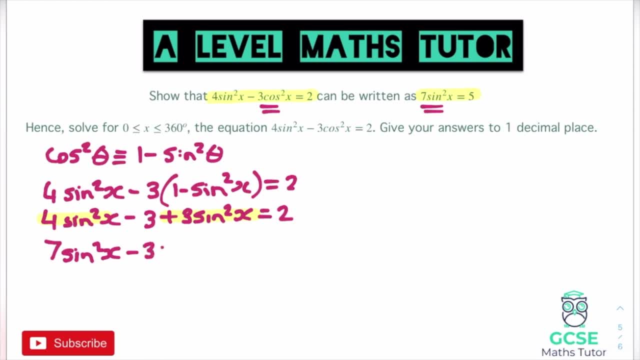 We also have that minus 3 is equal to 2. 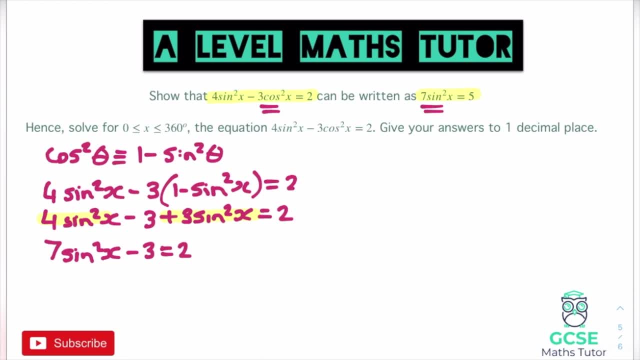 And now we could minus 2 from both sides, or we could add 3 to the other side. Now looking at the equation up here, what it wants us to be written, as it says it's equal to 5. 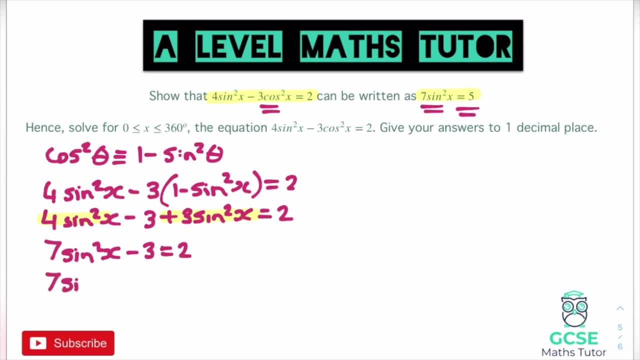 So we want to add 3 to the other side, which would give us 7 sine squared x is equal to 5. And there we are. 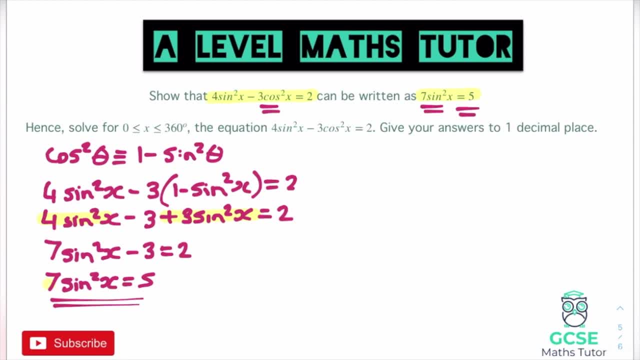 We have showed that it equals that. So that would be our final answer, and we have shown that correctly using our trigonometric identity. 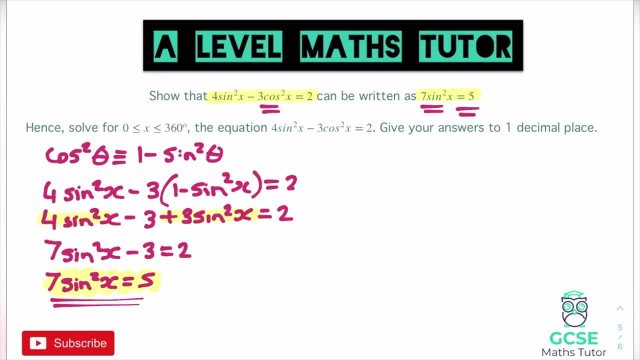 Part B here says, hence solve for values between 0 and 360, including 0 and 360, that this equation here is equal to 2. So we're going to solve this equation, and we're going to give our answer to one decimal place, or our answers to one decimal place. So we'll have a look at this and think about how we'll go about answering this. Now of course this equation here we have just shown can be written as this equation here. 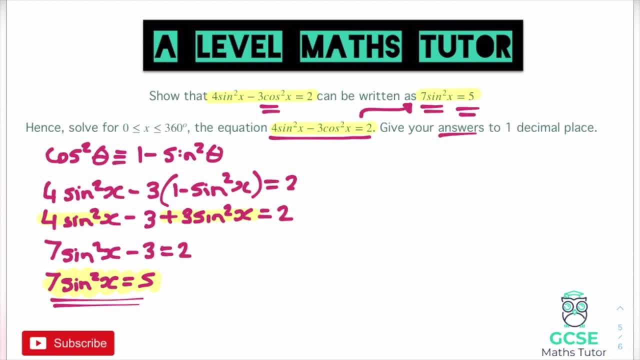 Now we would not be asked to do that unless it was going to be useful. 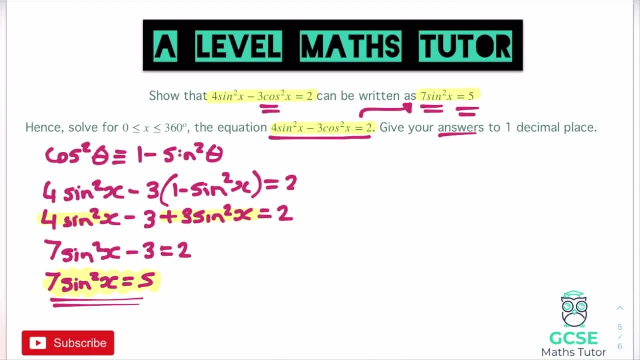 Now the reason it's useful is the second equation that we have shown only has sine in. So we're going to be able to use our sine graph to find our solutions, and how we'll go about doing that. 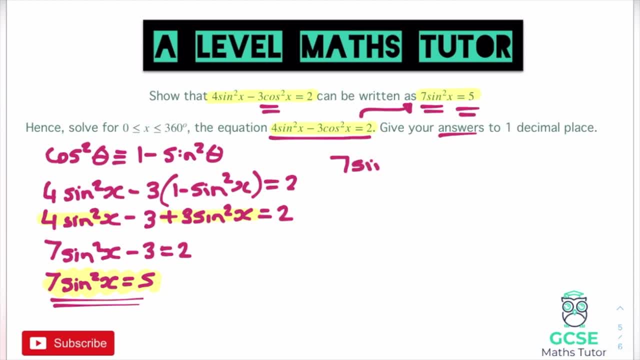 So at the moment we have 7 sine squared x is equal to 5, and we're going to go about solving it. And you'll notice this with a lot of these questions, that that part that it's asking you to show it as how it can be written is going to be used in the second part of the question. So to go about solving this, we want to get what sine x is equal to. So if we divide both sides by 7, we'll know what sine squared x is equal to. 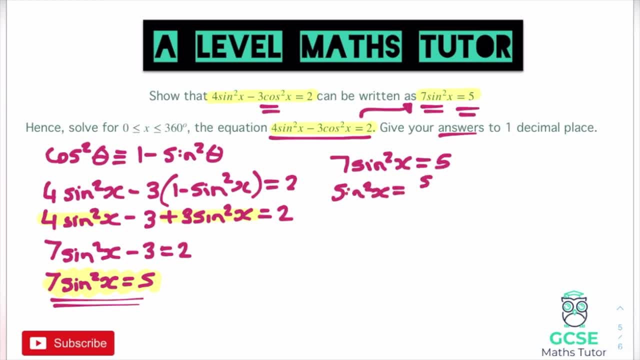 So sine squared x is equal to 5 over 7. Now to get what sine x is equal to we just need to square root both sides. So we're going to have that sine x is equal to, and don't forget when you square root you have plus and minus, so plus and minus the square root of 5 over 7. 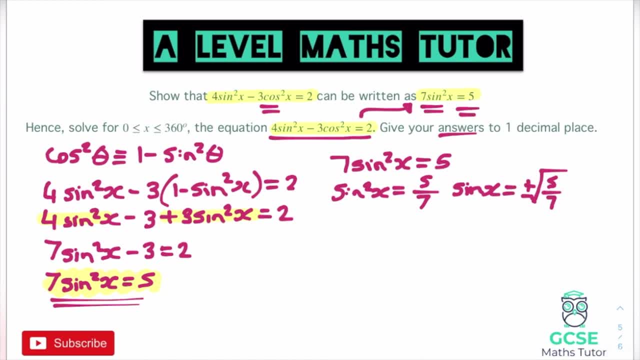 So there we go, that's what sine x is equal to, and now we can actually use our calculator to do shift sine and find the values there. 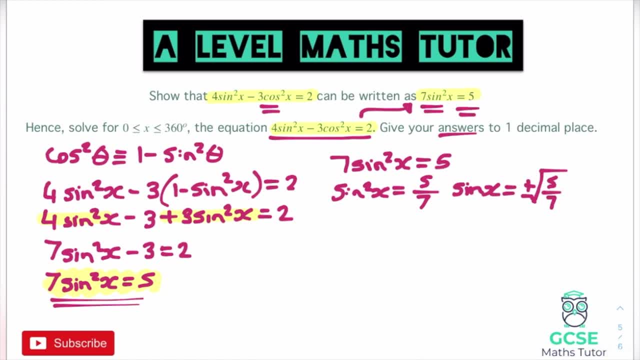 And if we put that into our calculator, let's do the positive one to start with. So sine minus 1 of, and let me just type it in, the square root of 5 over 7, let's have a look, let's just write this down, so sine minus 1 of 5 over 7 is equal to, and we get 57.688, so it wanted it all to one decimal place, so 57.7 degrees. 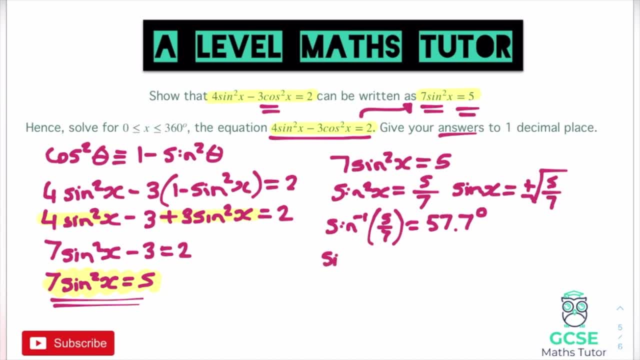 If we do the same for our next one, so sine minus 1 of negative 5 over 7, and again, just go into your calculator, sorry, the square root of, I've just realised I forgot to put the square root symbol there, put that in, I had to type that in on the calculator, we'll go back, we'll put the negative 5 over 7, close our bracket, and for this one, we get the same answer, but the negative version, so negative 57.7 degrees. 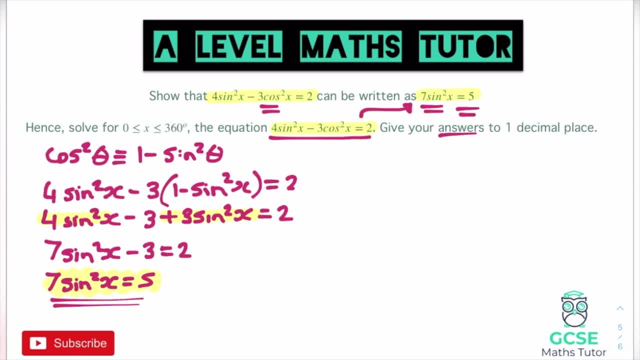 So we're going to be able to use our sine graph to find our solutions and how we'll go about doing that. So at the moment we have seven sine, squared x is equal to five, and we're going to go about solving it. 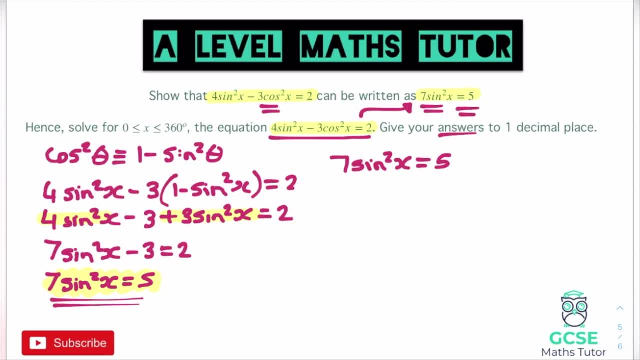 And you'll notice this with a lot of these questions- that that part that it's asking you to show it as how it can be written is going to be used in the second part of the question. So to go about solving this, we want to get what sine x is equal to. 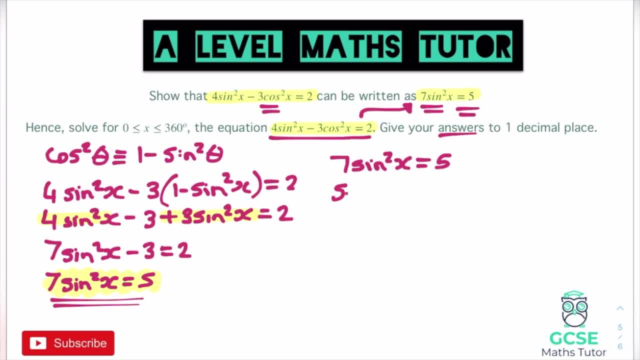 So if we divide both sides by seven, we'll know what sine squared x is equal to. So sine squared x is equal to five over seven. Now to get what sine x is equal to, we just need to square root both sides. So we're going to have that sine x is equal to. 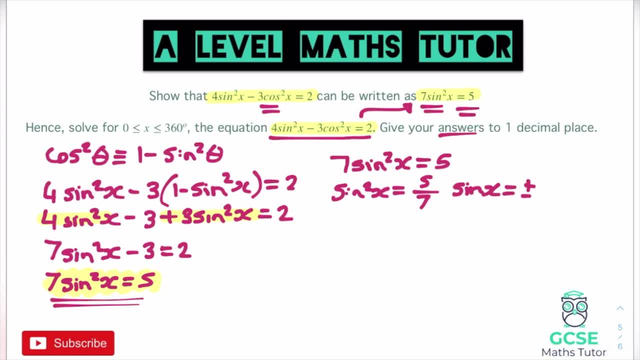 and don't forget, when you square root you have plus and minus. so plus and minus the square root of five over seven. So there we go. that's what sine x is equal to. And now we can actually use our calculator to do shift sine and find the values there. 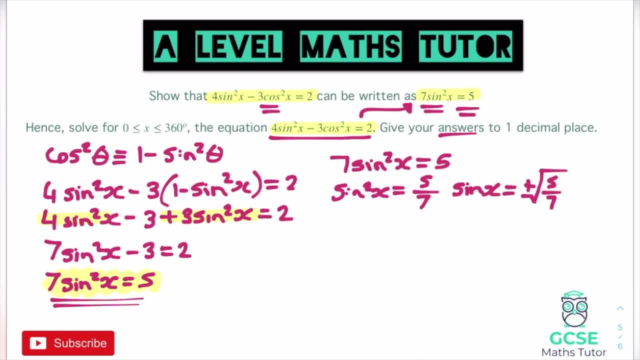 And if we put that into our calculator, let's do the positive one to start with, So sine minus one of, and let me just type it in the square root of five over seven. Let's have a look, let's just write this down. 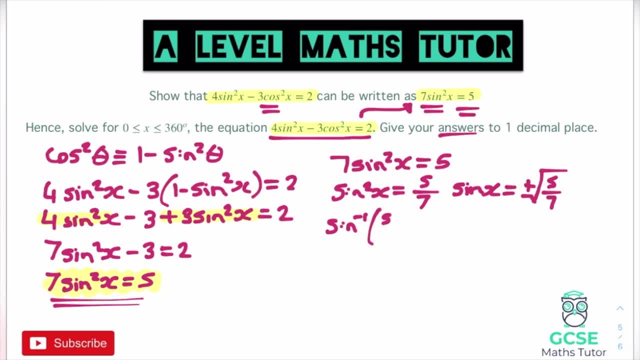 So sine minus one Of five over seven is equal to, and we get 57.688, so it wanted it all to one decimal place. so 57.7 degrees If we do the same for our next one. so sine minus one of negative five over seven. 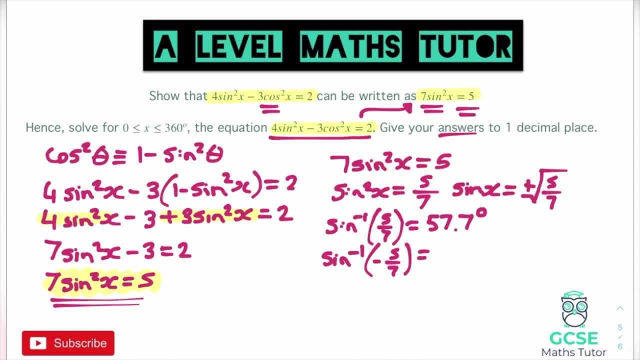 And again just go into your calculator. sorry, the square root of. I've just realised I forgot to put the square root symbol there. Put that in. I had typed that in on the calculator. We'll go back. we'll put the negative five over seven. 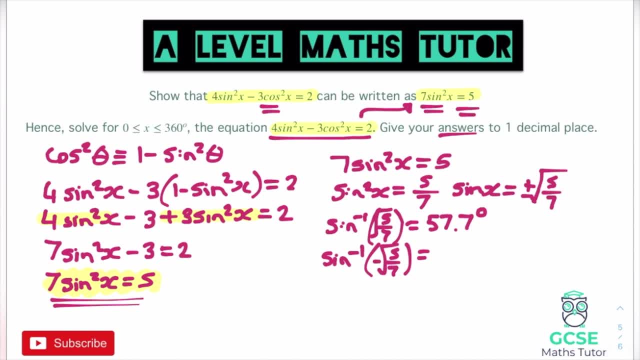 close our bracket And for this one we get the same answer, but the negative version. so negative 57.7 degrees. So we have actually solved our equation here. We've got two answers, We've got 57.7, and refer back to our ranges here. 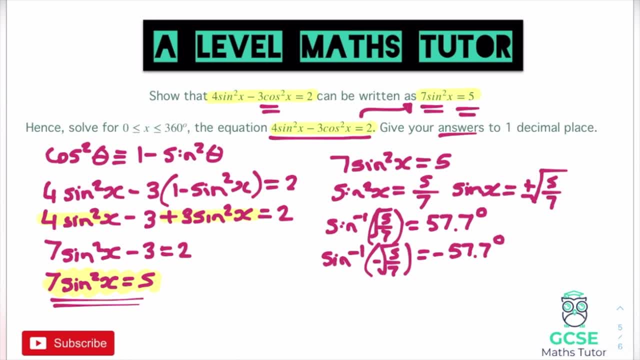 So we have actually solved our equation here, we've got two answers, we've got 57.7, and refer back to our ranges here, so it's between 0 and 360, but this negative 57.7 falls outside of that, so that's not going to be one of our solutions. However, it is going to be able to help us to find all of our solutions on our sine graph, so we're going to use these answers to see if we've got any other solutions. 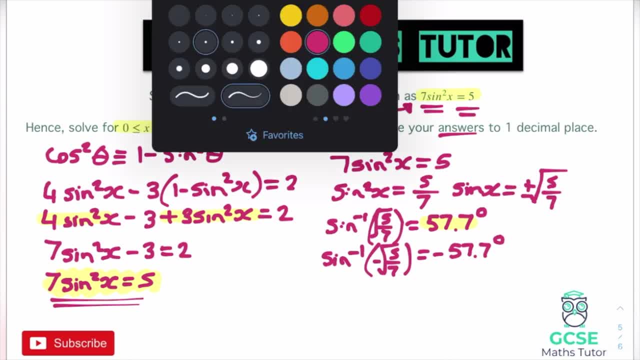 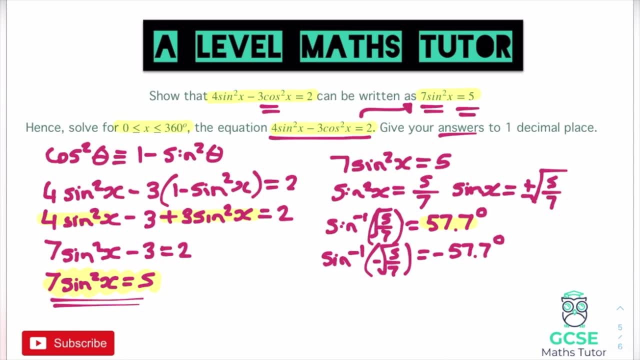 And this is where it comes into play that it helps to be able to draw the sine graph, and again, this is where you can use different solutions, you can use your quadrant method if you would prefer to, that's absolutely fine, but as I've said before, I think it's really important you know these graphs, so I always like to discuss them. So if we look at the sine graph, and we draw a basic sketch of what it looks like, if we actually draw that, sine starts in the origin, obviously it goes up to 1 and down to minus 1, and it goes along from 90, 180. 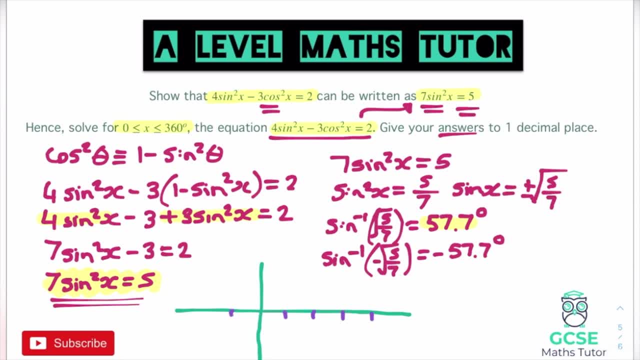 270, 360, and we'll go back a little bit as well as we have that negative value, and if I was to draw that in, and again, it's just a little sketch, just so we can visualize it, it would look something like that. So if we label on our points, negative and the positive side, 90, 180, 270, and 360, and then we'll have negative 90, and also negative 180. And let's just imagine where these points are. 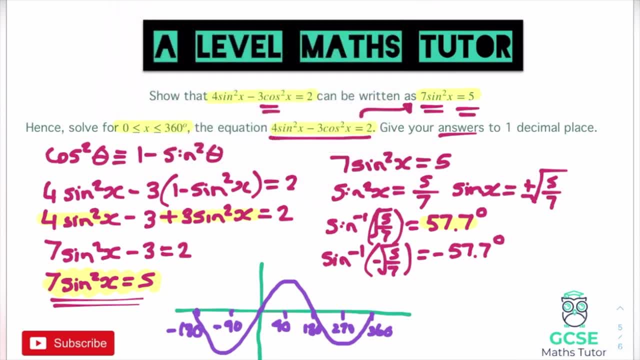 So the points that we have, we've got 57.7, which would lie between 0 and 90, so that would be just there, and we've got the negative 57.7, which is between 0 and negative 90, just here. So in order to find all of our solutions, all we have to do is trace along between 0 and 360, and see where these points hit any other points on the curve. 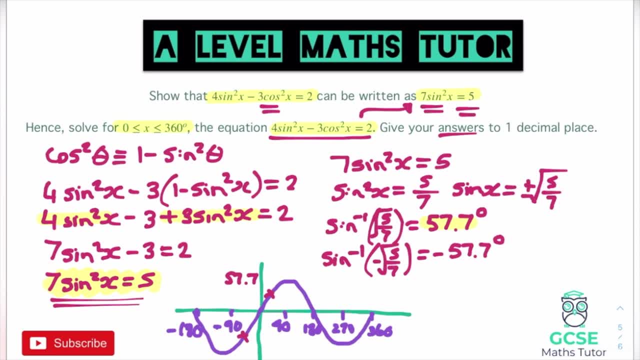 So we obviously have our 57.7 just here, and if we go to the right, we obviously hit the curve at another point. So in order to find that one, we can just think about on the graph. 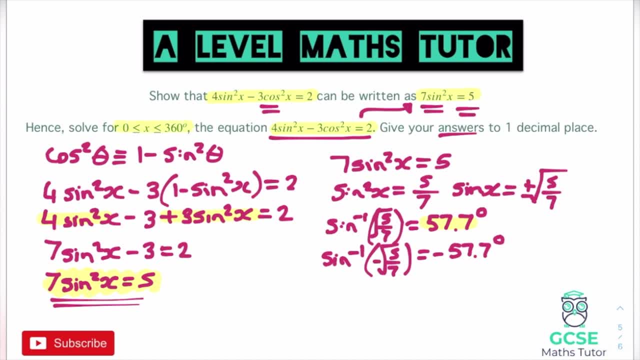 So it's between nought and 360.. But this negative 57.7 falls outside of that, So that's not going to be one of our solutions. However, it is going to be able to help us to find all of our solutions on our sine graph. 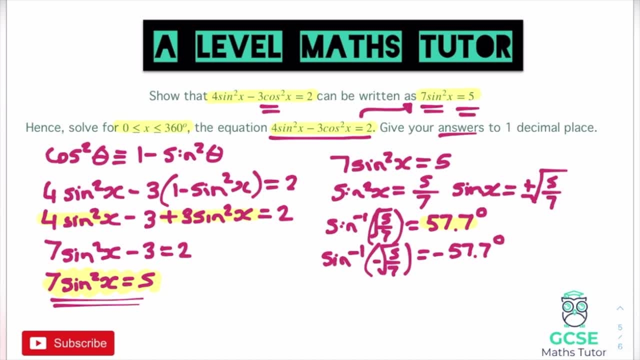 So we're going to use these answers to see if we've got any other solutions. And this is where it comes into play that it helps to be able to draw the sine graph. And again, this is where you can use different solutions. You can use your quadrant method if you would prefer to. 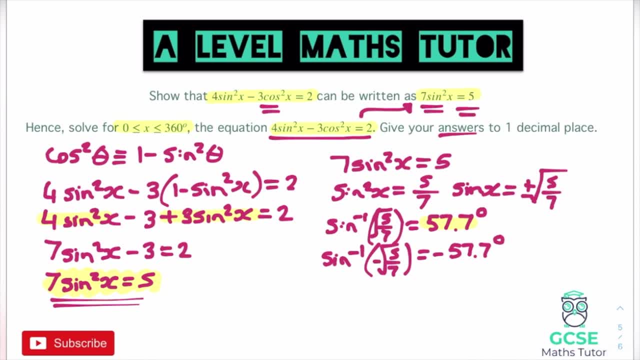 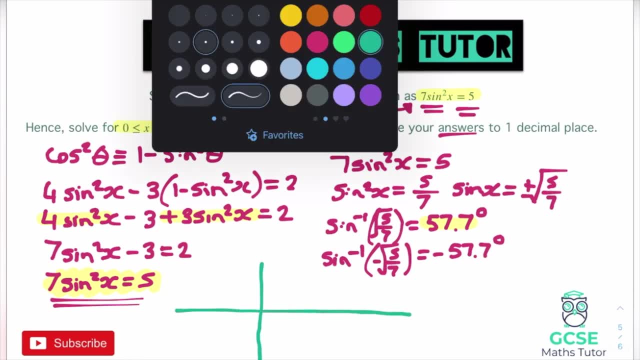 That's absolutely fine, But, as I've said before, I think it's really important. you know these graphs, so I always like to discuss them. So if we look at the sine graph and we draw a basic sketch of what it looks like, 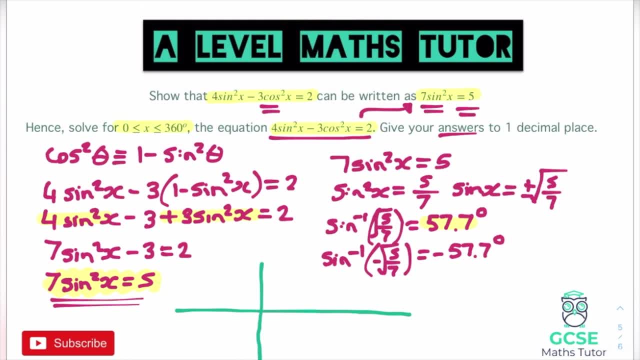 If we actually draw, that sine starts in the origin. Obviously it goes up to one and down to minus one And it goes along from 90, 180, 270, 360.. And we'll go back a little bit as well. 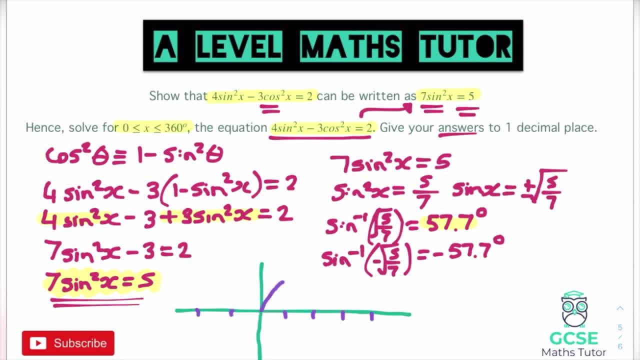 as we have that negative value. And if I was to draw that in- and again, it's just a little sketch, just so we can visualize it- it would look something like that. So if we label on our points negative and the positive side, 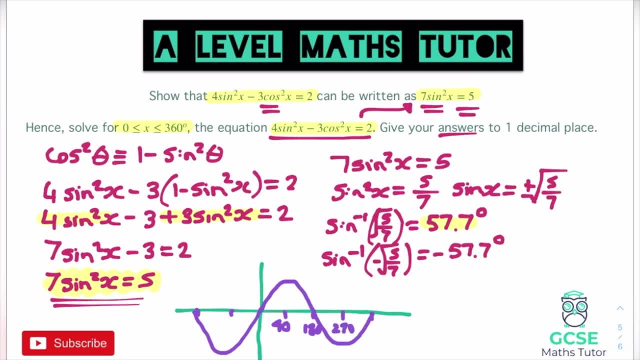 90,, 180,, 270, and 360. And then we'll have negative 90, and also negative 180.. And let's just imagine where these points are. So the points that we have, we've got 57.7,. 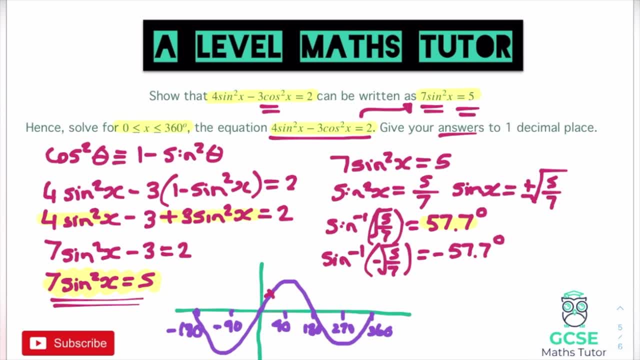 which would lie between nought and 90, so that would be just there, And we've got the negative 57.7, which is between nought and negative 90, just here. So, in order to find all of our solutions, all we have to do is trace along. 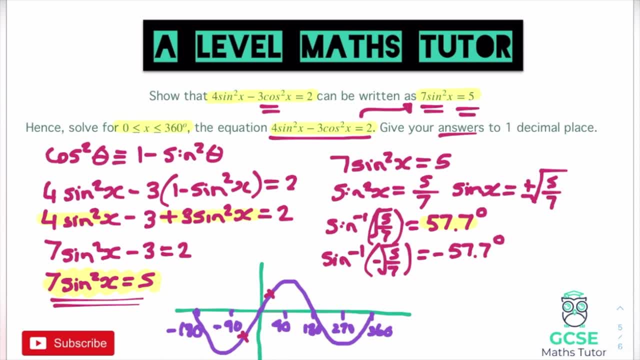 between nought and 360 and see where these points hit any other points on the curve? So we obviously have our 57.7 just here, And if we go to the right, we obviously hit the curve. another point just here. So, in order to find that one, 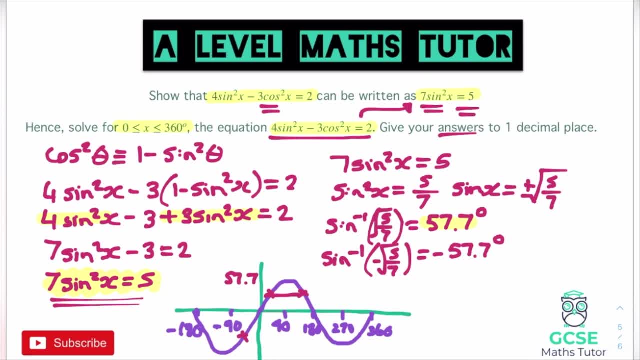 we can just think about on the graph Now, 57.7 is 57.7 away from zero. So to find that one on the right we would just do 180 and take away 57.7. And if we work that out and turn it into a decimal, 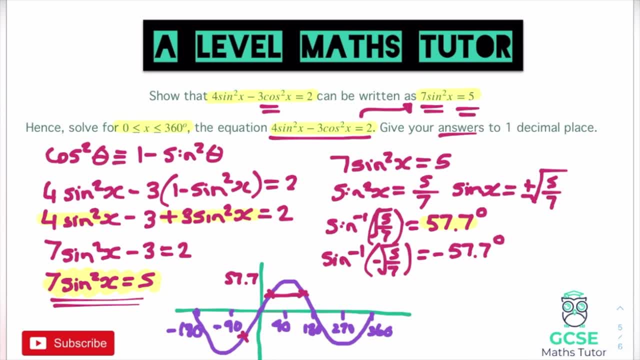 Now 57.7 is 57.7 away from 0, so to find that one on the right, we would just do 180, and take away 57.7. And if we work that out and turn it into a decimal, that comes out as 122.3. 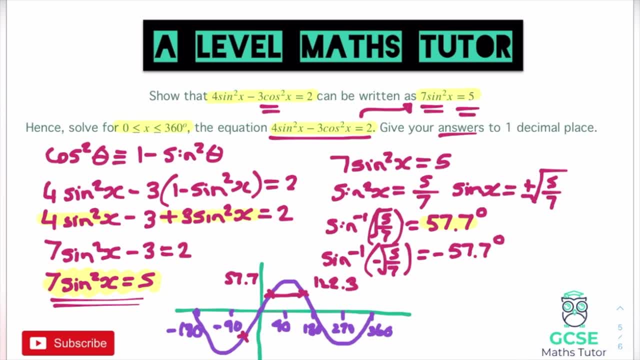 And there's one of our other solutions, and that's between 0 and 360. If we go down to the bottom one, at the negative 57.7, and we go across from that, we hit the curve here, and if we keep on going, we hit the curve again here, and that is between 0 and 360. So we have two more solutions just there. 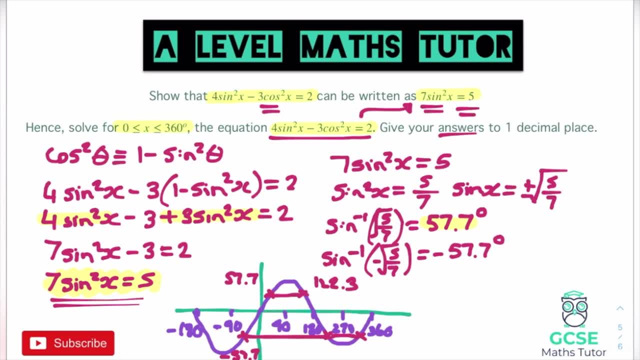 So to find that one, if we add 57.7 to the 180, then that is going to find our next solution. So if we do 180, add 57.7. 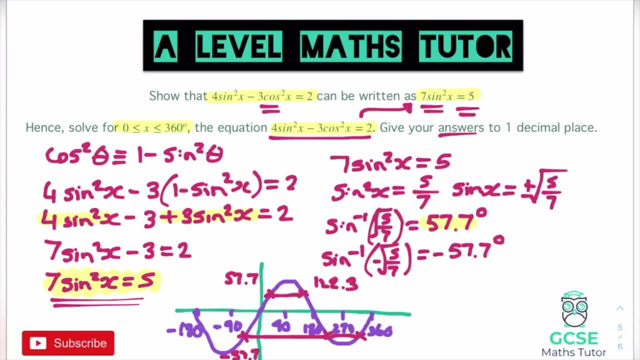 And make sure you type that in. If we type that in correctly, and there we go, that comes out as this one here, 237.7. And again, we can do that for the reverse. 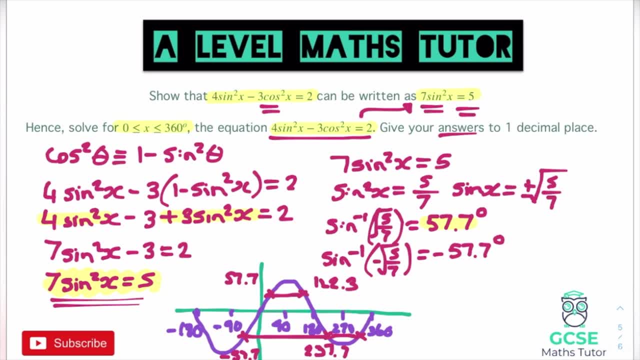 For the one next to it, we can do 360, take away 57.7, and that gives us our final answer there of 302.3. 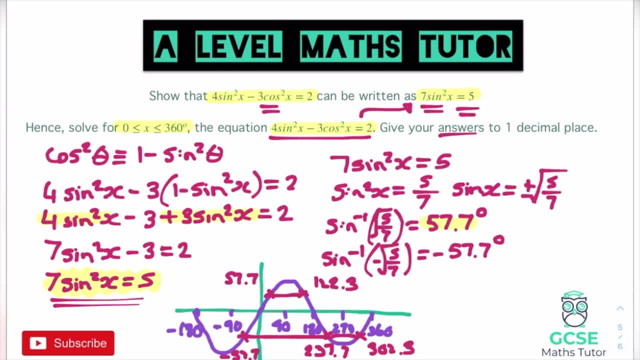 Now of course, there is another point on the graph, as I've obviously gone into the negatives, there is another point just here. But obviously that falls outside of our 0. 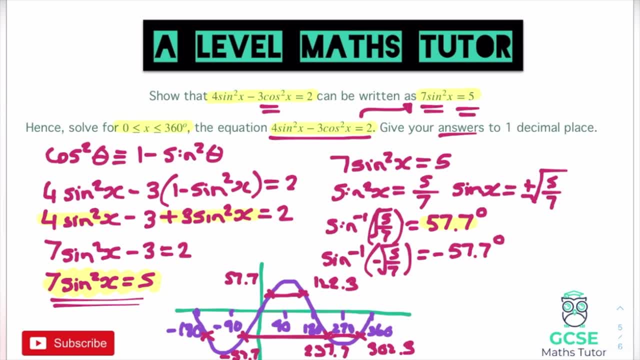 So that's not going to be a solution that we can use. 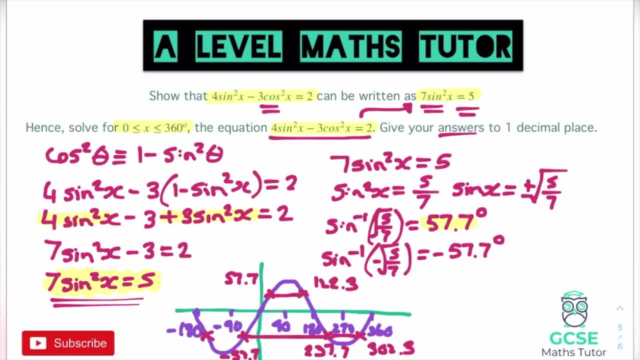 So the negative 57.7 we can't use, but we have got the 57.7, the 122.3 just here on that top part of the curve, and then we have also the 237.7 and the 302.3. 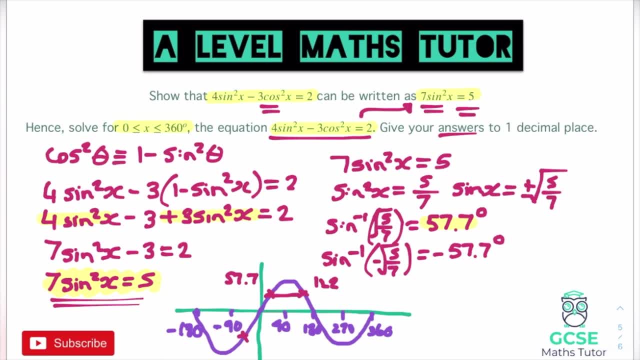 that comes out as 122.3.. And there's one of our other solutions and that's between nought and 360.. If we go down to the bottom one at the negative- 57.7, and we go across from that, we hit the curve here. 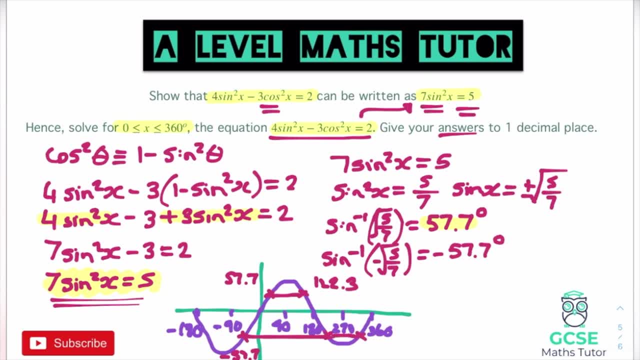 And if we keep on going, we hit the curve again here, and that is between nought and 360.. So we have two more solutions just there. So to find that one, if we add 57.7 to the 180,. 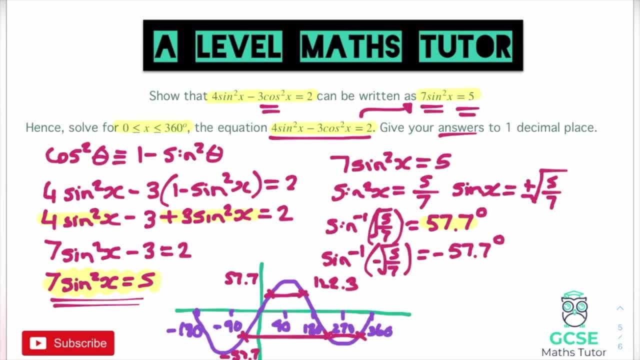 then that is going to find our next solution. So if we do 180, add 57.7, and make sure you type that in correctly, And there we go, That comes out as this one here, 237.7.. And again we can do that for the reverse. 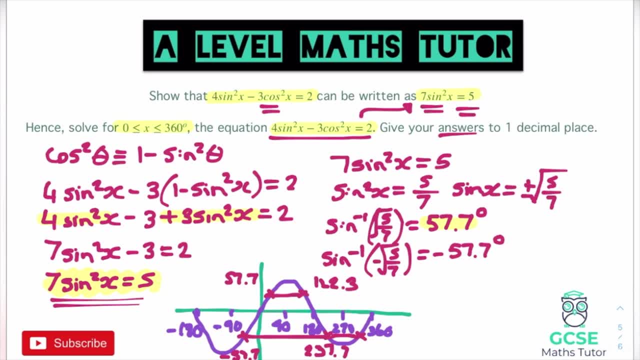 For the one next to it, we can do 360, take away 57.7.. And that gives us our final solution. So we've got our final answer there of 302.3.. Now, of course, there is another point on the graph. 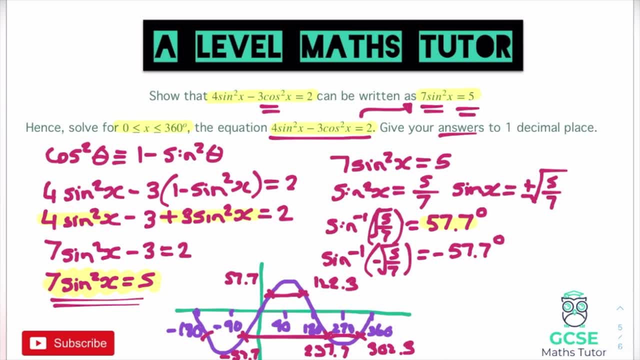 as I've obviously gone into the negatives. there is another point just here, but obviously that falls outside of our zero to 360 range, So that's not going to be a solution that we can use. So the negative 57.7, we can't use. 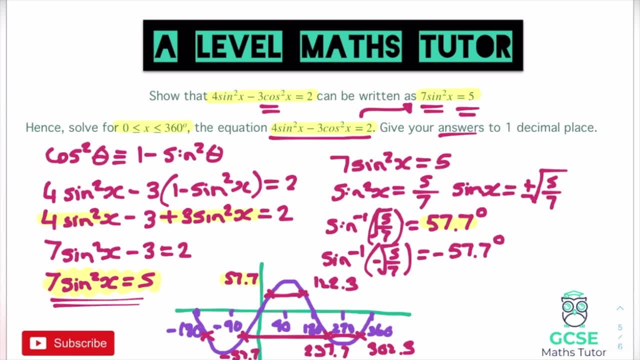 but we have got the 57.7,, the 122.3 just here on that top part of the curve, And then we had also the 237.7,, which is the negative 57.7., And the 302.3.. 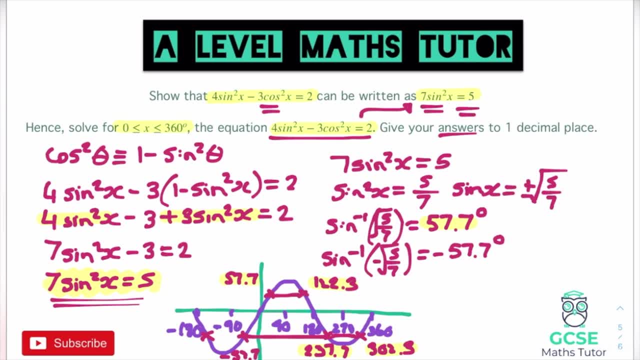 So we have four answers for this particular question. So we would give them. we would say that X is going to equal 57.7.. And paired with that we've got X is equal to 122.3 on the top part. 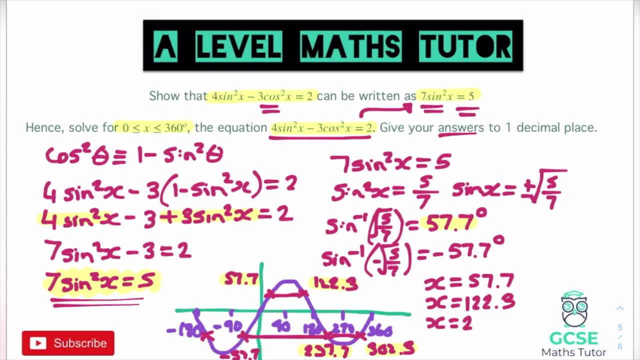 And then down the bottom we had: X was equal to 237.7.. And matched with that on the right there, on the right of that, was 302.3.. These are all degrees, So we would put degrees with all of them. 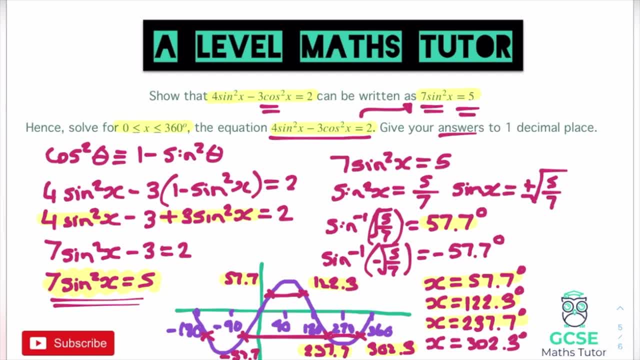 And there we go. They would be our four answers for this question, all given to one decimal place. So, as you can see, very important to know these trigonometric graphs and, obviously, knowing how to do your inverse of sine, and just getting that to the point where it was, sine X. 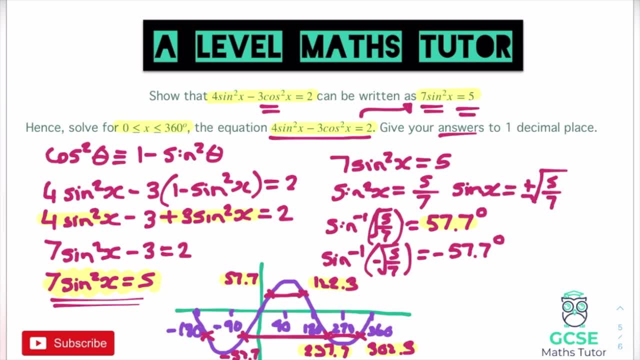 So we have four answers for this particular question. So we would give them, we would say that x is going to equal 57.7, and paired with that, we've got x is equal to 122.3 on the top part, and then down the bottom we had x was equal to 237.7, and matched with that on the right there, on the right of that was 302.3. These are all degrees, so we would put degrees with all of them, and there we go, they would be our four answers for this question, all given to one decimal place. 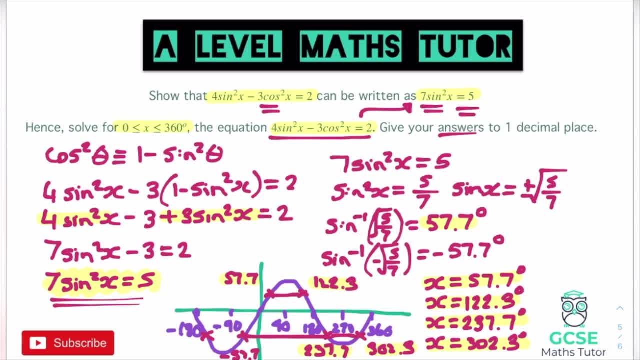 So as you can see, very important. to know these trigonometric graphs, and obviously knowing how to do your inverse of sine, 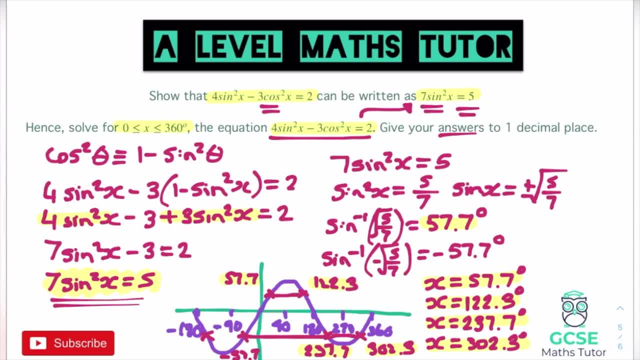 and just getting that to the point where it was sine x was equal to a number, so that we could actually find that amount in degrees and relate it to the trigonometric graph. 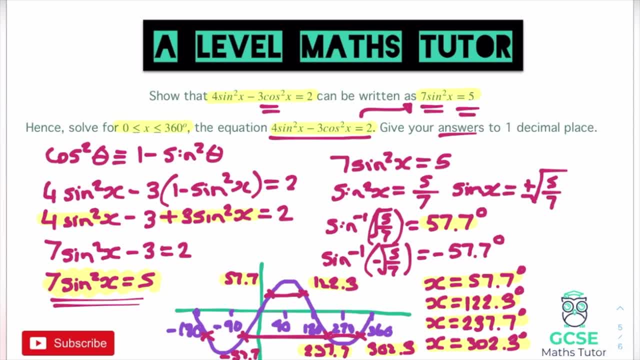 So that's one type of question, and obviously you can have harder ones than this, and we're going to have a look at some harder ones as well. 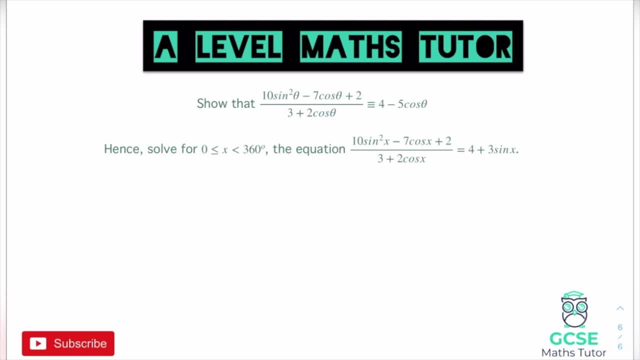 Okay, so looking at one of our harder trigonometric equations, you can see that it obviously doesn't look very nice. It says, 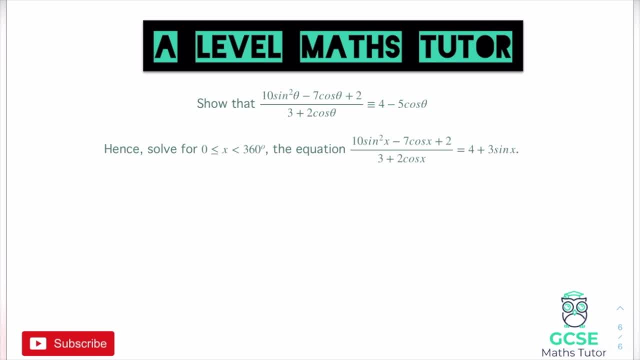 Then it asks us, hence solve, and we've got a very similar question to what we've looked at before. But we're going to start with this first part, and show that all of this comes out as 4-cosθ. Now straight away you can see that in our answer part there, that we're looking to show that it's identical to, it has a cos in. 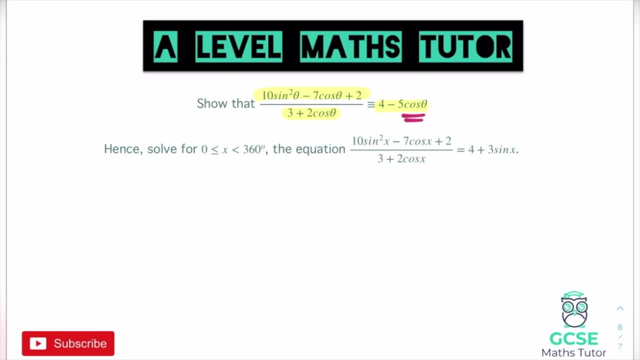 So for all of the pieces that have a sine in, or a sine squared theta in, we're going to want to turn that into a cos. 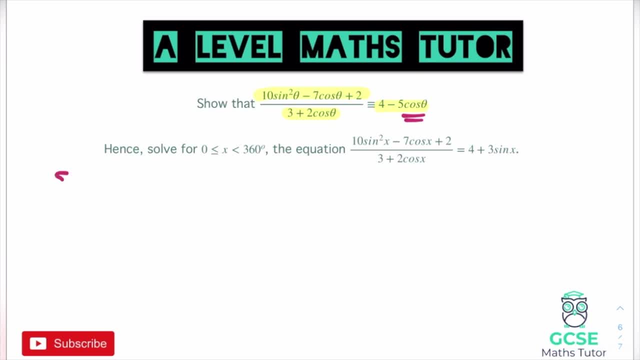 So straight away we'll write down our identity for that, and that is that sine squared theta is identical to 1 minus cos squared theta. 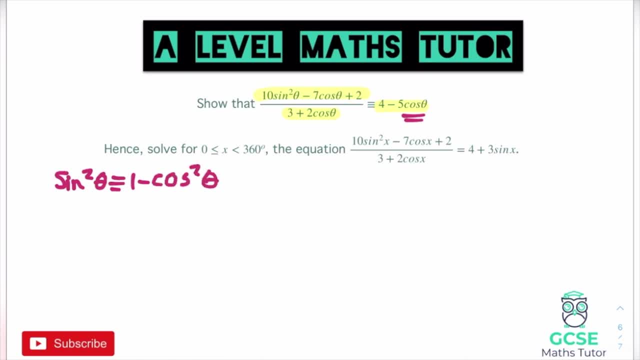 And we'll plug that in and see where we get to. So if we start by replacing the sine squared theta, we have 10 lots of 1 minus cos squared theta. 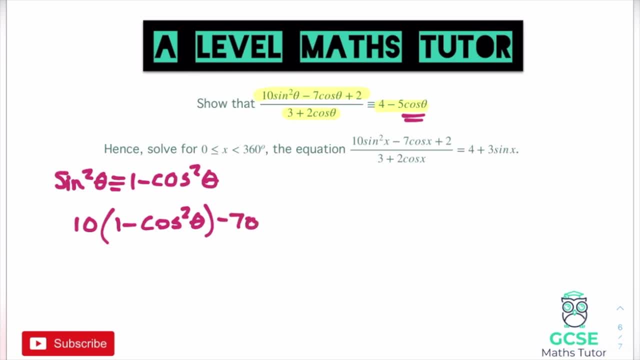 Minus 7 cos theta, plus 2, and that's all over 3 plus 2 cos theta. But we'll just go about simplifying the numerator to start with. 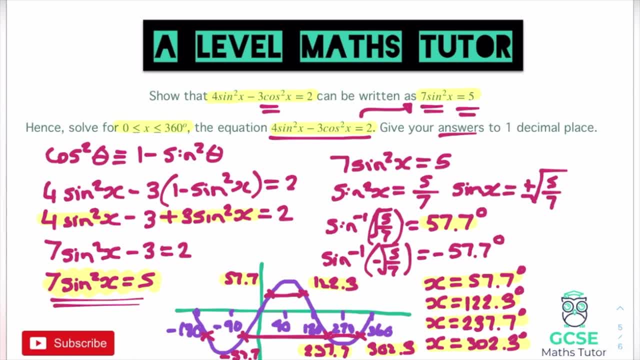 was equal to a number, so that we could actually find that amount in degrees and relate it to the trigonometric graph. So that's one type of question And obviously you can have harder ones than this And we're going to have a look at some harder ones as well. 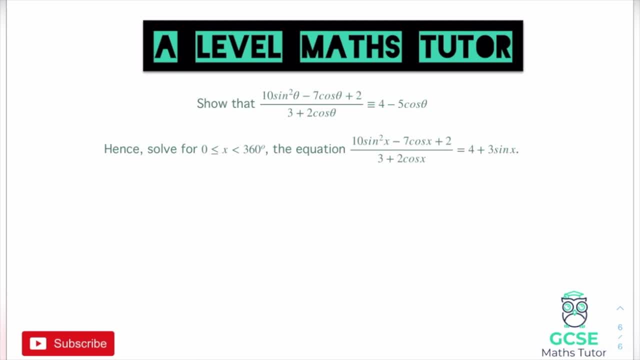 Okay. so looking at one of our harder trigonometric equations, you can see that obviously it doesn't look very nice. It says: show that 10 sine squared theta minus seven, cos squared theta plus two over three plus two, cos theta is always identical to. 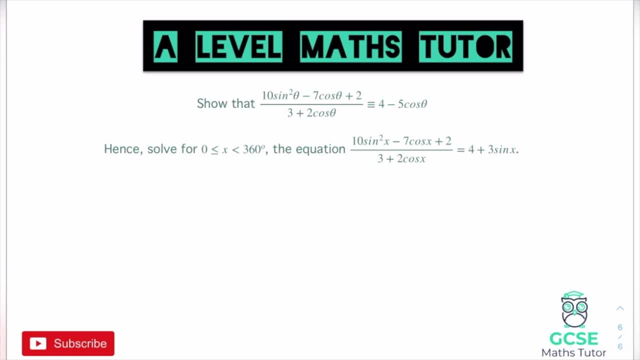 or equal to four minus four cos theta. Then it asks us: hence solve, and we've got a very similar question to what we've looked at before. But we're going to start with this first part and show that all of this comes out as four minus cos theta. 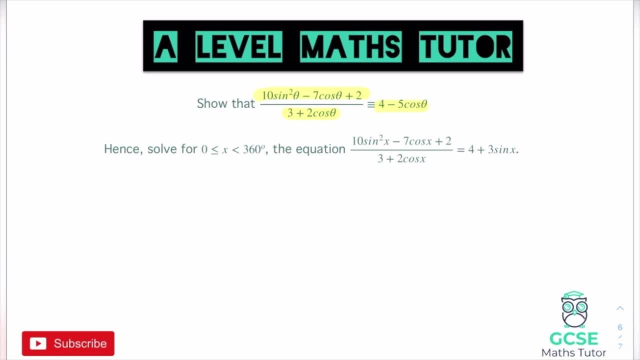 Now straight away, you can see that in our answer part there that we're looking to show that it's identical to, it has a cos in. So for all of the pieces that have a sine in or a sine squared theta in, we're going to want to turn that into a cos. 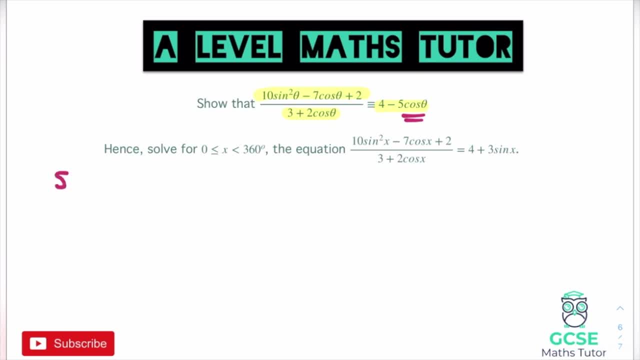 So straight away we'll write down our identity for that, and that is that sine squared theta is identical to one minus cos squared theta, And we'll plug that in and see where we get to. So if we start by replacing the sine squared theta, 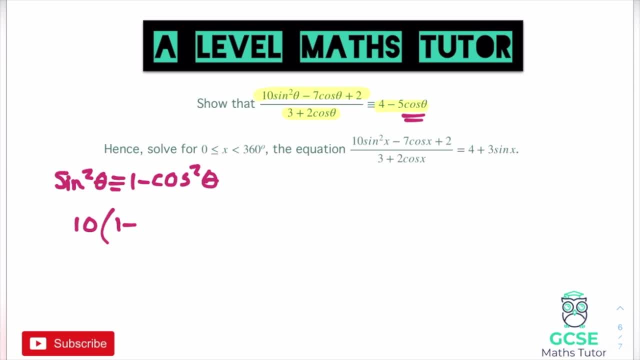 we have 10 lots of one minus cos squared theta minus seven cos theta plus two and that's all over three plus two cos theta. But we'll just go about simplifying the numerator to start with. So the next step for the numerator would be to expand that. 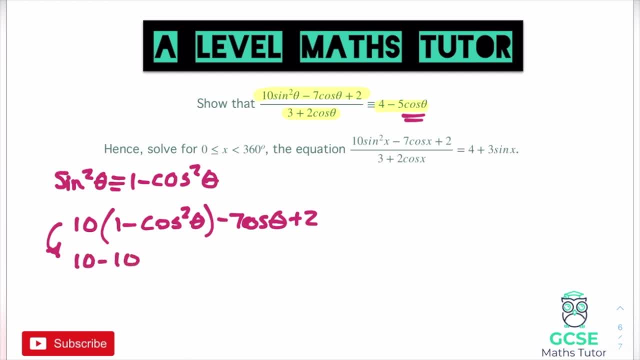 bracket. so we would have 10 minus 10 cos squared theta, and that is then minus seven cos theta plus two. So that's our next step, and now we're just going to think about whether we can simplify this. Now, the only thing we can really do to simplify this: 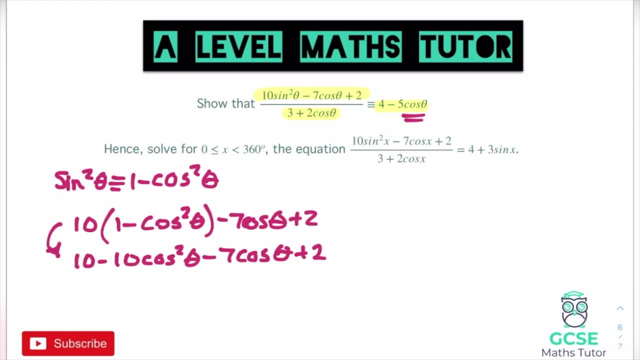 is obviously to add the 10 and the two together. So we'll add those two together, as they are our only like pieces on the top, and that would leave us with 12 minus 10 cos squared? theta minus seven, cos theta. Okay, there we go. 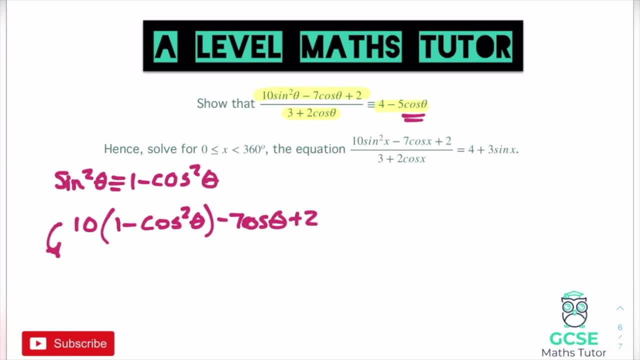 So the next step for the numerator would be to expand that bracket. So we would have 10 minus 10 cos squared theta, and that is then minus 7 cos theta, plus 2. So that's our next step, and now we're just going to think about whether we can simplify this. Now the only thing we can really do to simplify this is obviously to add the 10 and the 2 together. So we'll add those two together as they are our only like pieces on the top, and that would leave us with 12 minus 10 cos squared theta, minus 7 cos theta. Okay, there we go. 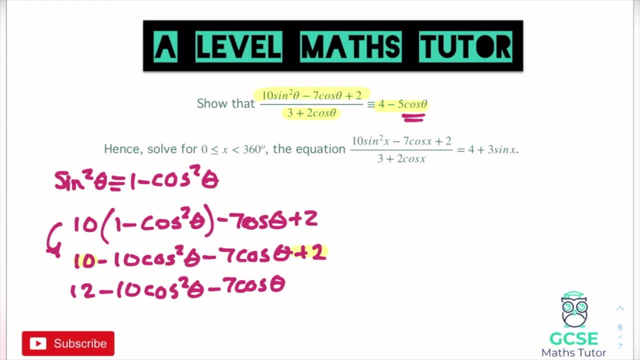 So at this point we need to think about whether this factor, this is just like a trigonometric quadratic. 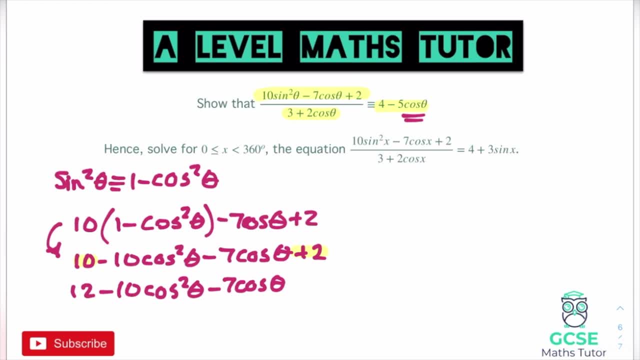 If we think back to obviously looking at quadratics, we could rewrite this in terms of x. 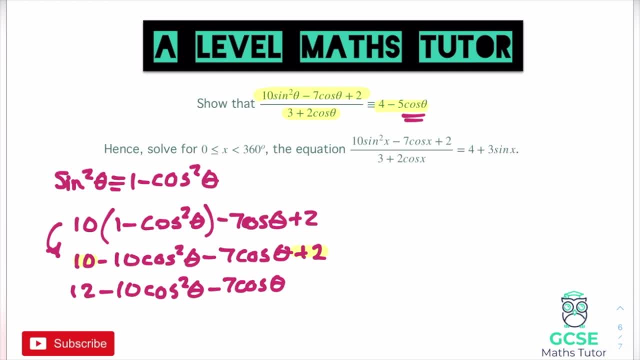 So rather than writing cos, I'm just going to replace that with the letter x and rewrite this as a quadratic. 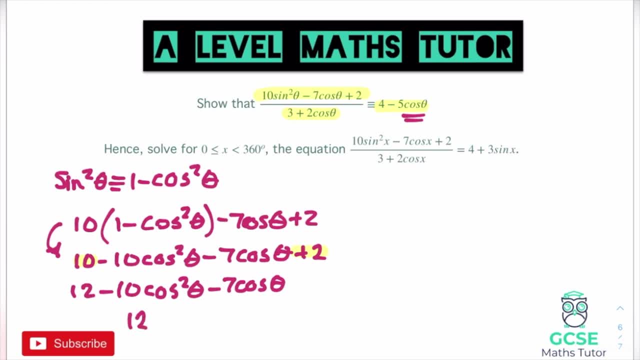 So if I was to rewrite that, it would look like this. It would look like 12 minus 10, and that's cos squared. So I would have 10 x squared minus 7 x. And I probably want to rearrange that so it looks like a normal negative quadratic, which is 12 minus, and then put the 7 x, and then minus 10 x squared. 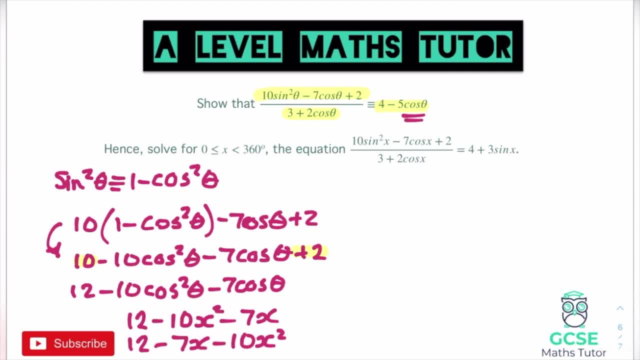 So this is going to really help if you are struggling to factorise trigonometrics when we have the quadratics and we're trying to actually factorise them. 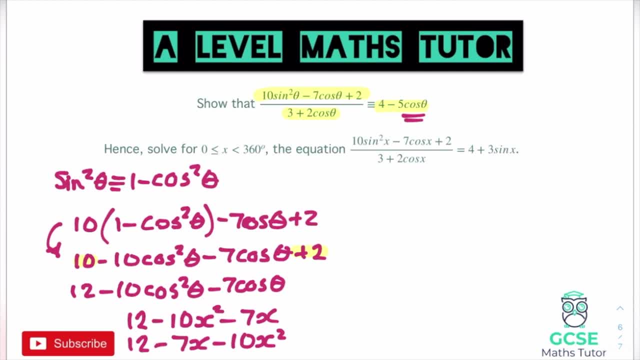 You can just write that, the cos or sin or whatever we're using in terms of x, and then look at it from there. 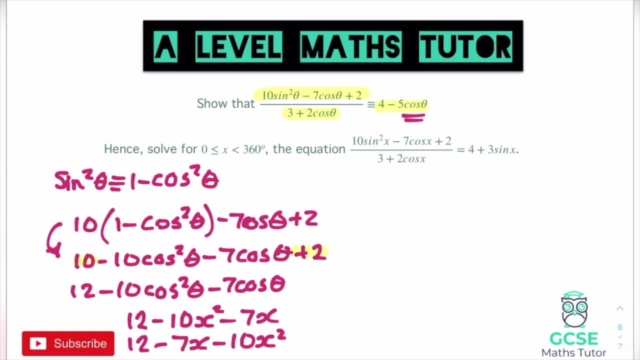 So if we go about factorising that, we want to think about those numbers that multiply to make 12, but of course we can actually change this quadratic, and, um, 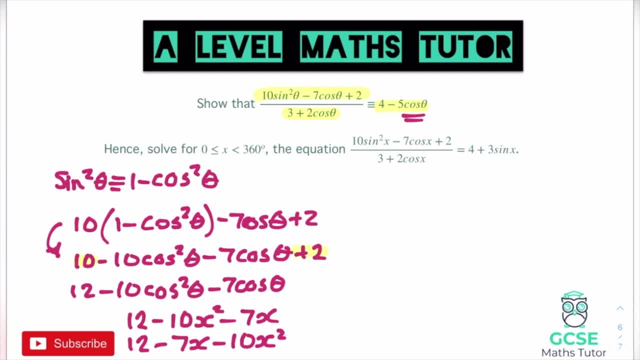 swap back our brackets at the end. So just to make it a little bit easier, I'm going to write it as positive 10 x squared plus 7 x minus 12, as this is really nice and quick to factorise. 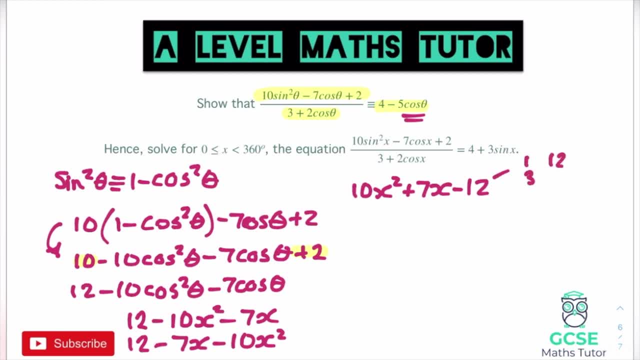 Our factors here would be 1 and 12, 3 and 4, or 2 and 6. 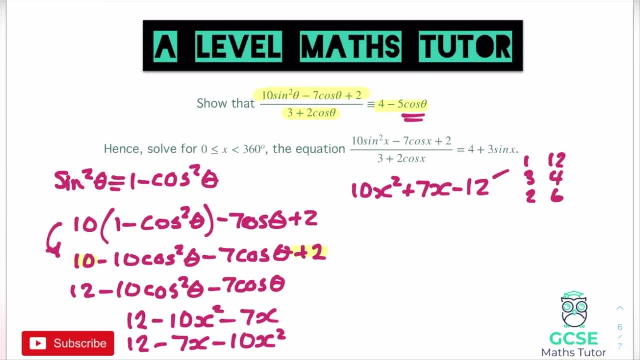 And you can obviously see that that is going to be, um, one of those numbers, but we need to think about our brackets. 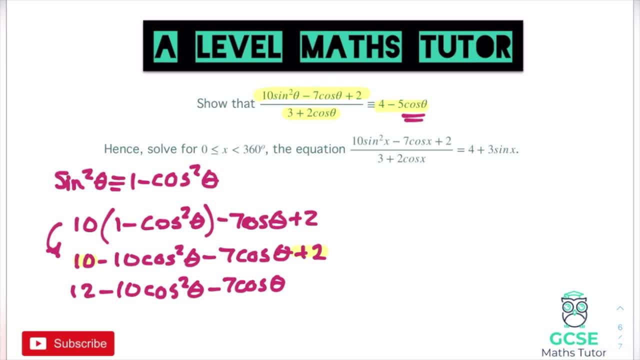 So at this point we need to think about whether this factorises. This is just like a trigonometric quadratic. if we think back to obviously looking at quadratics, we could rewrite this in terms of x. So rather than writing cos, I'm just going to replace. 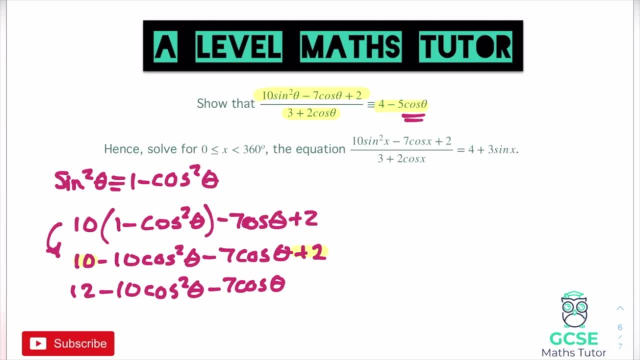 that with the letter x and rewrite this as a quadratic. So if I was to rewrite that, it would look like this: It would look like 12 minus 10 and that's cos squared. so I would have 10 x squared minus seven x. 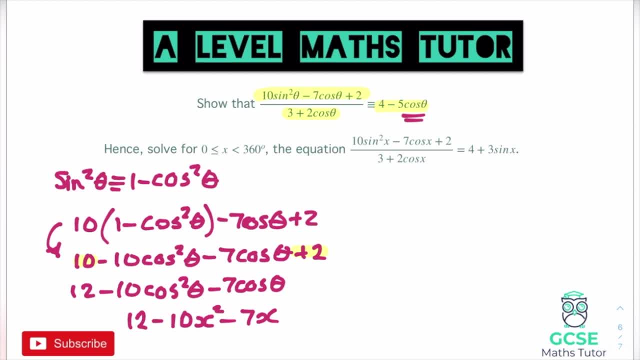 And I probably want to rearrange that so it looks like a normal negative quadratic which is 12 minus and then put the seven x and then minus 10 x squared. So this is going to really help if you are struggling to factorise trigonometrics when we have the quadratics. 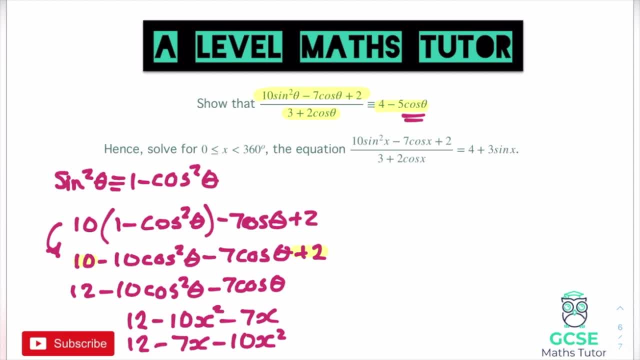 and we're trying to actually factorise them. You can just write the cos or sin or whatever we're using in terms of x and then look at it from there. So if we go about factorising that, we want to think about those numbers that multiply to make 12. 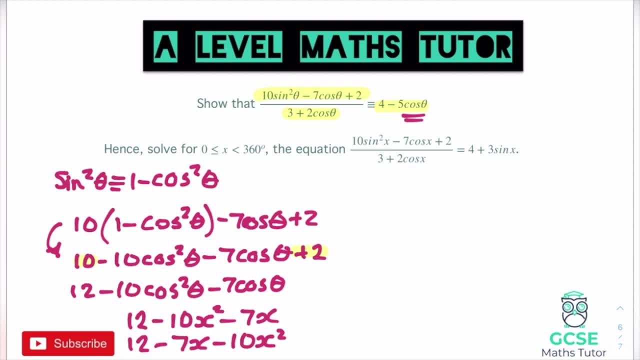 but of course we can actually change this quadratic and swap back our brackets at the end. So just to make it a little bit easier, I'm going to write it as positive: 10 x squared plus seven x minus 12, as this is really nice and quick to factorise. 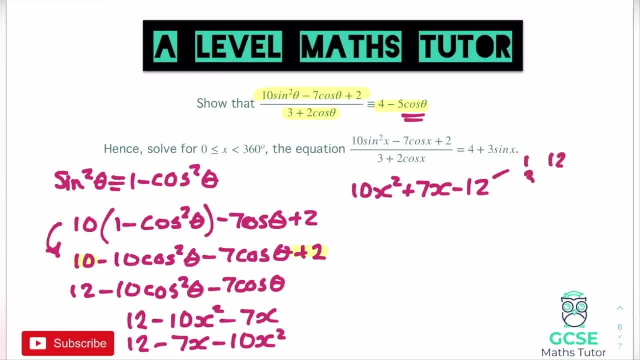 Our factors here would be one and 12,, three and four or two and six, and you can obviously see that that is going to be one of those numbers. but we need to think about our brackets Now. it's unlikely that it's going to be 10 and one. 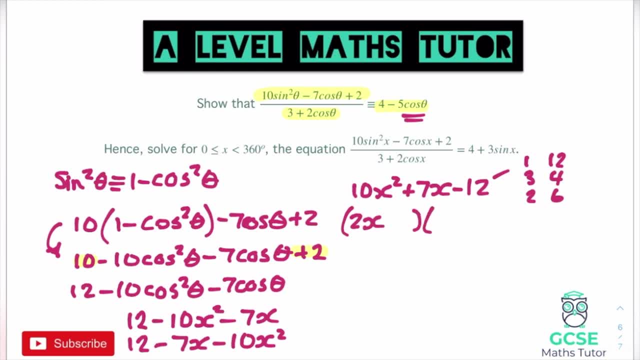 so we'll go with two x and five x and see if it factorises from there. Of course, if you don't want to factorise, you could type these into your calculator to get your solutions. but nice and easy for us to factorise. We have two times four, so it's going to be yeah. 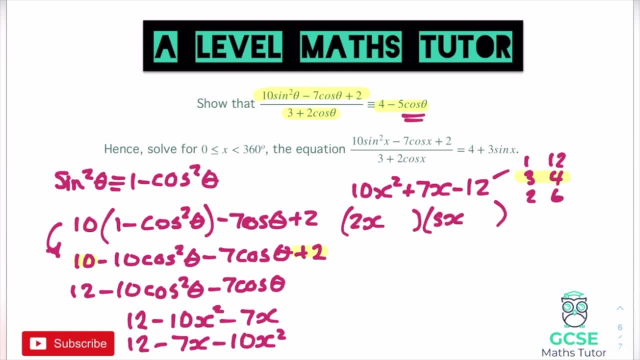 it's going to be that one there, three and four. again, take your time with this, but two times four would equal eight and three times three, sorry, three times five. on the other one would be 15 and 15 and eight. we can make seven with. 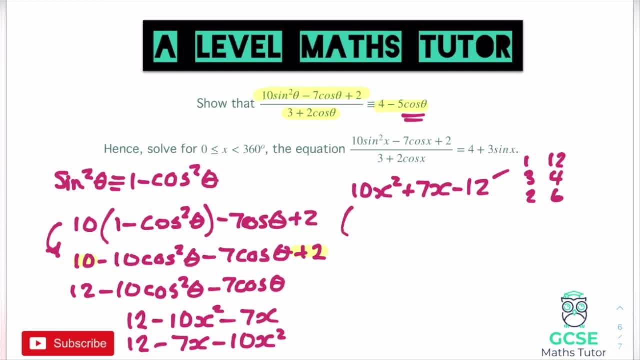 Now it's unlikely that it's going to be 10 and 1, so we'll go with 2x and 5x, and see if it factorises from there. 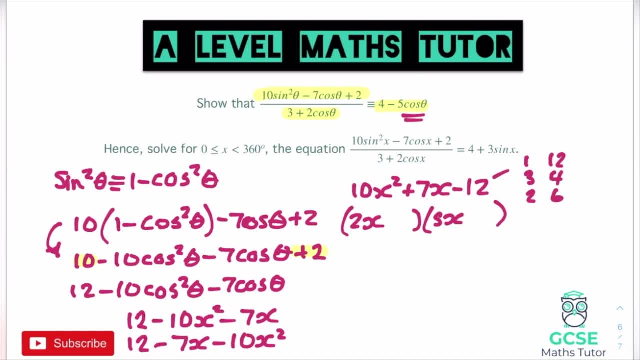 Of course, if you don't want to factorise, you could type these into your calculator to get your solutions, um, but nice and easy for us to factorise. 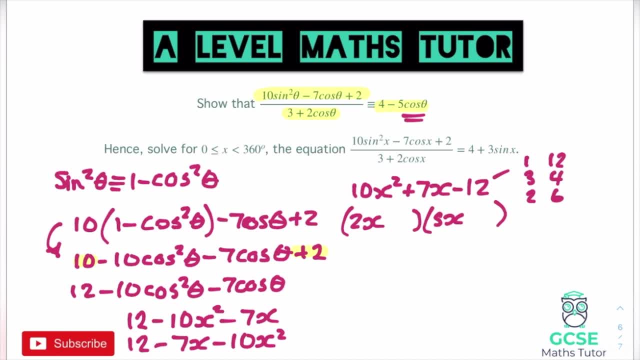 We have 2 times 4, so it's going to be, yeah, it's going to be that one there, 3 and 4, again take your time with this, but 2 times 4 would equal 8, and 3 times 3, um, sorry, 3 times 5 on the other one would be 15, and 15 and 8 we can make 7 with. We're going to make positive 7, so we'd want positive here and negative here, as that is going to make negative 8 plus 15, which makes plus 7. 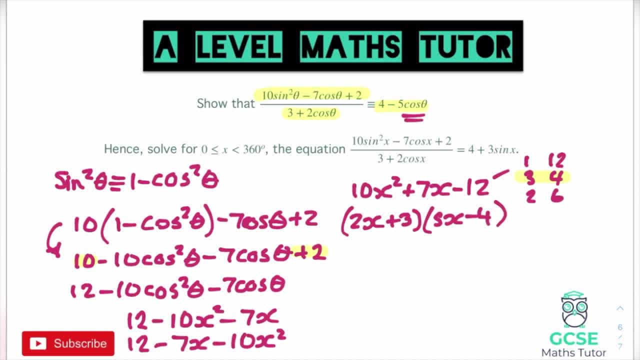 So we've managed to factorise it, all you have to do, because we swapped over the negative quadratic and made it positive, you just swap these brackets, or the pieces in the bracket over, so we would have, and it doesn't matter when there's a plus, but I'll swap it over anyway, 3 plus 2x, and over here we have 4 minus 5x. Okay, so there are our brackets done, but obviously these pieces, the x's, should have been a cos, so we just want to replace that, which would mean that our numerator now wouldn't have the x there, but would have the cos, so our numerator would be 3 plus 2 cos theta, and next to that, 4 minus 5 cos theta. There we go. 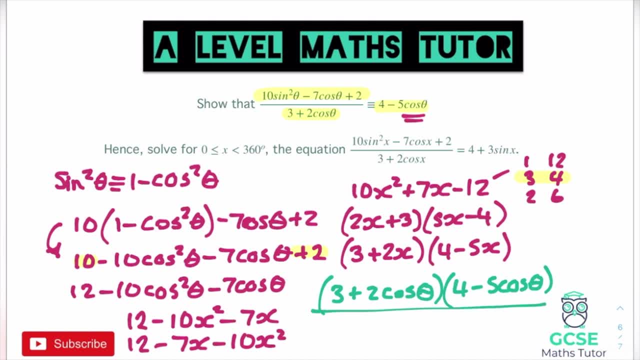 And our denominator, if we write that in as well, was 3 plus 2 cos theta. Now if you have a look, obviously looking at this fraction here, you can see that we have a matching factor on the top and the bottom, which is the 3 plus 2 cos theta. So they can both be cancelled out, which means all we are left with is the 4 minus 5 cos theta. So all of that would go down to 4 minus 5 cos theta, and as you can see, that matches what we're being asked to find in the question, where we're being asked to show that it was always equal to 4 minus 5 cos theta. 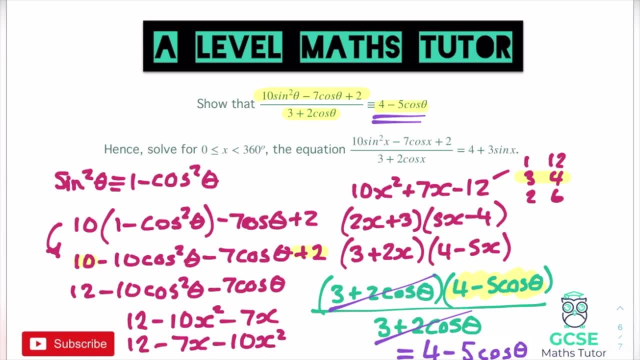 So we've managed to prove that for step 1. So this would be the first stage of this question. 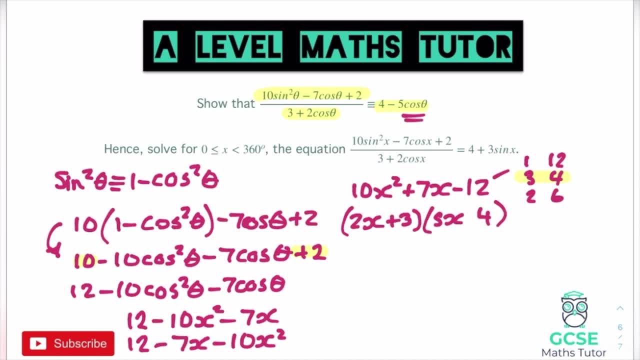 We're trying to make positive seven, so we'd want positive here and negative here, as that is going to make negative eight plus 15, which makes plus seven. So we've managed to factorise it. all you have to do, because we swapped over the negative quadratic. 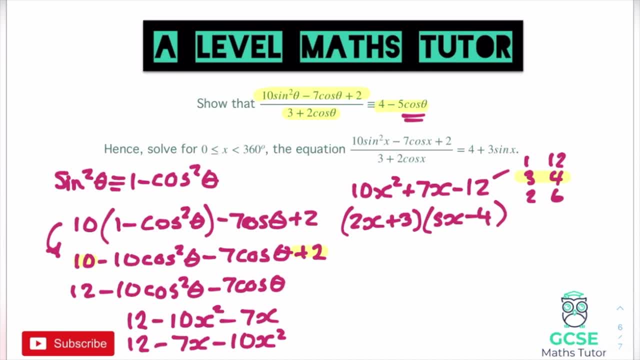 and made it positive. You just swap these brackets or the pieces in the bracket over. so we would have- and it doesn't matter when there's a plus, but I'll swap it over anyway- three plus two x, and over here we have four minus five x. 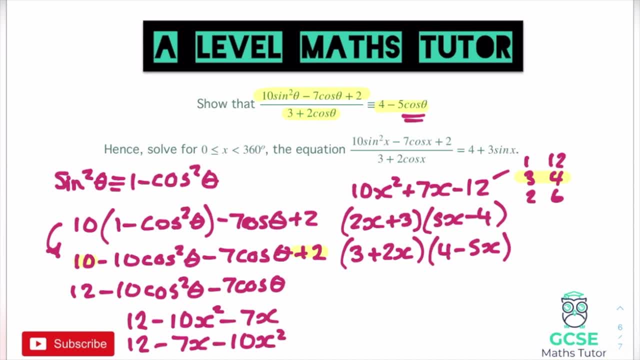 Okay, so there are our brackets done, but obviously these pieces, the x's, should have been a cos, so we just want to replace that, which would mean that our numerator now wouldn't have the x there but would have the cos. So our numerator would be three plus two, cos theta. 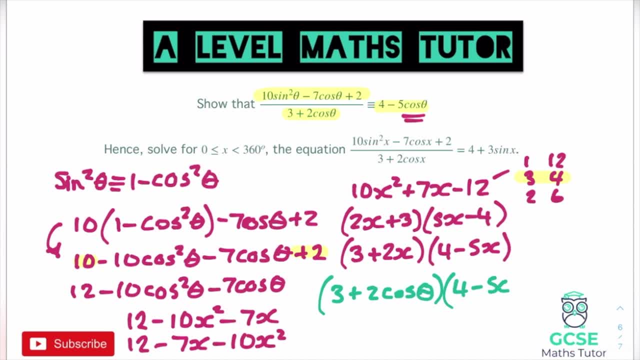 and next to that, four minus five cos theta. There we go, And our denominator, if we write that in as well- was three plus two cos theta. Now, if you have a look- obviously looking at this fraction here- you can see that we have a matching. 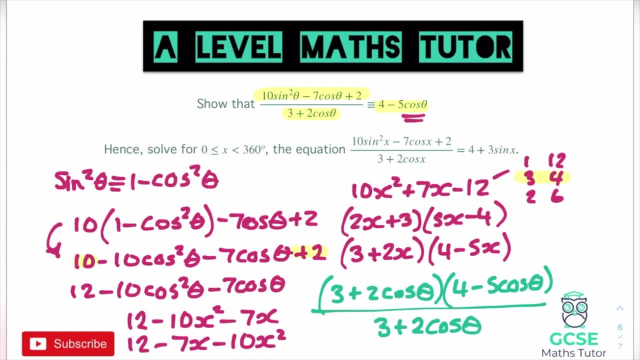 factor on the top and the bottom, which is the three plus two cos theta. So they can both be cancelled out, which means all we are left with is the four minus five cos theta. So all of that would go down to four minus five cos theta. 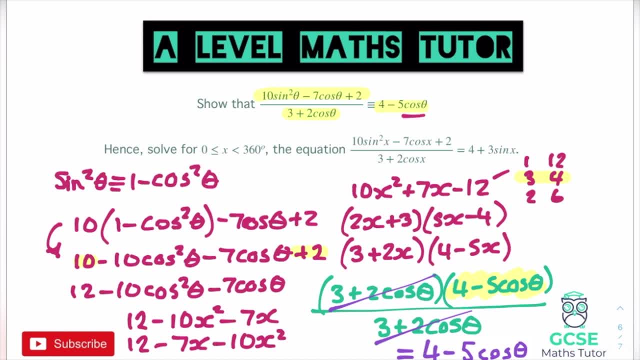 and, as you can see, that matches what we're being asked to find in the question, where we're being asked to show that it was always equal to four minus five cos theta. So we've managed to prove that for step one. So this would be the first stage of this question. 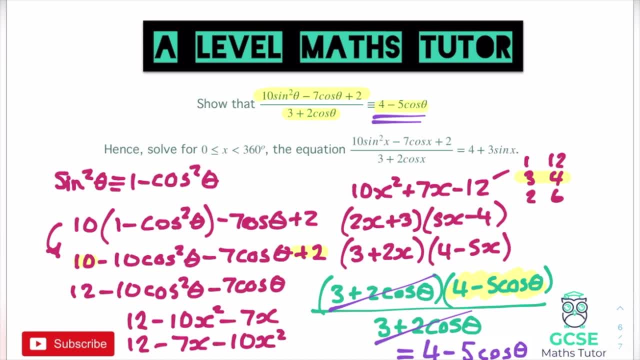 Obviously, you can see that I've run out of a lot of space here, so I am going to have to get rid of this working, but we're going to have a look now at the second part of the question, So we'll get rid of all this working. 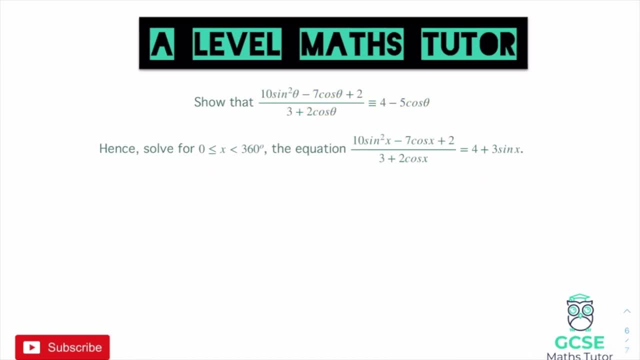 and we'll have a look at the second part. Okay, so for the second part of this question, it says: hence solve between nought and three hundred and sixty, including nought, but not three, sixty, the equation. and then it gives us the original equation. 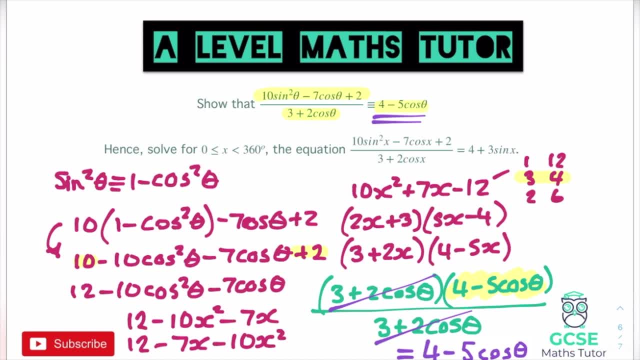 Obviously you can see that I've run out of a lot of space here, so I am going to have to get rid of this working, but we're going to have a look now at the second part of the question. 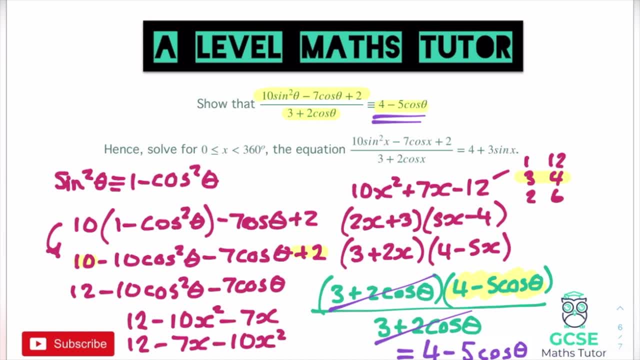 So we'll get rid of all this working, and we will have a look at the second part. 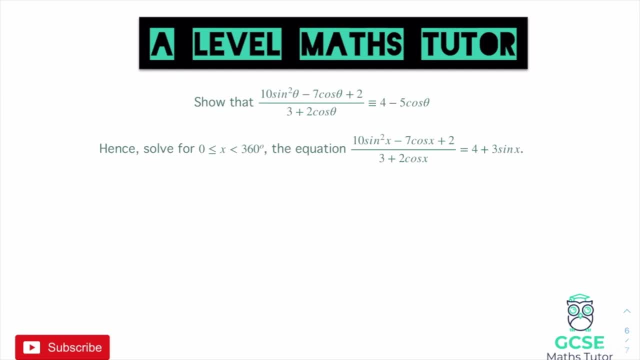 Okay, so for the second part of this question, it says, hence solve between 0 and 360, 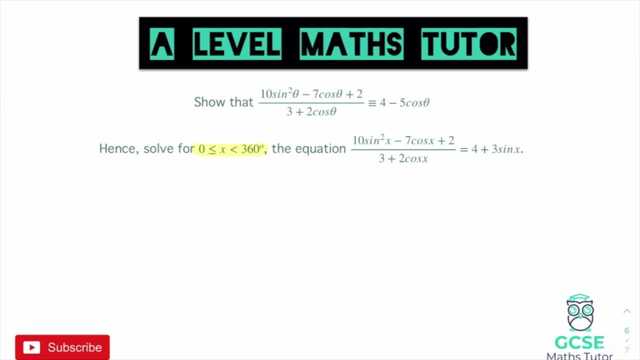 including 0 but not 360, the equation, and then it gives us the original equation, or the original pieces that we had there, but instead of putting theta, they've put x, but this time it doesn't say that it equals 4 minus 5 cos theta, it says that it is equal to 4 plus 3 sin x. 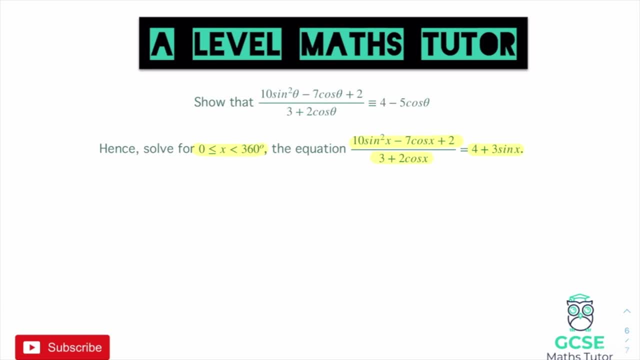 Now we already know from the first part that all of that is going to be equal to 4 minus cos theta, and if we were to write that using the letter x, that would just be 4 minus 5 cos theta. So we know that if both of them are equal to each other, that 4 minus 5 cos x is going to be equal to 4 plus 3 sin x, and that's going to be a little bit easier for us to use than that fraction, and again you're seeing in this question, we're using the piece from the start to help us with the second part here. 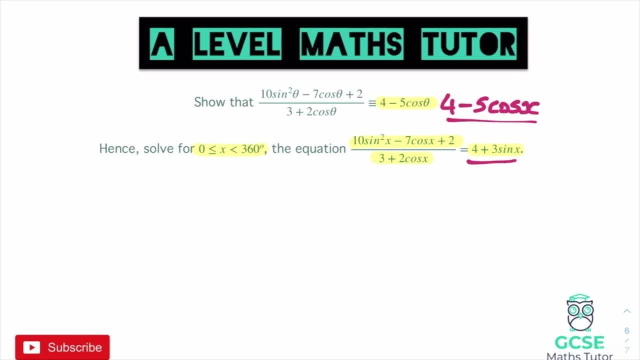 So the first thing we're going to want to do is set them equal to each other. So if we say that 4 plus, it doesn't matter which one we write first, let's just go for 4 plus 3 sin x, and that is going to be equal to 4 minus 5 cos x. Now again we want to obviously solve this, so we want to get this to a point where it only has sin cos or tan, and we'll think about how we could maybe get there. Now the first thing that you might notice here is there's a 4 on both sides, so we could minus 4 from both sides, and that would just leave us with 3 sin x, which is going to be equal to negative 5 cos x. 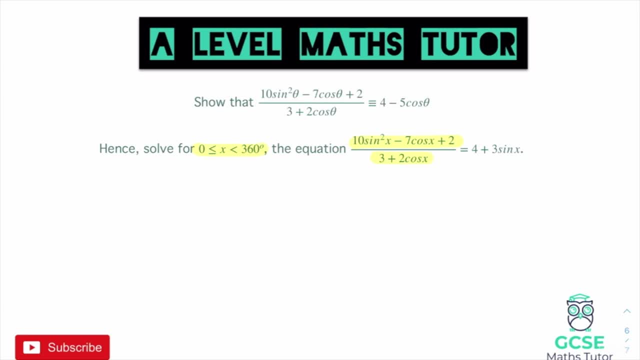 or the original pieces that we had there. but instead of putting theta, they've put x. but this time it doesn't say that it equals four minus five cos theta. It says that it is equal to four plus three sine x. Now we already know from the first part. 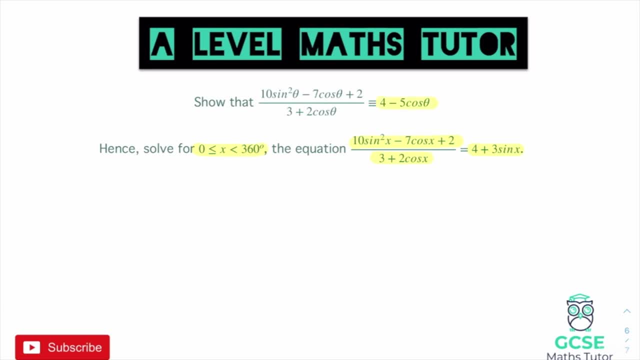 that all of that is going to be equal to four minus cos theta. and if we were to write that using the letter x, that would just be four minus five cos x. So we know that if both of them are equal to each one another, that four minus five cos x. 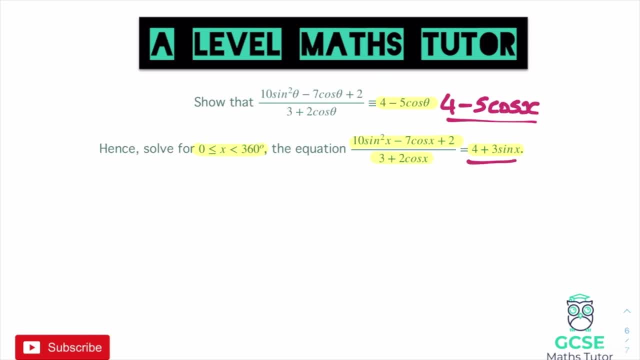 is going to be equal to four plus three sine x and that's going to be a little bit easier for us to use than that fraction. And again, you're seeing, in this question we're using the piece from the start to help us with the second part here. 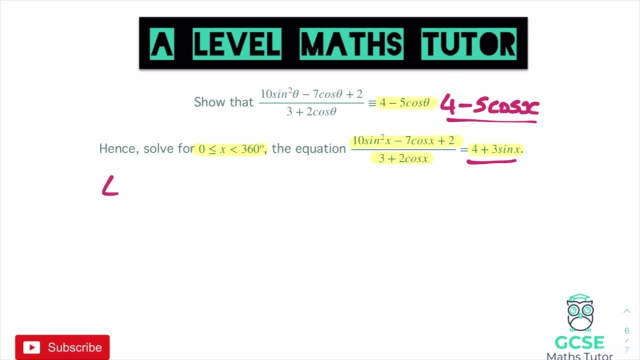 So the first thing we're going to want to do is set them equal to each other. So if we say that four plus, it doesn't matter which one we write first, let's just go for four plus three sine x, and that is going to be equal to four minus five cos x. 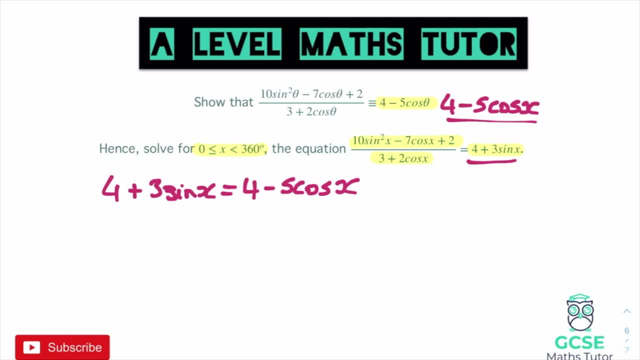 Now again, we want to obviously solve this. so we want to get this to a point where it only has sin, cos or tan, And we'll think about how we could maybe get there. Now, the first thing that you might notice here is there's a four on both sides. 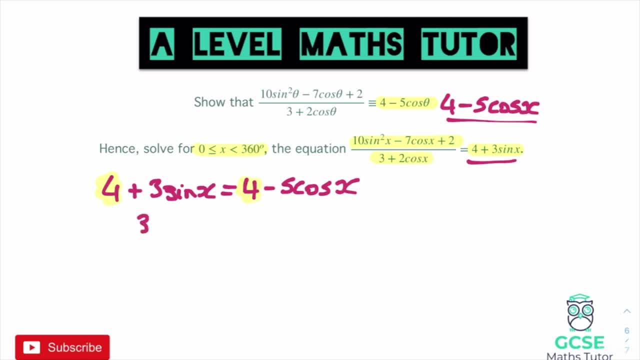 so we could minus four from both sides, and that would just leave us with three sine x, which is going to be equal to negative five cos x. So that would be our first step and that's gotten rid of a four from both sides. What we could now do to get it so it's just sine x. 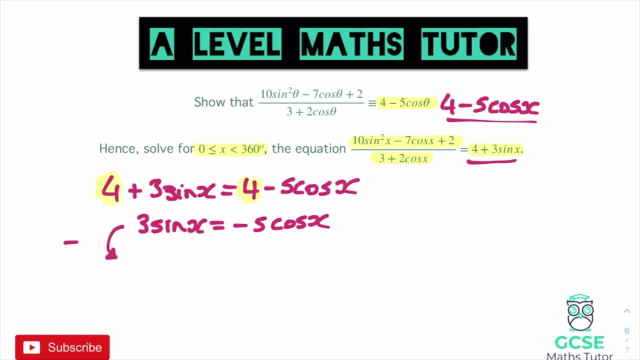 or just cos x, and I'm just going to divide both sides by three. That's going to remove the three from the start, And then we'll think about where we could go with next. So if we divide both sides by three, that leaves us with sine x equals. 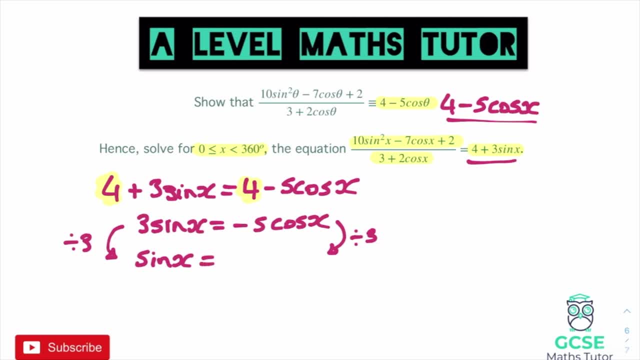 which is going to be helpful, is equal to- and I'll just divide the negative five by the three, so negative five thirds cos x. Now, at this point here you'd hopefully notice that one of our trig identities is going to get involved, and that is if we divide both sides by cos x. 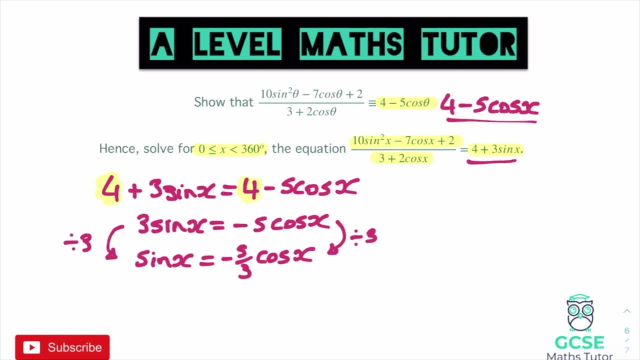 we're going to have sine x over cos x. Now we know from our trig identities identity that sine x divided by cos x is equal to tan x. So that is going to eliminate our two different trig pieces there, because now we're just going to have tan x. So if we do that, 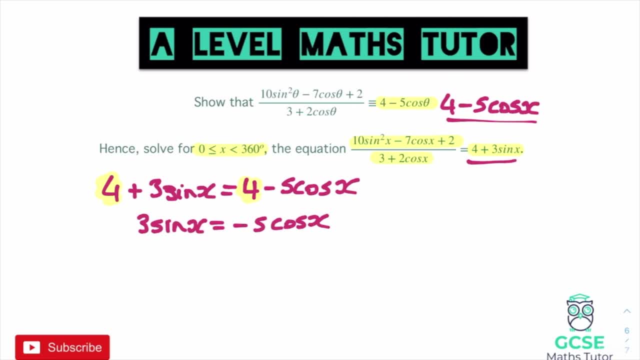 So that would be our first step, and that's gotten rid of a 4 from both sides. What we could now do to get it so it's just sin x or just cos x, and I'm just going to divide both sides by 3. That's going to remove the 3 from the start, and then we'll think about where we could go with next. So if we divide both sides by 3, that leaves us with sin x equals, which is going to be helpful, is equal to, and I'll just divide the negative 5 by the 3, so negative 5 cos x. 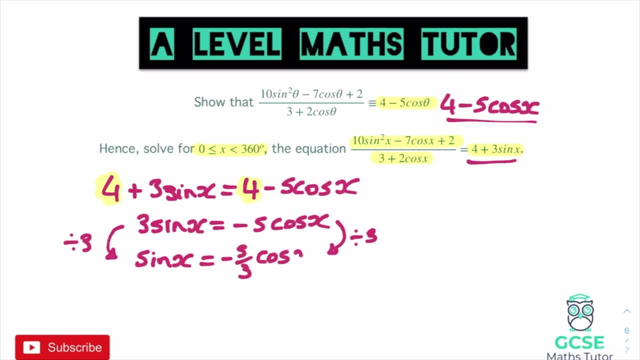 So that leaves us with 3 cos x. Now at this point here you'd hopefully notice that one of our trig identities is going to get involved, and that is if we divide both sides by cos x, we're going to have sin x over cos x. Now we know from our trig identity that sin x divided by cos x is equal to tan x. So that is going to eliminate our two different trig pieces there, because now we're just going to have tan x. 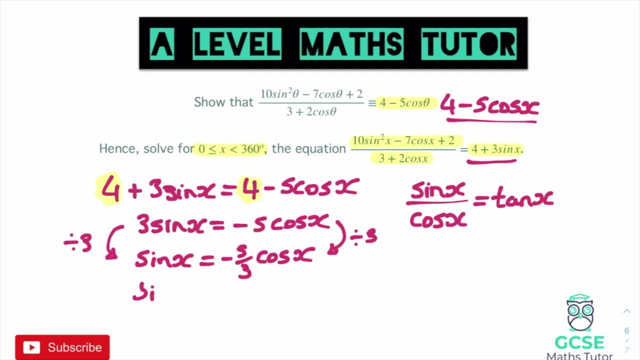 So if we do that, we would have sin x over tan x, and we divide by cos x, sorry, sin x over cos x, is going to equal negative 5 over 3. 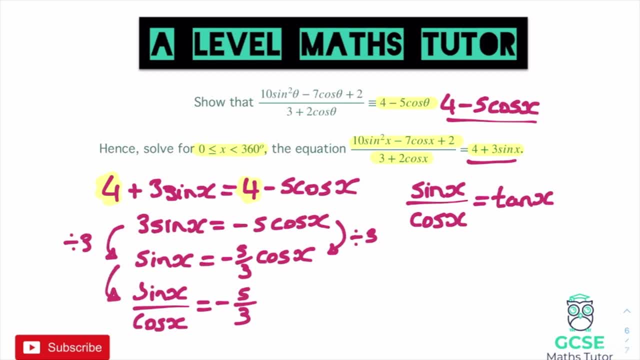 And again you could write in what you've done there, we've just divided by cos x. There we go. 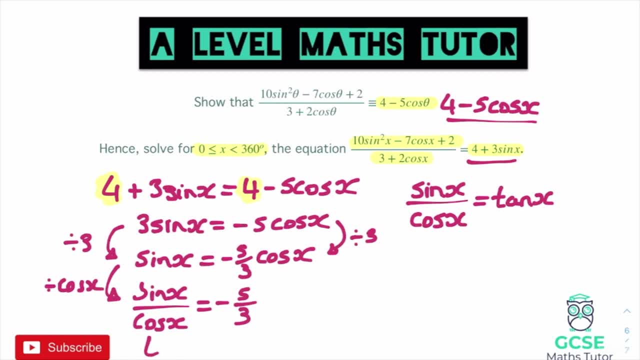 And of course sin x over cos x is equal to tan x, so we could just rewrite this that tan x is equal to minus 5 over 3. 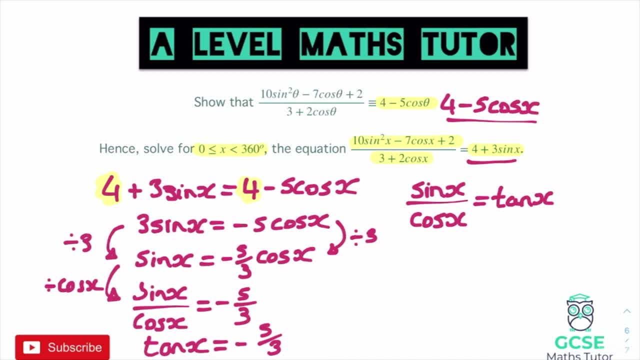 So that's going to be very important there, because now we're in a position where we can solve it. 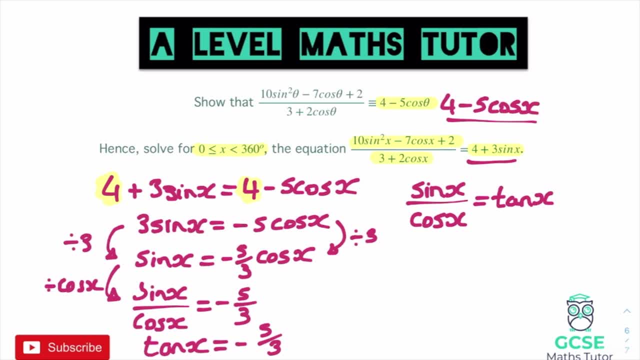 So at this point, we can do the inverse of tan, and get our solution. 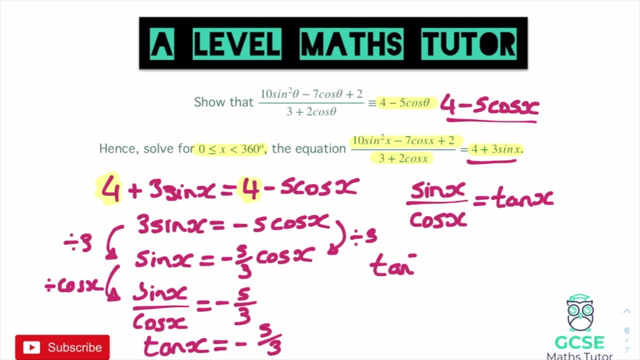 So for tan minus 1, so we get our angle, and that's tan minus 1 of negative 5 over 3. 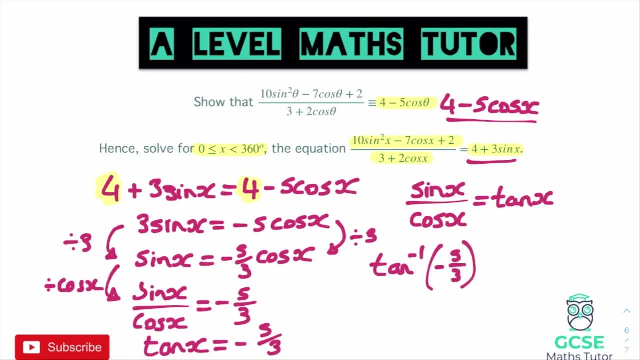 If we type that into our calculator, we get the answer, and it comes out as minus 59.0. 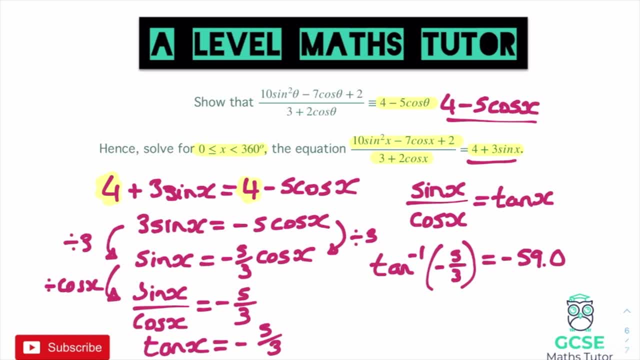 So we've got our first solution. Now of course that has fallen outside of our range that we were looking at, 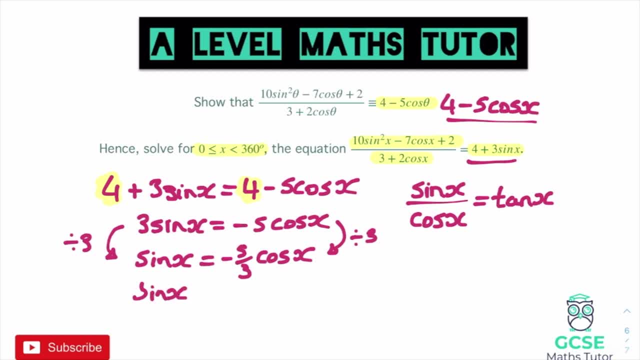 we would have sine x over tan x when we divide by cos x. sorry, sine x over cos x is going to equal negative 5 over 3.. And again you could write in what you've done there. we've just divided by cos x. There we go, And of course sine x over cos x is equal to tan x. So 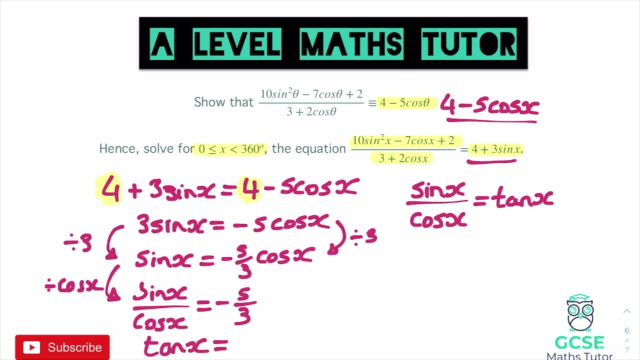 we could just rewrite this: that tan x is equal to minus 5 over 3.. So that's going to be very important there, because now we're in a position where we can solve it. So at this point we can do the inverse of tan and get our solution. So for tan minus 1, so we get our angle and that's tan. 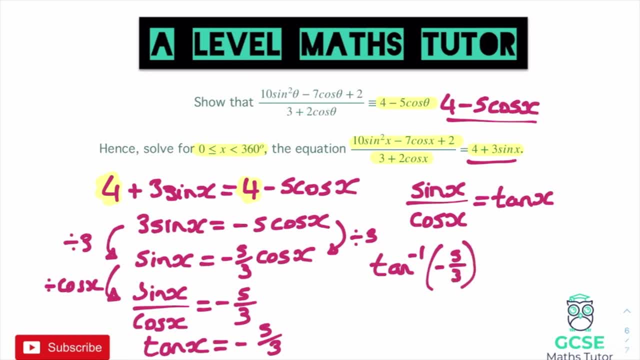 minus 1 of negative 5 over 3, if we type that into our calculator, we get the answer and it comes out as minus 59.0.. So we've got our first solution. Now, of course, that has fallen outside of our range that we were. 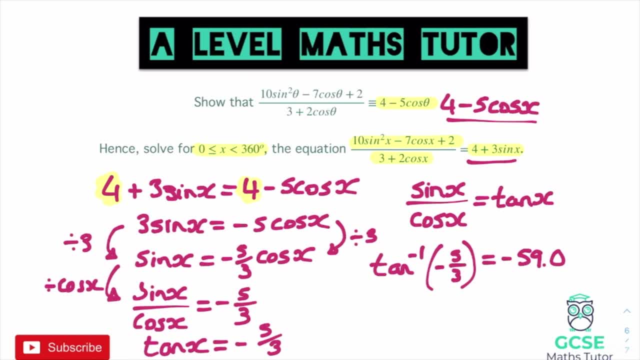 looking at, as we're only looking between 0 and 360.. So for this we are going to have to draw our tan graph and we're going to have to visualize where those solutions are. So if we get rid of some of this working and we're going to have to visualize where those solutions are. So if we get 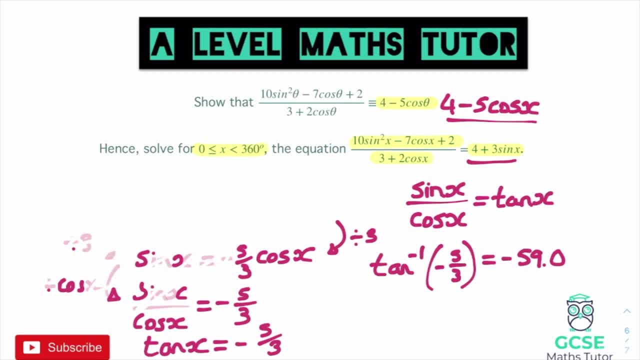 rid of some of this. we can just draw the graph over here and that's going to help us just to visualize that. So here we go, Let's just get rid of all of this. Lots of pieces there, But we want to draw this tan graph. I'm going to draw a nice sketch of that. So if we draw some axes again, 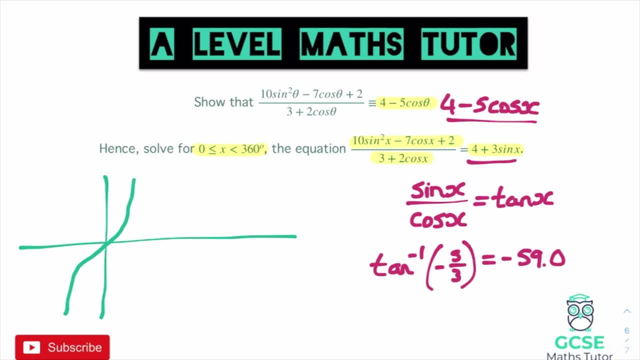 our first wave goes through the origin, and then we have our asymptote at 90, and our next one goes up, then through the 180, and our next asymptote is at 200.. So we've got our tan graph and we've got 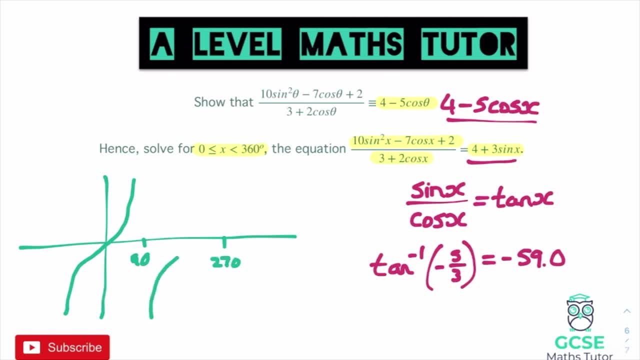 our tan graph at 270.. So that's going to go up through the center there And I've drawn that very badly, so we should probably draw that again. Again, it is just a sketch, just to help you to visualize it, but it's good to draw it quite well. And our next one would start at 270, and it goes. 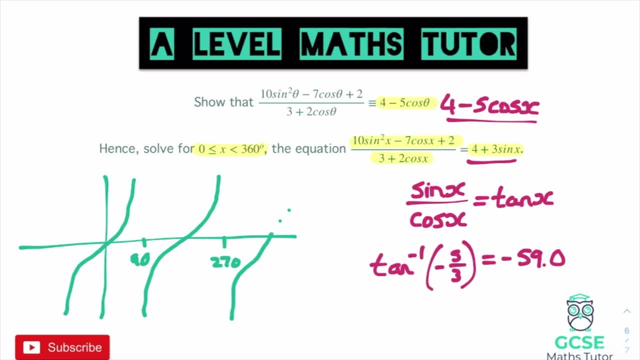 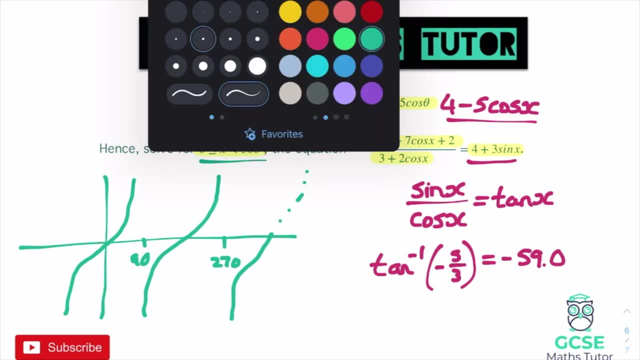 up through 360.. So we could stop there, but of course that does actually carry on, but we don't need to draw the rest in because we're only going up to 360.. So let's think about where that solution would lie. We've got negative 59.0. 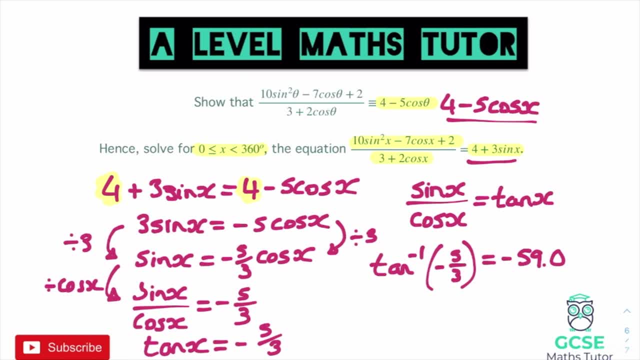 as we're only looking between 0 and 360. So for this we are going to have to draw our tan graph, and we're going to have to visualise where those solutions are. 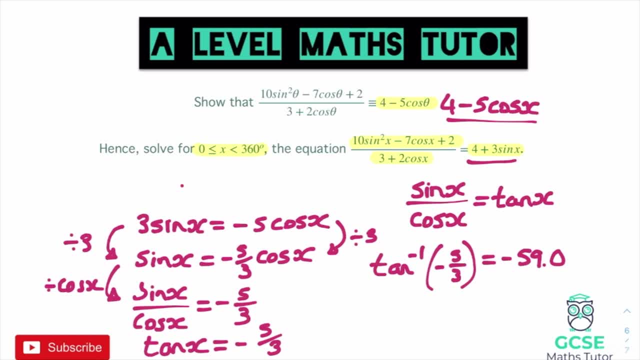 So if we get rid of some of this working, and we can just draw the graph over here, and that's going to help us just to visualise that. 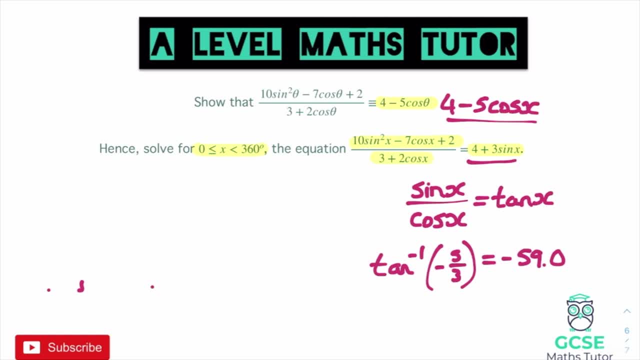 So here we go, let's just get rid of all of this, lots of pieces there. 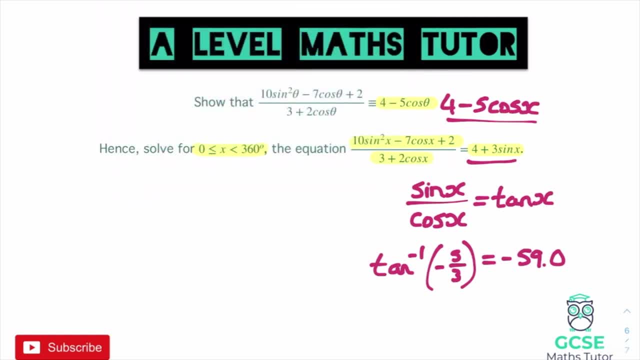 But we want to draw this tan graph, and we want to draw a nice sketch of that. So if we draw some axes, 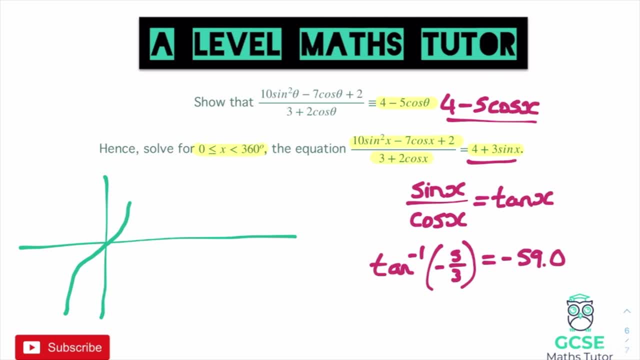 again our first wave goes through the origin, and then we have our asymptote at 90, and our next one goes up then, through the 180, and our next asymptote is at 270. 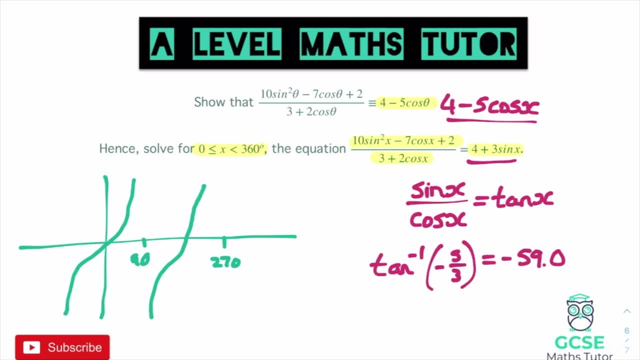 So that's going to go up through the centre there, and I've drawn that very badly, so we should probably draw that again. Again it is just a sketch, just to help you to visualise it, but it's good to draw it quite well. 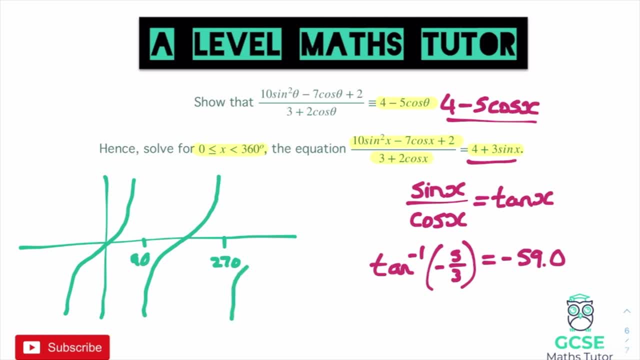 And our next one would start at 270, and it goes up through 360, so we could stop there, but of course that does actually carry on, but we don't need to draw the rest in, because we're only going up to 360. 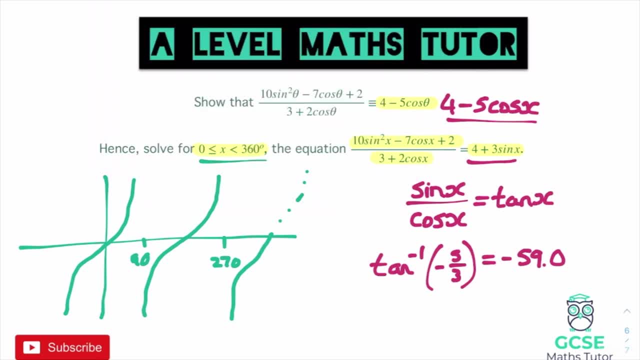 So let's think about where that solution would lie, we've got negative 59.0, and that would go between 0 and the negative 90, where our other asymptote is. So it's going to be somewhere in the middle, let's just imagine it falls just there, if we were to trace that down, and then of course all we're going to do, is we're going to go across, so we would go across, we'll hit the next curve just here, and then we're going to go across again, and we'll hit the next curve just there. 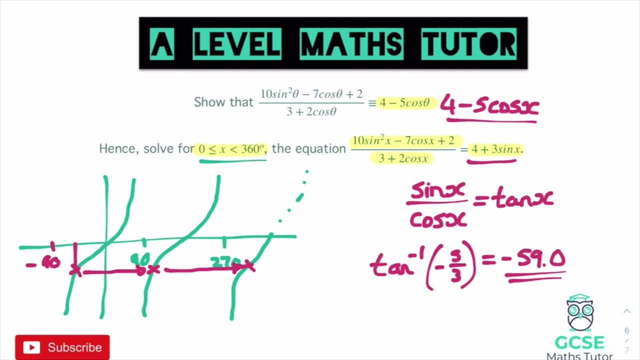 Again you might know some quick ways of jumping between these tan values, and again if you use any of your quadrants and things like that, that's absolutely fine, but again as I've explained before, 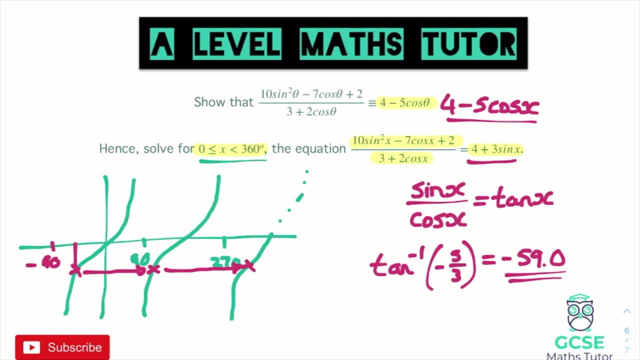 I do like to visualise what these graphs look like, just to imagine where they're going to go. 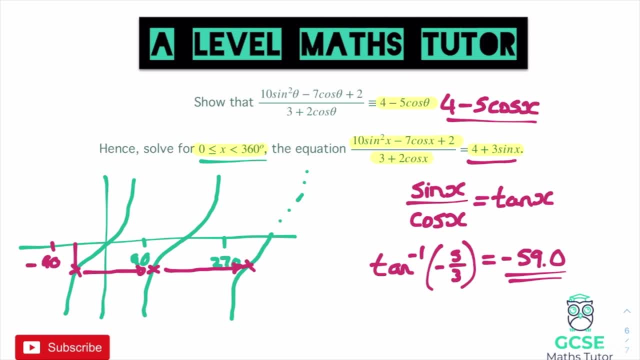 So for the first one, to jump between these two, it is just a jump of 180 degrees. 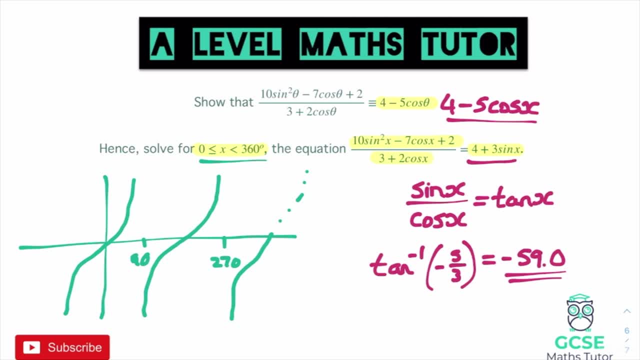 And that would go between 0 and the negative 90, where our other asymptote is. So it's going to be somewhere in the middle. Let's just imagine it falls just there if we were to trace that down, And then of course all we're going to do is go across. So we would go across, We'll hit the next. 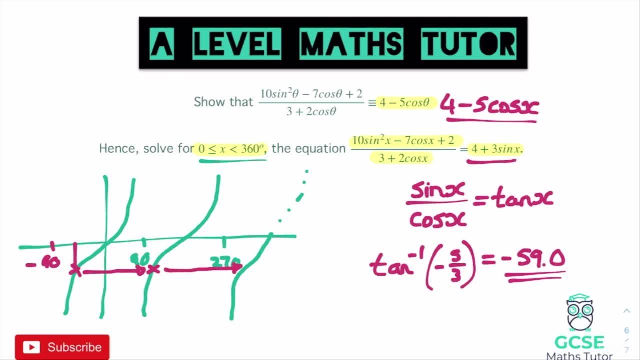 curve just here And then we're going to go across again and we'll hit the next curve just there. Again, you might know some quick ways of jumping between these tan values. And again, if you use any of your quadrants and things like that, that's absolutely fine. 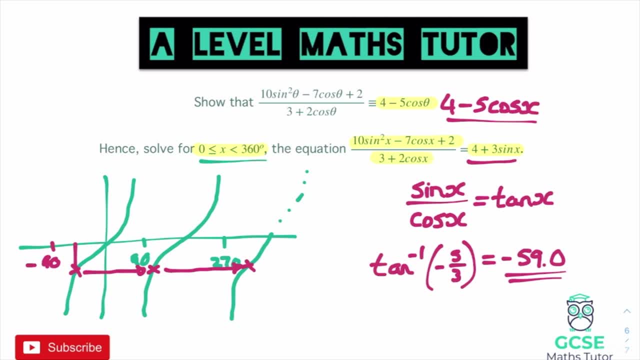 But again, as I've explained before, I do like to visualize what these graphs look like, just to imagine where they're going to go. So for the first one to jump between these two, it is just a jump of 180 degrees. So if this one here is negative 59, let me just check it on the calculator, because 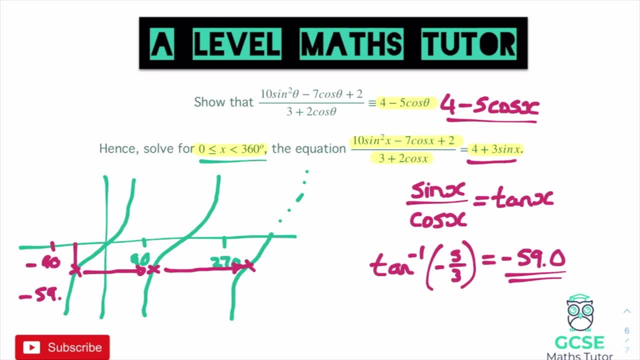 it doesn't say in this question how to round it. It did come out as negative 59.04, so I'm going to give it to two decimal places just to make it a little bit more accurate. So negative 59.04, to jump. 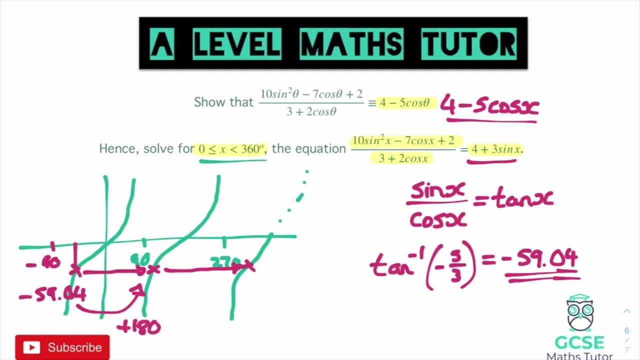 to the next one, I'm going to add 180.. So if we add 180 to that, it comes out as 120.96.. It comes out as: and there we go. So, jumping on to the next one, I would go another 180, so plus 180 again. 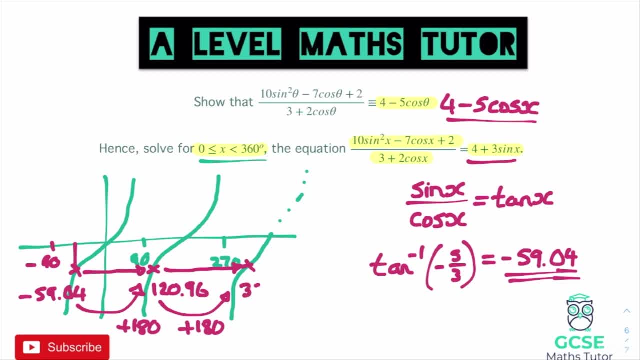 And that comes out as on the calculator that comes out as 300.96.. And of course, if we jump to 180 again it would go over our limit. So if we jump to 180 again it would go over our limit. 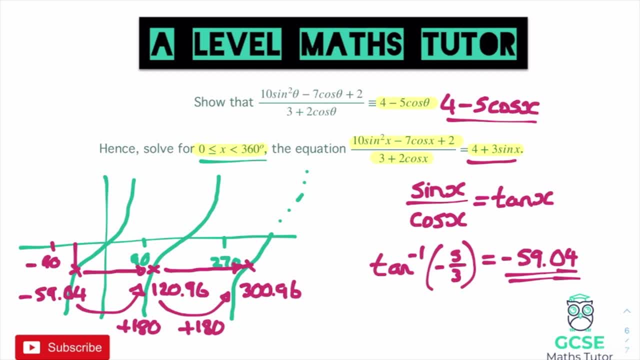 Which is 360 degrees. So these three, these solutions, here we've got three solutions: negative 59.04,, which is below zero, So we can't have that one, but we do have 120.96, and also 300.96.. So we do have two solutions there. Again, we would round that as we see. 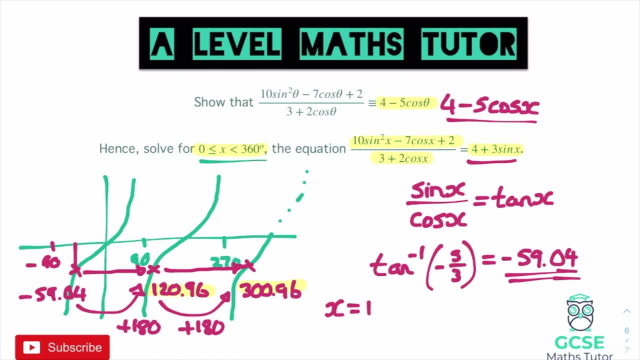 appropriate. So we could say that x is equal to 120.96.. Of course we could write that is equal to 120.96.. So we could write: that is equal to 120.96.. So we could write: that is equal to 120.96.. 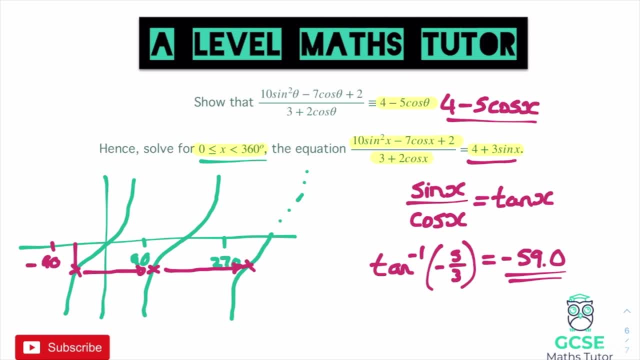 So if this one here is negative 59, and let me just check it on the calculator, because it doesn't say in this question how to round it, it did come out as negative 59.04, so I'm going to give it to two decimal places, just to make it a little bit more accurate, so negative 59.04, to jump to the next one there, all I need to do is add 180. 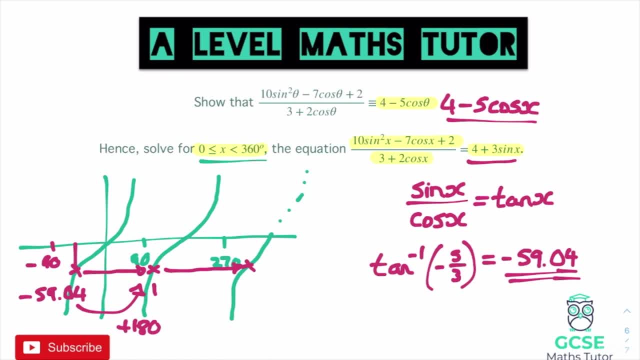 So if we add 180 to that, it comes out as 120 point, 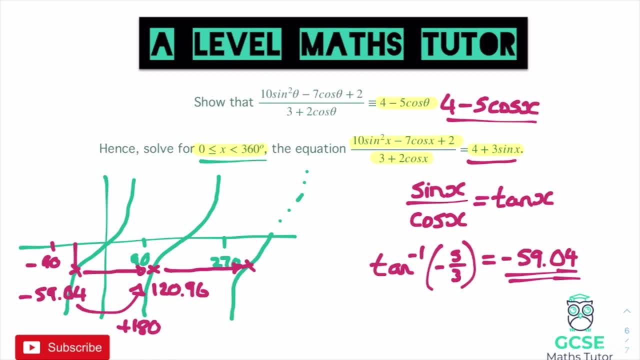 and then 96 it comes out as, and there we go, 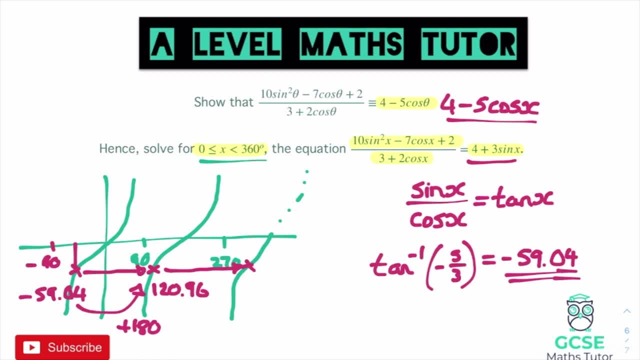 so jumping onto the next one, I would go another 180, so plus 180 again, and that comes out as, on the calculator, that comes out as 300 point 96, 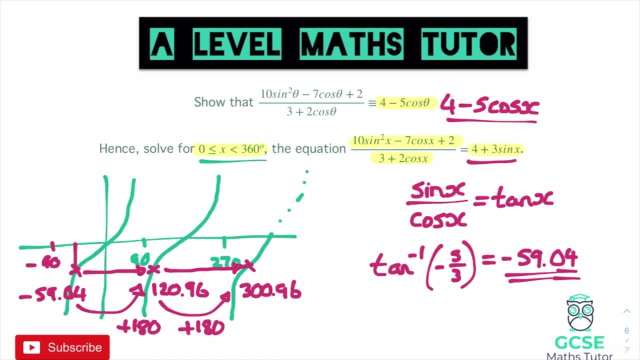 and of course if we jump to 180 again, it would go over our limit, which is 360 degrees. 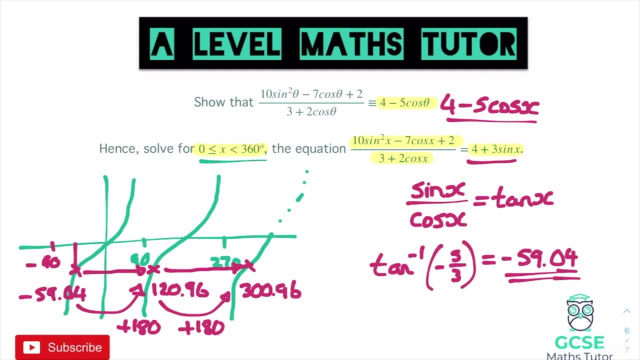 So these solutions here, we've got three solutions, negative 59.04, which is below zero, so we can't have that one, but we do have 120 points, 0.96, and also 300 point 96. So we do have two solutions there, again we would round that as we see appropriate, so we could say that x is equal to 120 point 96, of course we could write that is equal to, or we could say 121 degrees, to the nearest degree, and we also have x is equal to 300 point 96, 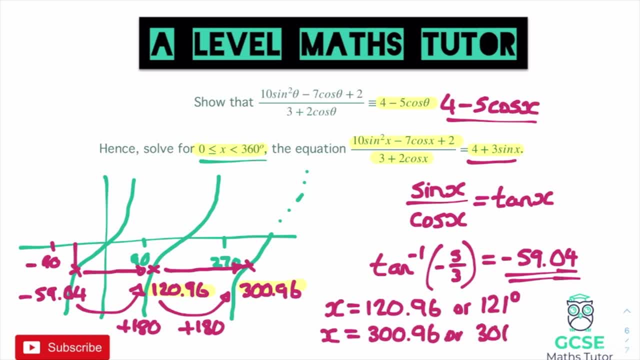 or we could write that that is equal to 301 degrees, again just being to the nearest degree there. 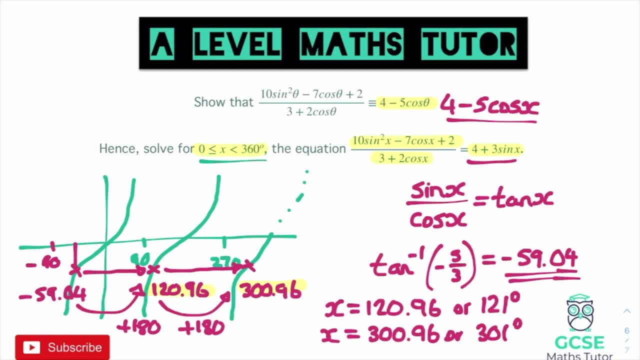 So obviously you can see this one is pretty tough, there was quite a lot of steps, 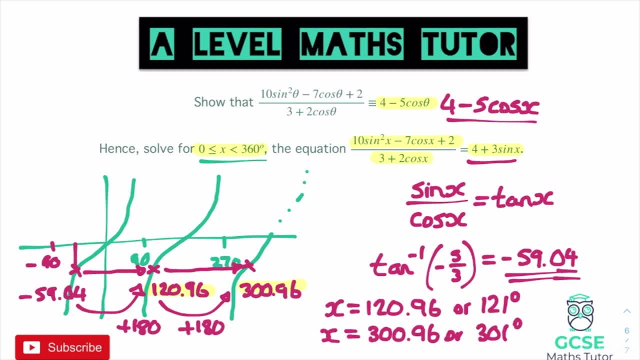 but you can see a lot of similarity between these trigonometric equations, whereby we are isolating it down to either sin cos or tan, we're doing the inverse to find the angle, and then we're just sketching it onto the graph, so we can see how many solutions we've got. 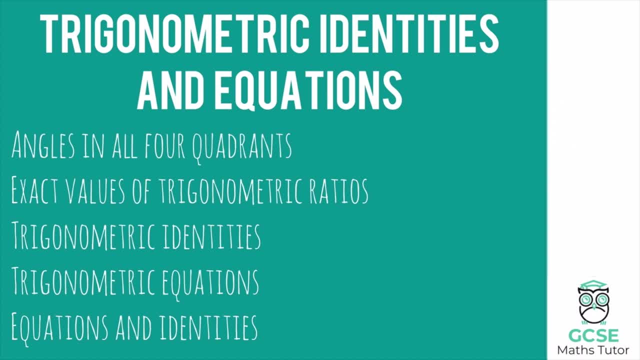 Okay, well done, that is the end of the video, I hope you enjoyed that, if you did, please don't forget to like, don't forget to comment, and don't forget to subscribe, and I'll see you for the next chapter.